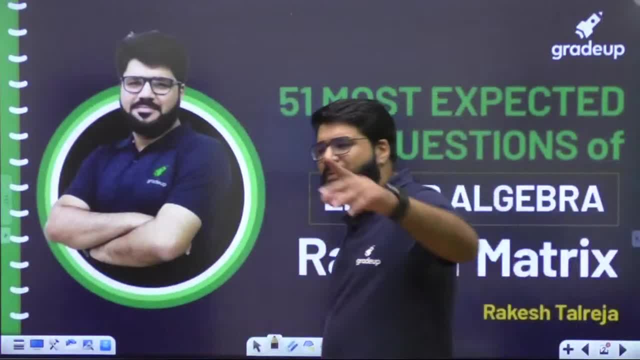 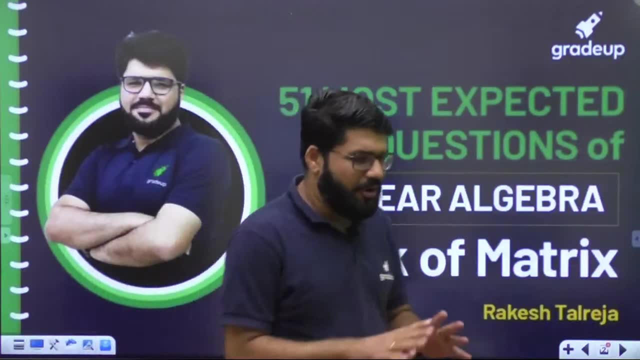 thought, you know, usually we are keeping up, usually we are keeping up at 10 pm, but this time I thought let's keep it late night. okay, let's see, you know you look all guys just free from all of your dinner, all of your day activities. 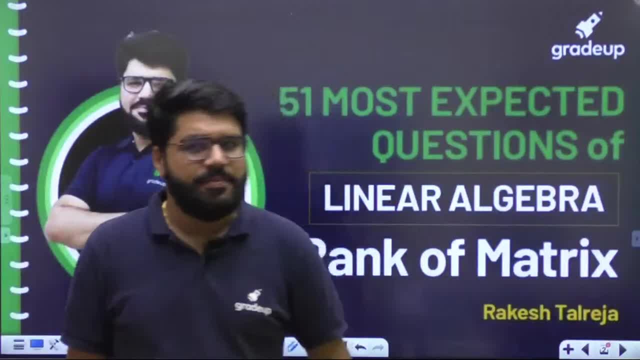 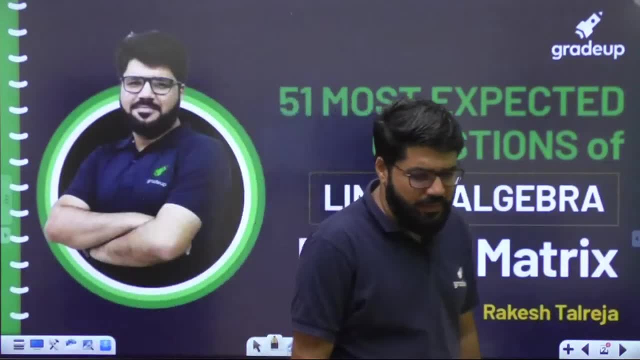 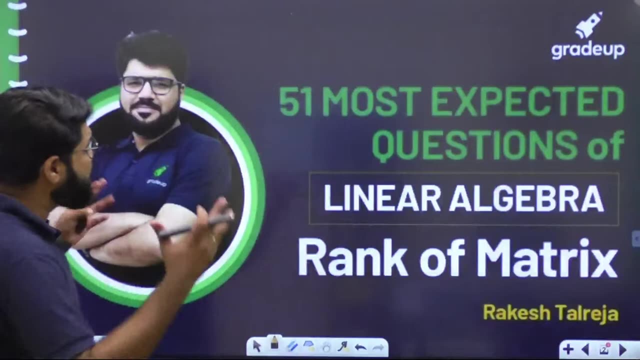 everything done so night, one hour practice of linear algebra. so, unlike the previous series where I was talking about- you know, last time I talked to you about expertise in probability, where we covered up all the concepts of probability and questions, important questions. so this is going to be a question based series. okay, but of course, 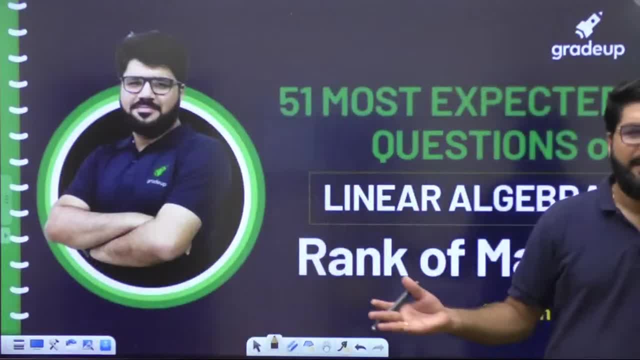 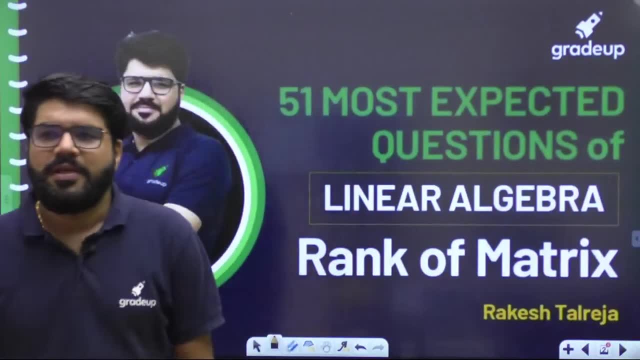 questions will associate concepts with it. okay, questions will, of course, associate the concept with it. right, absolutely, absolutely, pkpk, I'll take up some abstract questions and then I'll come back to you in the next session. you As well, don't worry. don't pull the full power. have done full power. let's see. 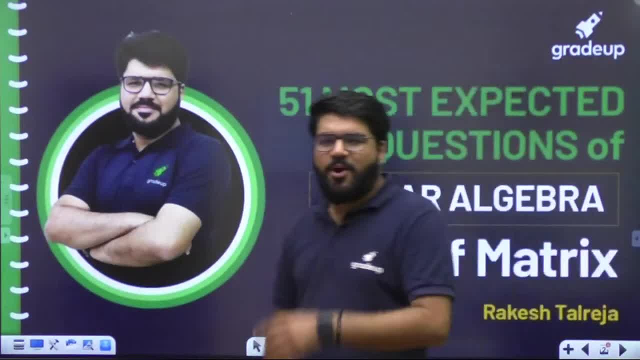 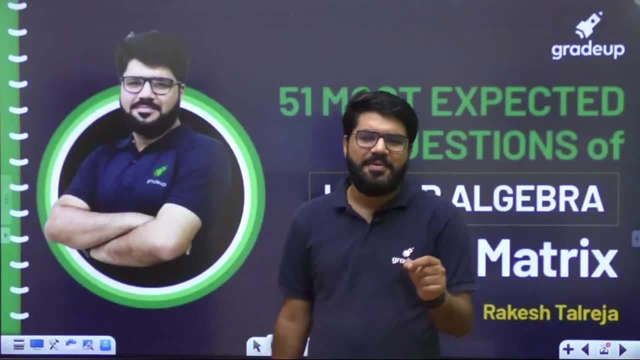 the full George, and let's you know, come on, everybody share. let me see how many of you have the high Joe's. usually, you know, every time we are ending the session at around 11 in 1115, but this time we are beginning at 1115, right? and 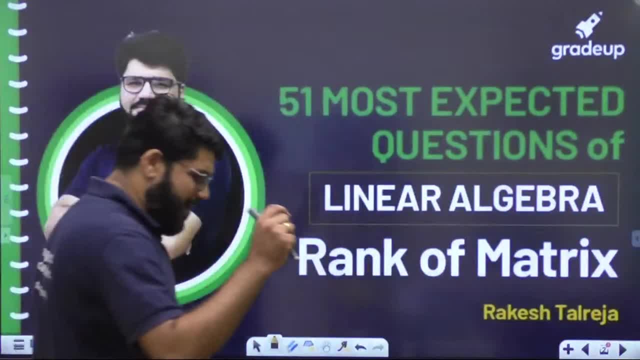 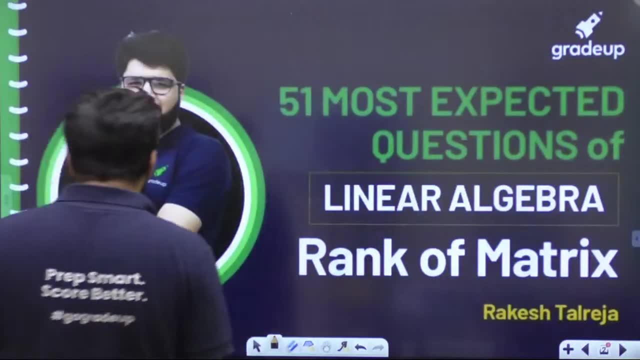 let's see how's the Josh? let go disco Panna. hey right, disco per na hemo que si be. time has a yoga. that's what I believe. okay, that's what I believe. so can we cross our comfortable times? I did not learn anything today, but I know some of the topics are important. friends, see you at school. don't forget to stay to the video. 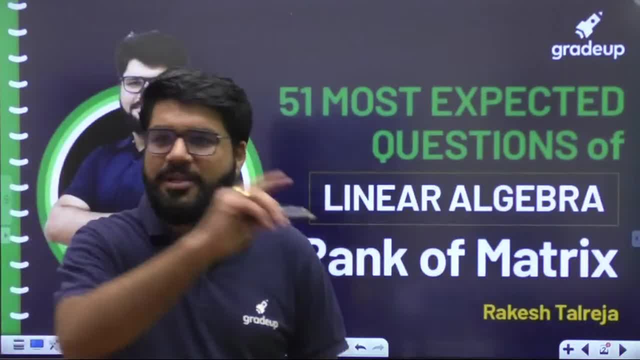 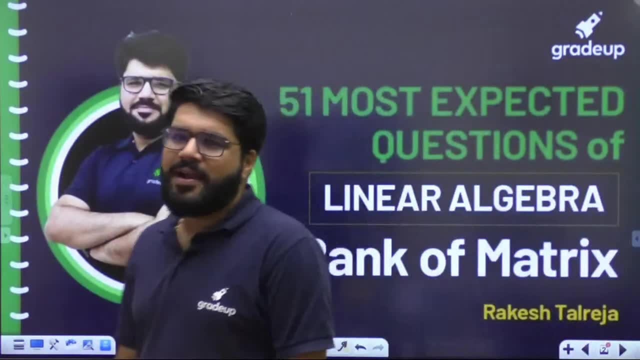 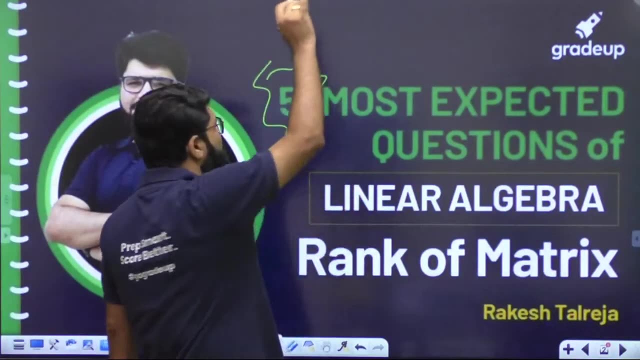 like evening and all, and can we study at any time? Do we have that much of passion? Do we have that much of enthusiasm for our preparation? Yes, Yes, it's a party type of questions. It's a party type of questions. Yes, Sandeep, sure. So, as the series says, 51, 51- most expected questions. 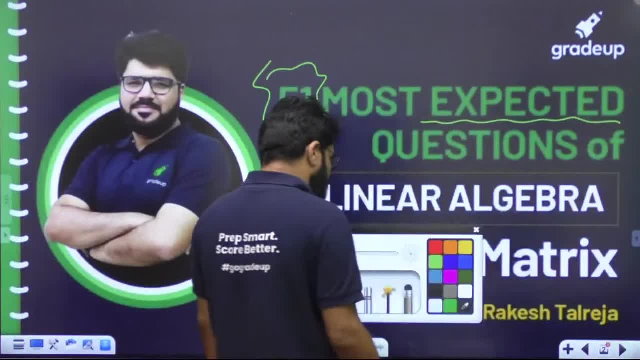 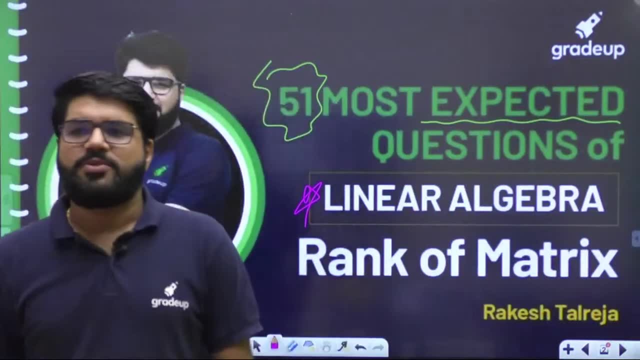 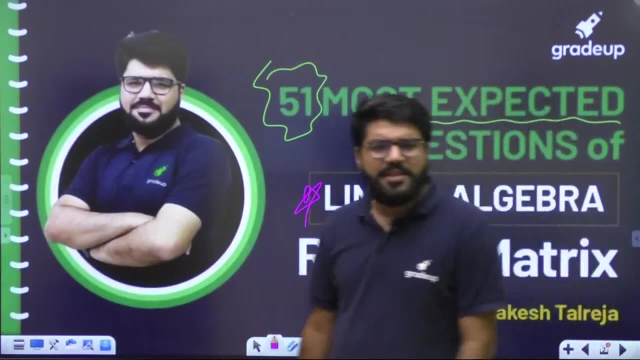 most expected questions of the linear algebra is what we are going to discuss? 51 most expected questions of the linear algebra. What is what we are going to discuss? Yes, yes, Basha, I have had high josh, high enthusiasm Lag raha hai mujhe, Okay, but still, the crowd should be more, I think. 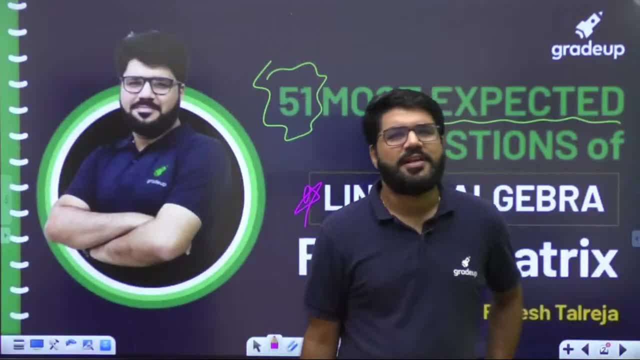 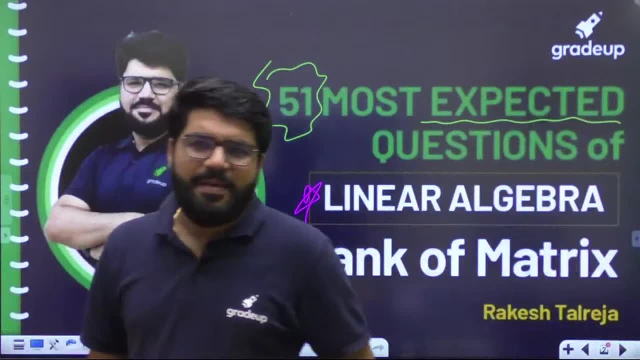 10 pm: more crowd. Yeah, it is the first class. It is the first class starting with rank because, as the series says, 51 most expected questions, right? So josh is lesser than 10 pm, josh kya. 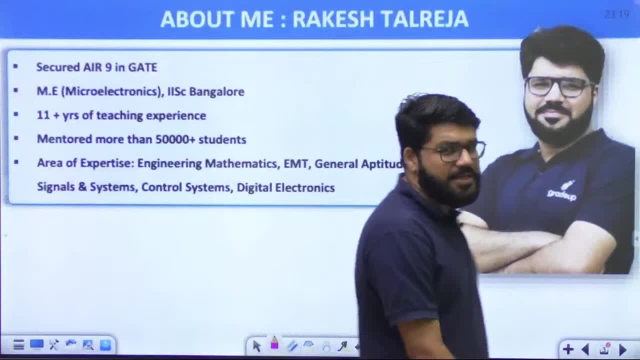 Check karte hain. Well, we'll wait for some time and then we shall be able to come in. So, guys, if any case is new to my session, if anyone, this is a new session. If anyone is new to my session. 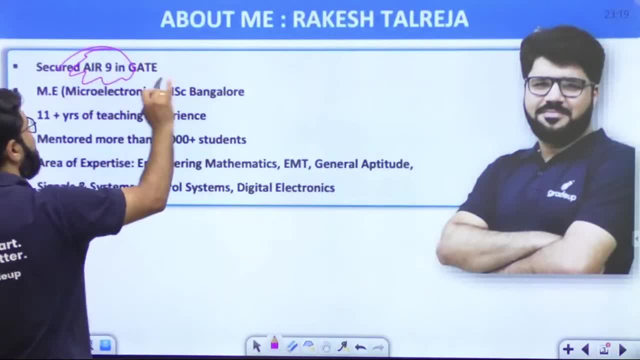 this is a brief intro about me. This is your mentor and educator, Rakesh. I have secured all India rank 9th in the GATE examination and pursued my master's from the Indian Institute of Science, Bengaluru right. It has been more than 11 years of this industry, training more than 50,000 students. 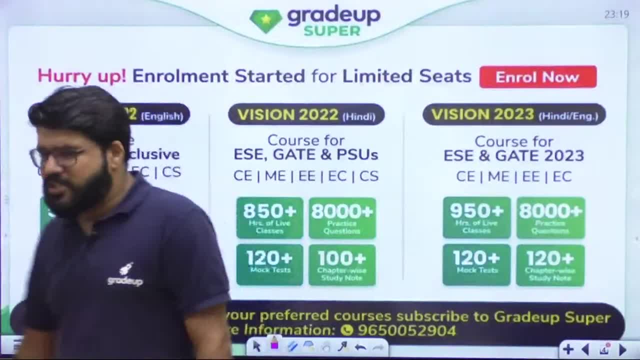 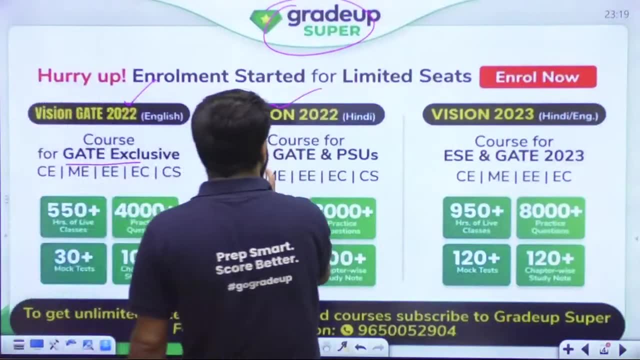 in my journey. Yes, So yeah. this is the. there are the several batches available on the grade of super. That is, the Vision 22 in English course for GATE, Vision 22 ESE, GATE, PSU and Vision 23 for the. 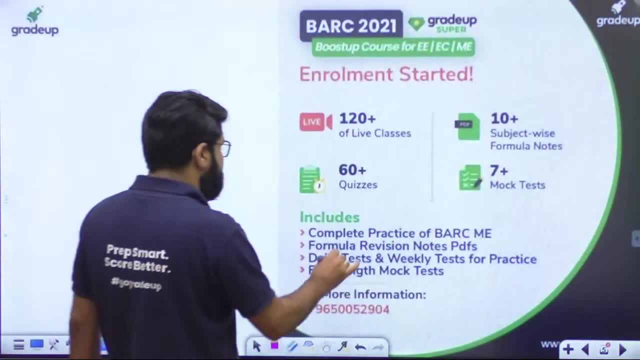 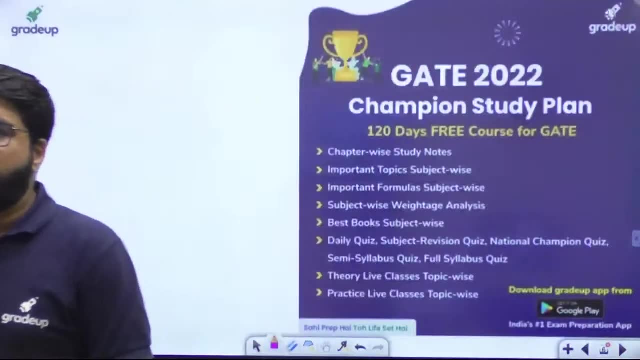 second year students. Next month BARC examination is there. So if you want the practice and revision course for BARC that is also available on the grade of super right For the self-study students, this is the GATE 22 champion study plan, offering you daily life classes, theory classes, 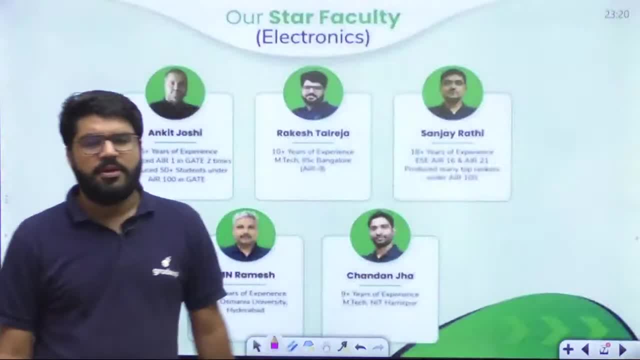 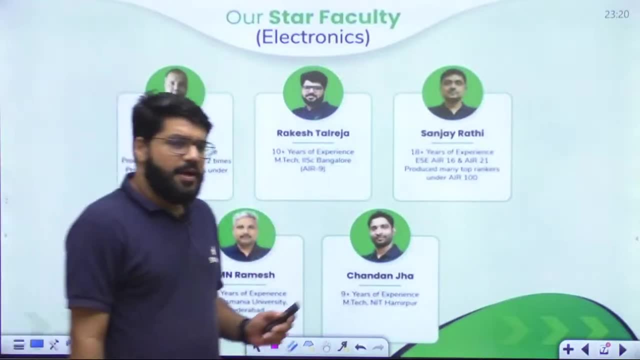 practice classes, daily quizzes, study notes- everything in this particular batch, This is the star and the most expert best faculty team of the nation for electronics and communication engineering right. This is the MMC makeup course for GATE 22.. So if you want to learn more about 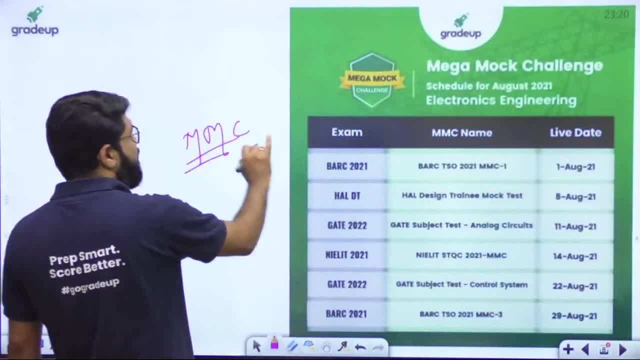 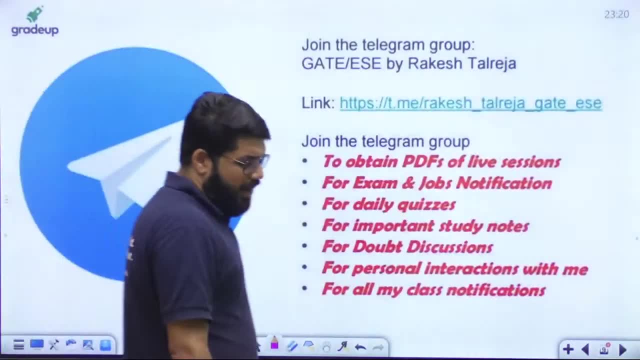 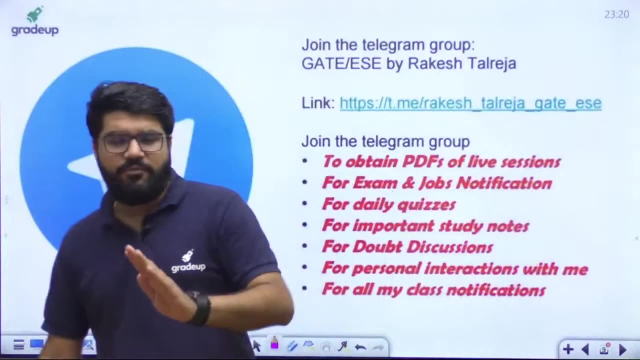 the mock challenge for electronics and communication. you can take the snapshot and appear on this challenges on the specified dates. right, right, right, right, right And guys. so what I only expect from you is the total concentration, dedication and attendance. Okay, If you want. 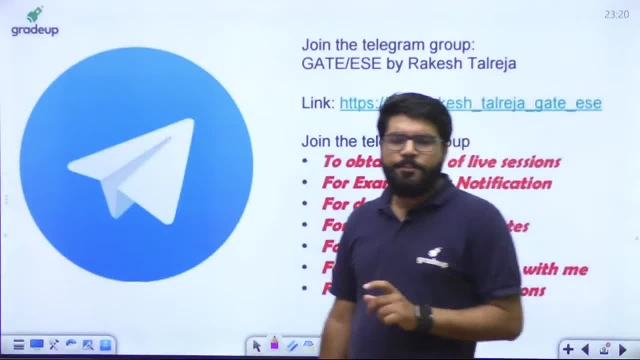 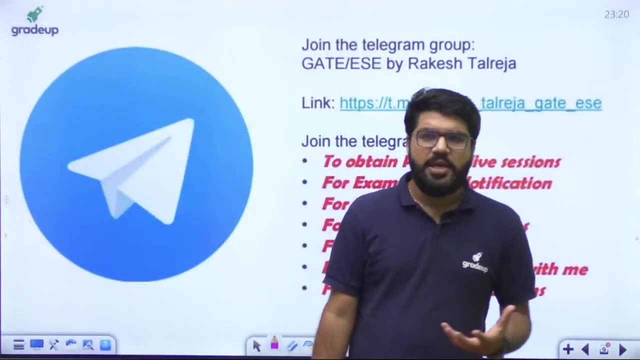 to get a command over the most expected questions of linear algebra. Okay, So you know, as this topic, as this name suggests, we are going to focus through questions, all important areas. I will give you the definitions, the theories that you can get from anywhere, but how to approach. 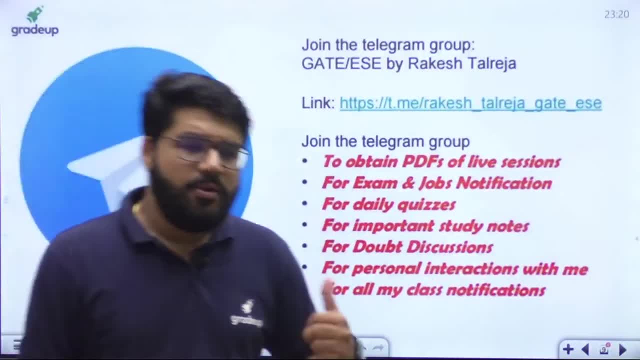 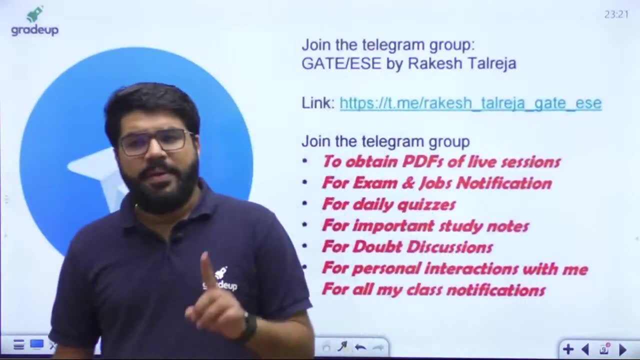 the questions of the most important category from the linear algebra Today is rank. I will tell you the complete schedule also at the last rank, then what? all the topics we are going to follow tomorrow? right PDF will be available at the telegram. That is what is the link of my telegram. 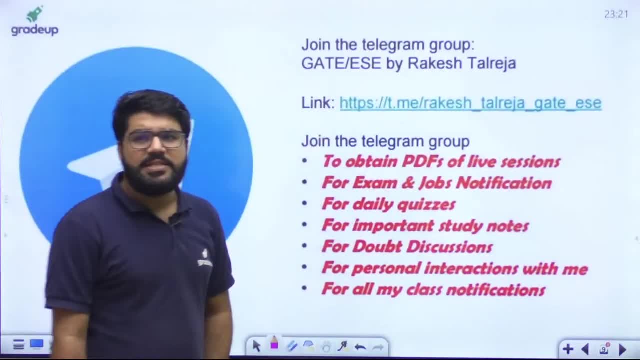 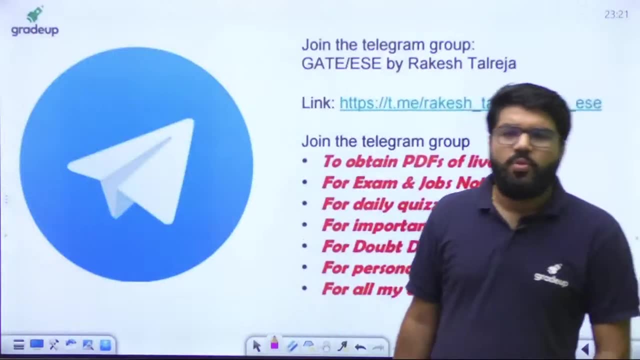 group. You can join my telegram group by the name GATE slash ESC by Rakesh Talreja, or I can share you the link also. I will share you the link also, Meanwhile, don't worry. So whatever we are discussing, just have your concentration, just have a pen paper. 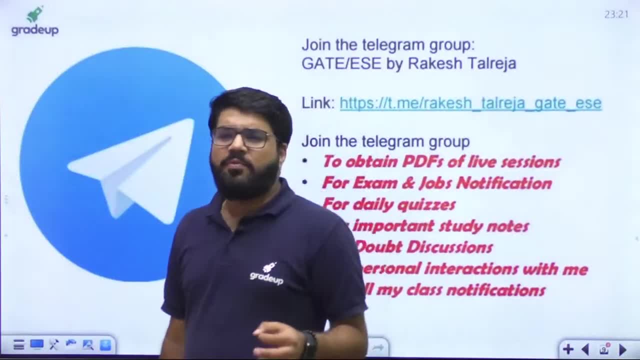 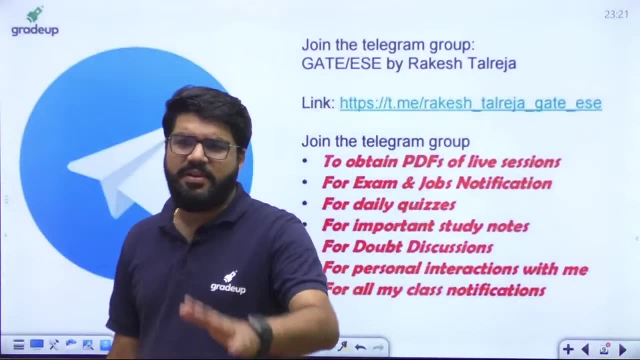 That's it And you know properly, are registered, to be precise, and whatever questions we are discussing, just start solving the questions there. But the rest, the detailed solutions, the detail notes, whatever we are discussing, will be there in the telegram. Okay, Right. 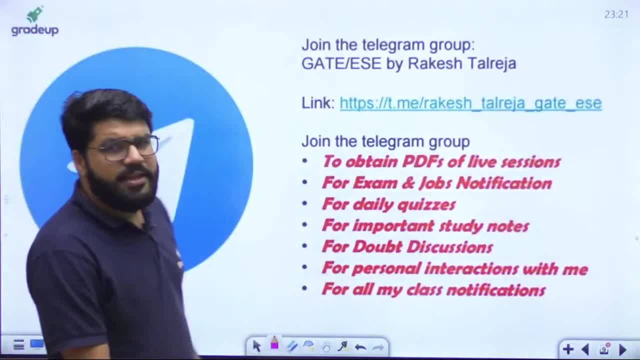 Chalo, Chalo. So I will tell you: Yeah, yeah, yeah, yeah, yeah, This is the first class of the series. Still, there are topics coming up. Okay, I will give you. I will give you. 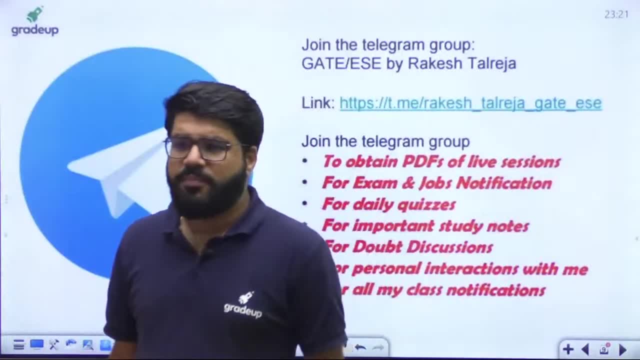 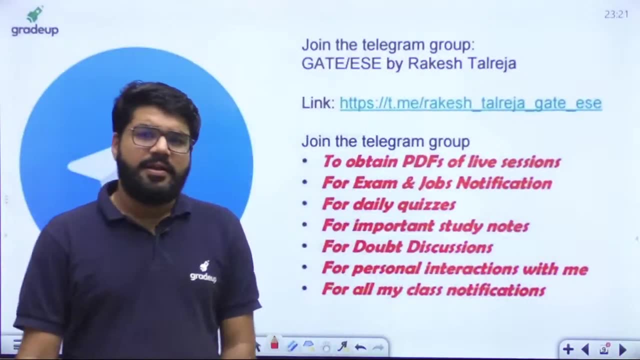 at the last, I will give you the briefing of the topics as well. I will give you the briefing of the topics as well. Need not worry, Chalo guys, Begin karte hain session ko Full enthusiastic session, Right, So how's the Josh guys? How's the Josh? Show me your Josh. and then the first. 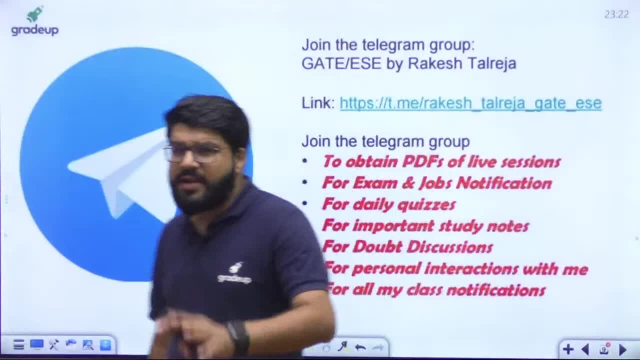 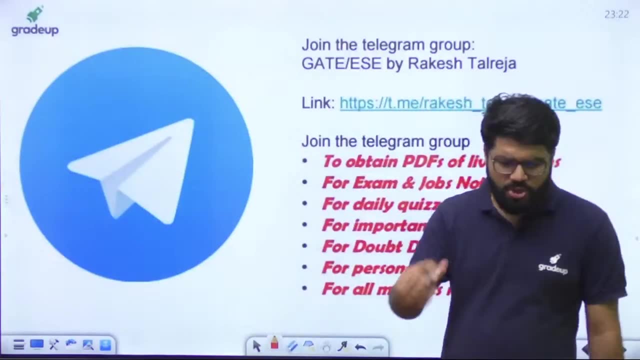 question coming up, And then the methods of solving various tricks. See, rank has methods and has lots of tricks. Okay, So how's the Josh? Show me your Josh through the comment box. Ek baar apne Josh ko highlight kar do Maza aa jayega thoda sa Right. And then I 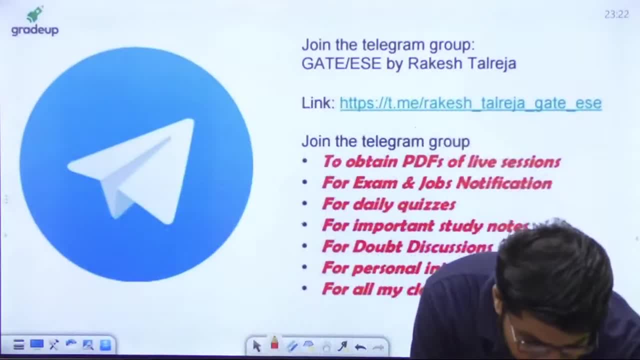 am going to present you the first question. Okay, By the way, I am going to present you the first question. Okay, By the way, I am going to present you the first question. Okay, By the time, I shall share you the link of the telegram. I will do that thing, but I want to see your. 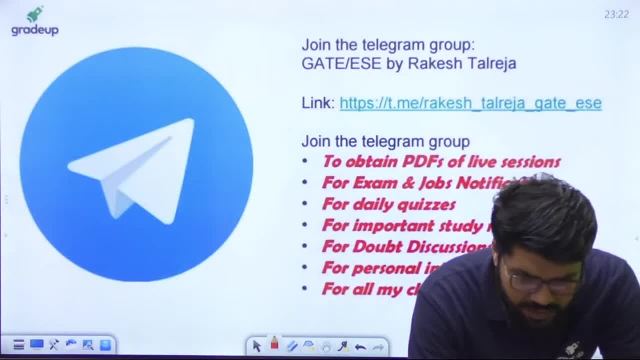 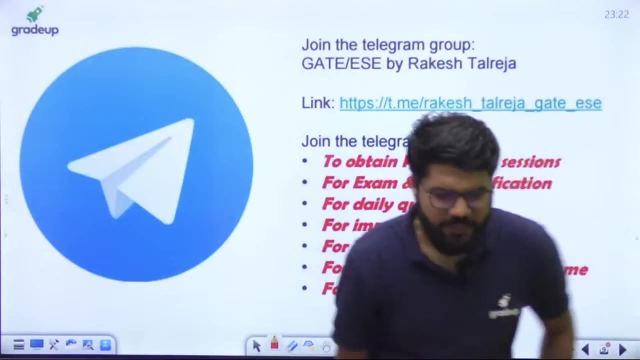 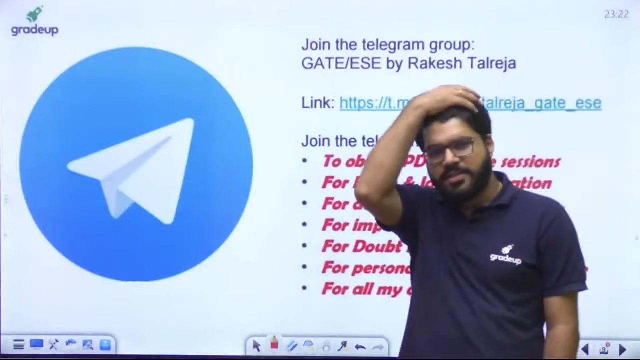 Josh, How's the Josh at night, 1122 PM. How's the Josh Show? it should be seen in the comment box. Akar Josh hain, toh, it should be seen in the comment box. Absolutely seen in the comment box. Hai hai, hai, yes, Yes, chalo. So let's catch up. Let's begin up the session. 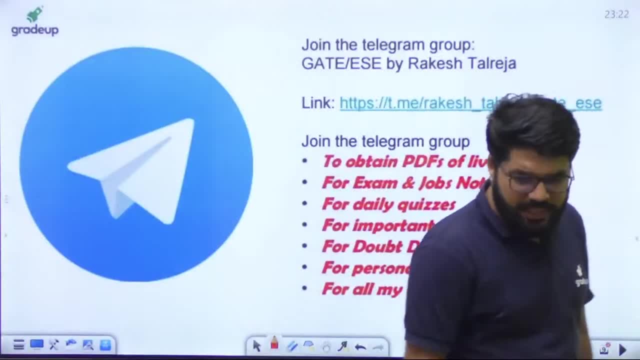 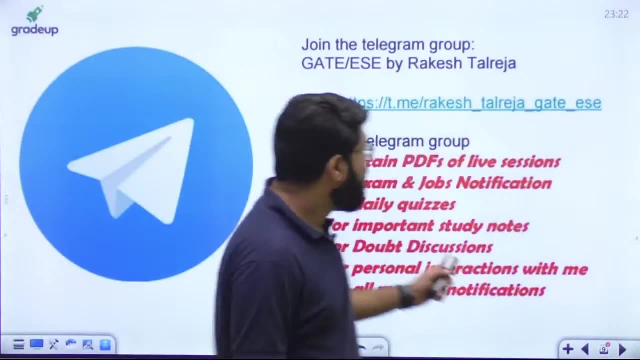 Okay, chats up and let's begin up the session enthusiastically. and yeah, this is what is the link of the telegram: those who want to join the telegram group for the pdf, the link is also shared with you. the question number one: here on your screen, find the rank of the matrix a, which is 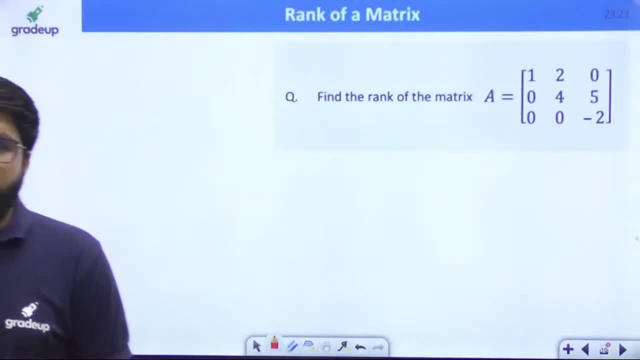 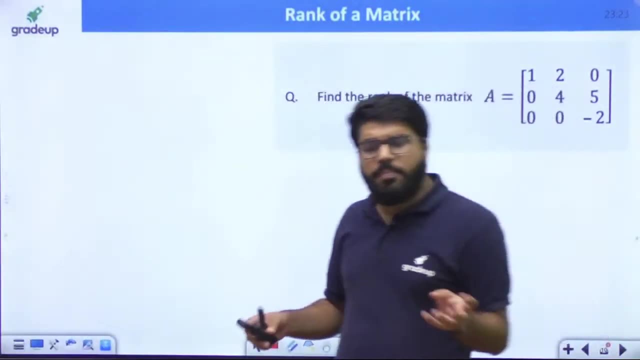 one, two zero zero four, five zero zero minus two. right zero zero minus two. now, what can be the first approach of finding the rank? there can be different approaches, i'm telling you or the tricks, but what can be the first approach to understand the first approach, you should know. 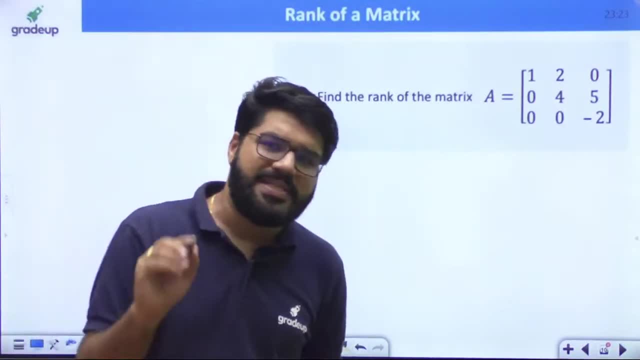 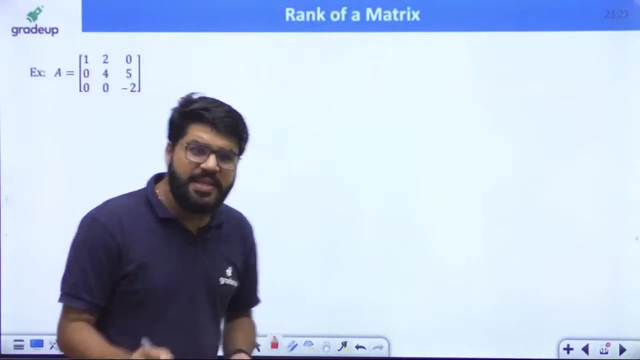 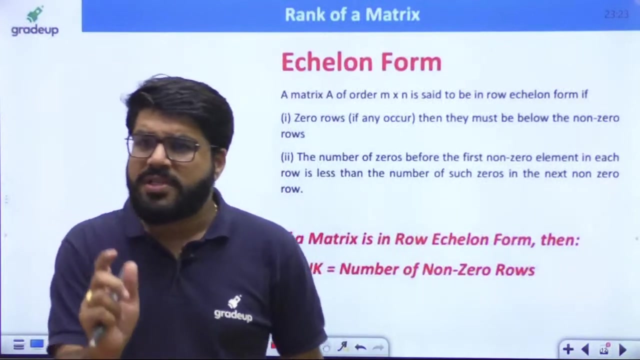 something known as the echelon form, right, so one, two, zero zero, four, five and zero zero minus two. let us get started with the question by basically what is known as the echelon form. so let's, whatever basic theory is required, we will revise the theory also, but mostly it is the question. okay, yeah, so 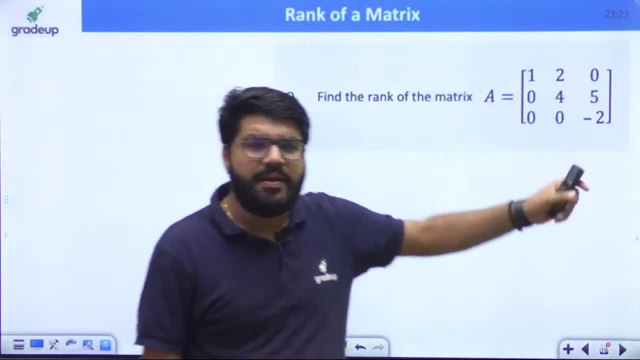 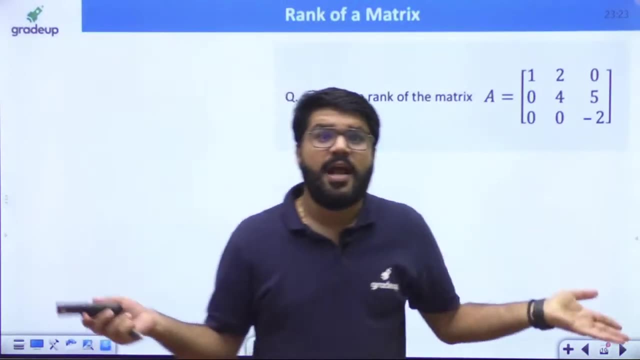 you are ready to comment, guys. so some of you are ready to comment. what is the rank of this matrix? it is just a matter of you know how you can tell the rank of this matrix. oh my god, it's three. yes, the answer is three, sir. how? how? that far, there are two, three ticks, starting with the first echelon form. okay, guys, so echelon. 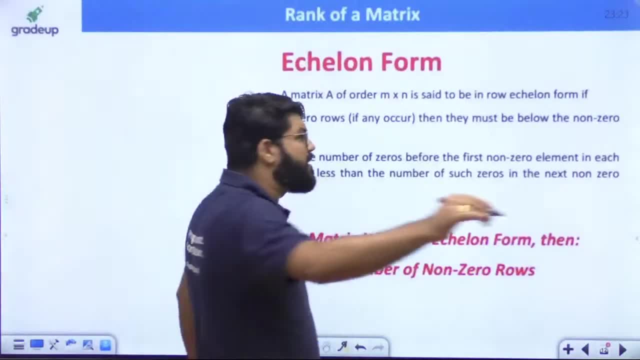 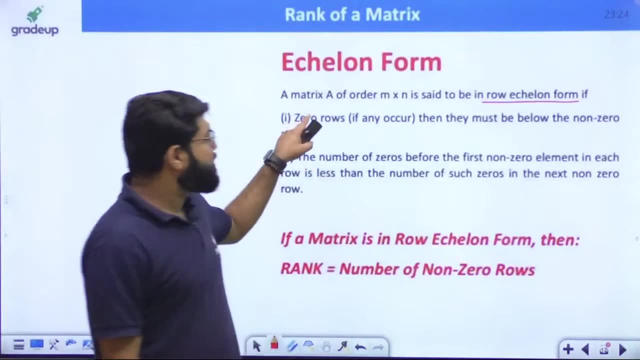 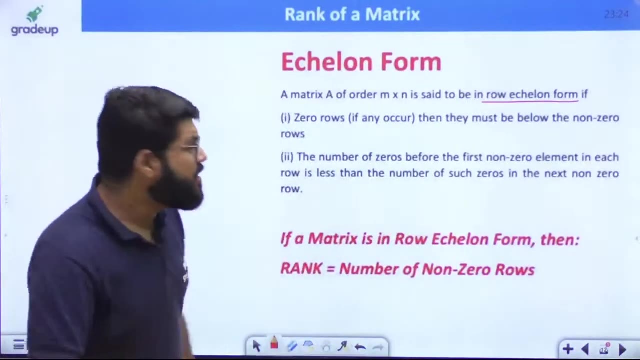 form or precisely row echelon form, precisely the row echelon form. already, the rank is three in the comment box. so basically, what is the echelon form? a matrix a of the order m cross, n is in the row form. if zero rows, if any, if there is any row of zero. 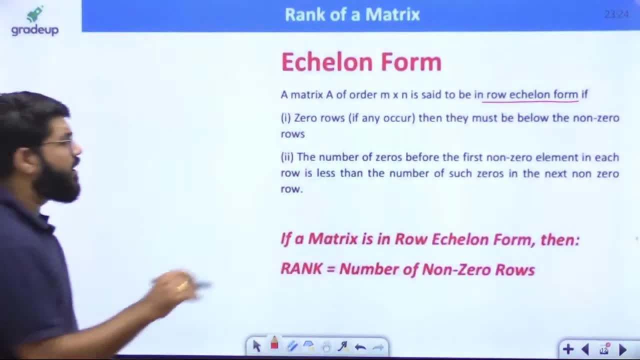 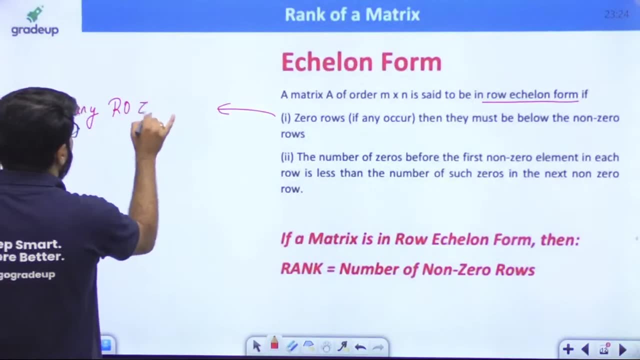 they must be below all the non-zero rows. I will write down in short. I will write down in short: if there is any row of e? r o, z means row of 0, full row of 0. if there is any r? o z, it must be at last. 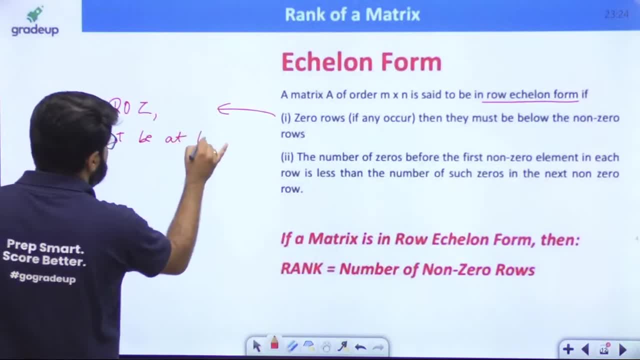 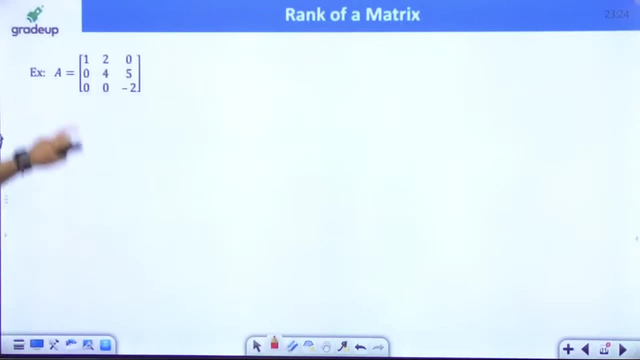 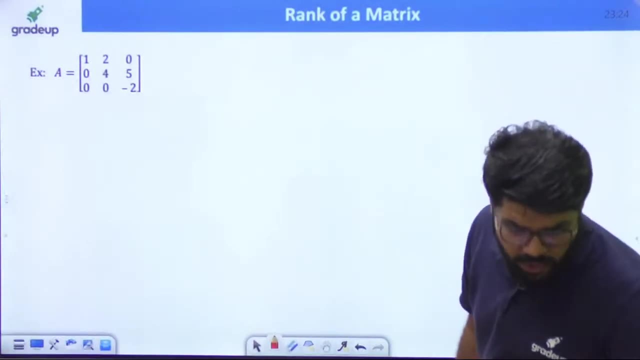 below all the non-zero rows. it must be at last, okay. so have a look at this given question. the same question is copied here: one, two, zero, zero, four, five and zero zero minus two guys. is there any zero, sir? it's their voice cut or a voice not clear. let me just hear. let me also. 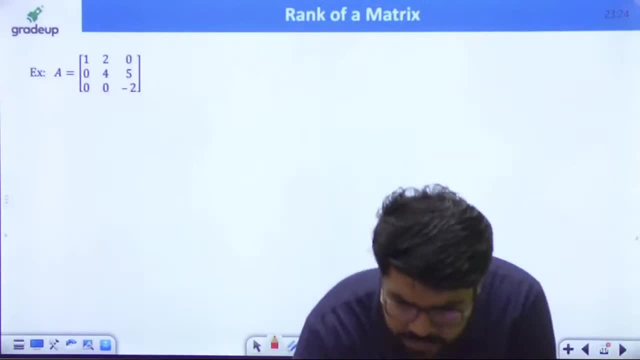 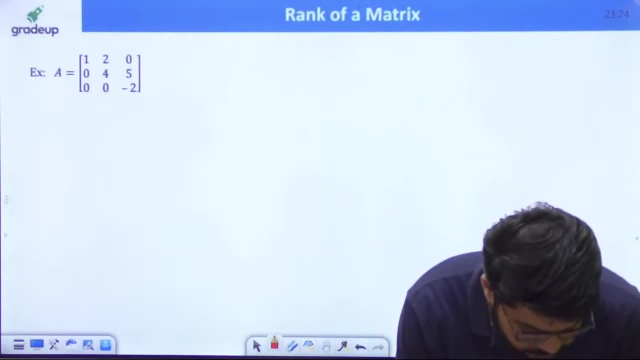 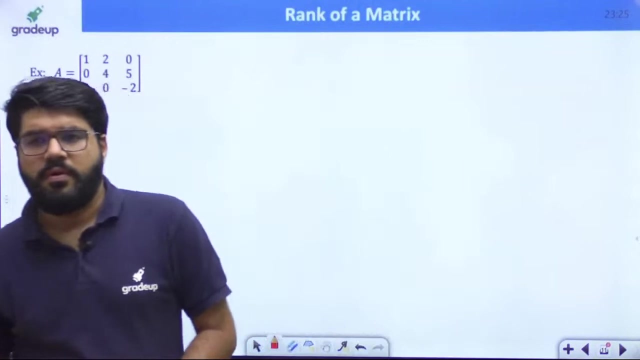 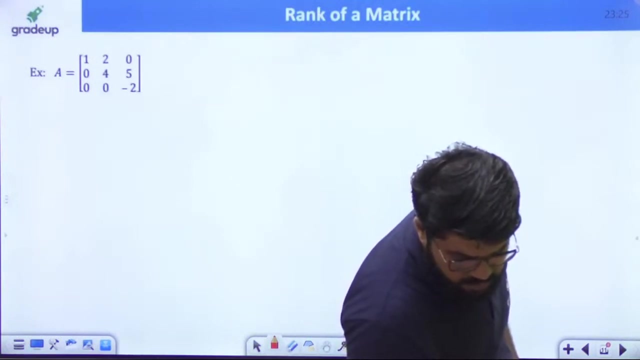 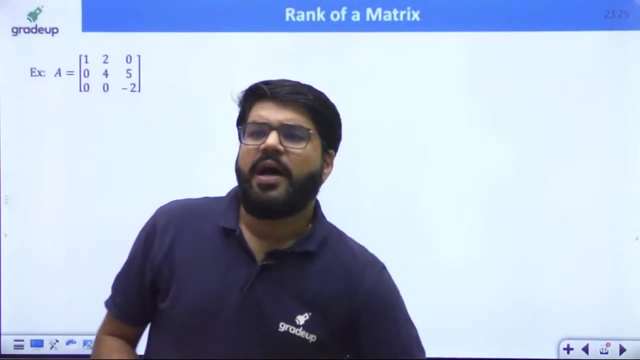 hear it, guys, let me also hear it up. why I am NOT able to hear it up, this, the voice low? let me just check it out, you know? no, no, I think I think it's clear. I'm able to hear it. I'm able to hear it, ok. ah, yes, it's the PK sort of you. 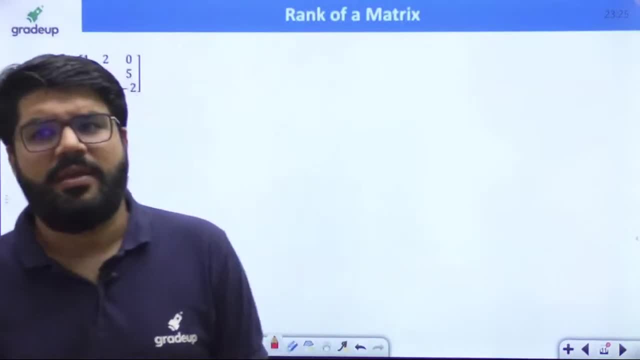 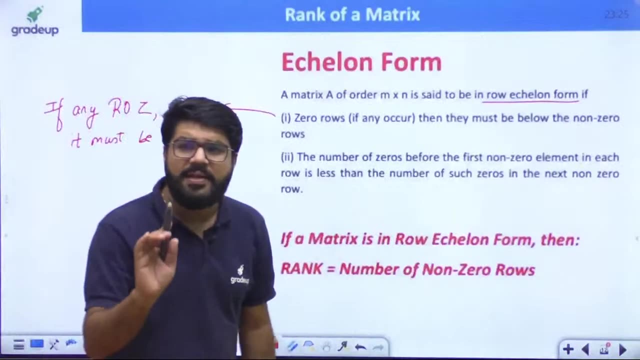 team, but there may be cases where u TM is not bucket, so I'm just calling it as a Klenform. so, guys, the first you need to understand, guys, which is what I'm seeing, which is absolutely point: if there is any row of zero, it must be at the last, it must be at the 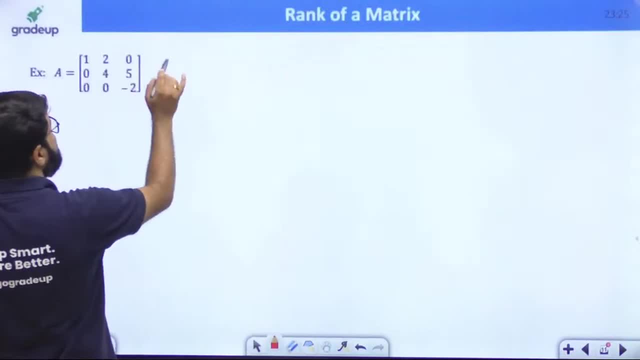 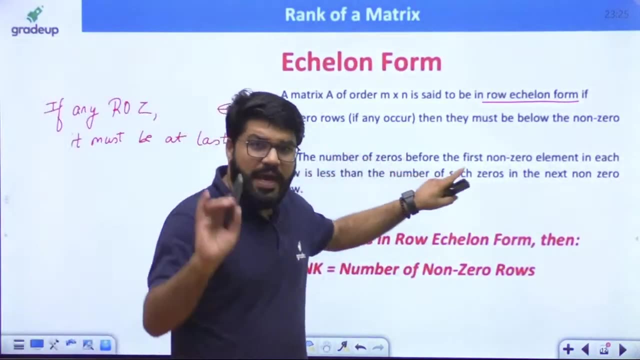 last. okay, do I have any row of zero? sorry, do I have any row of zero, sir? no, now read the second point of the echelon form. the number of zeros may hurt you. simple Karuba: the number of zeros before the first nonzero element in each row. 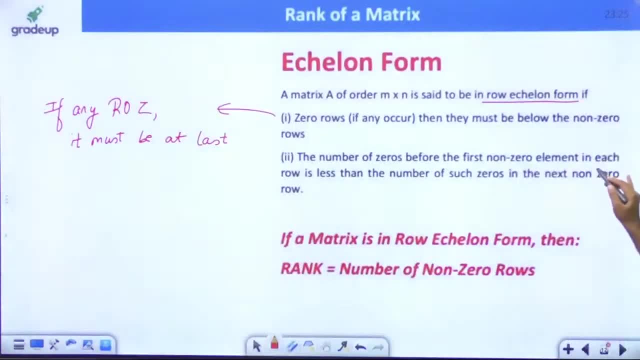 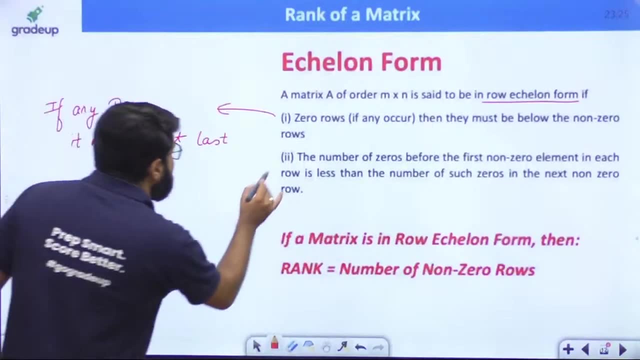 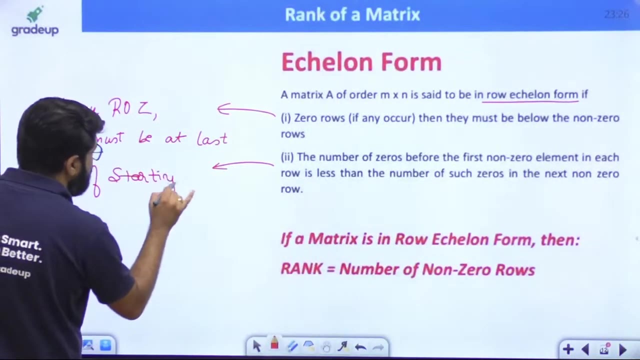 the number of zeros before the first nonzero element is each row is less than the number of surge zeros in the next non zero. let me make it simple. let me make it simple that the number of starting zeros- I call it on number of starting zeros- number of starting zeros must follow, must follow increasing order. 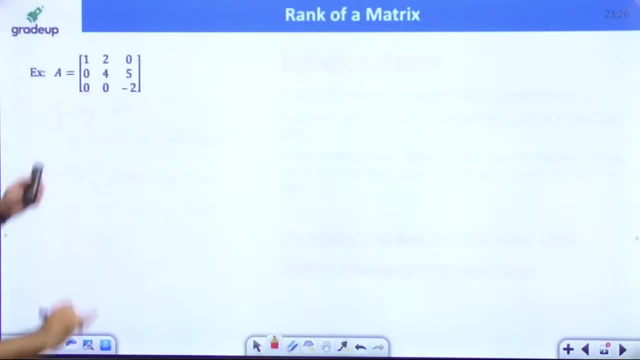 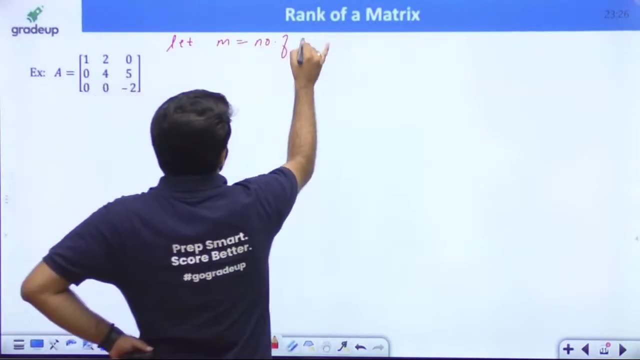 okay, must strictly follow the increasing order. now let us try to understand this point here. let us try to understand and let me write down: let M is equal to the吃 to number of starting zeros. Once you understand that, then questions will be easy, And then 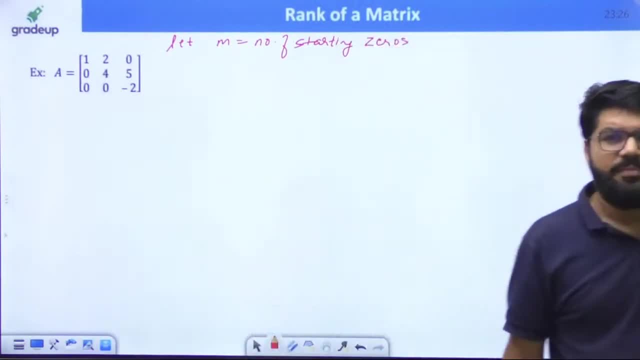 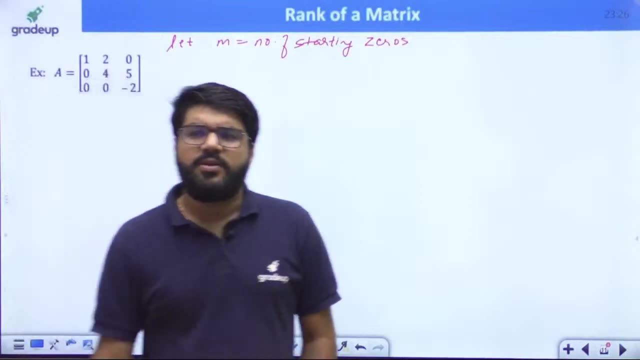 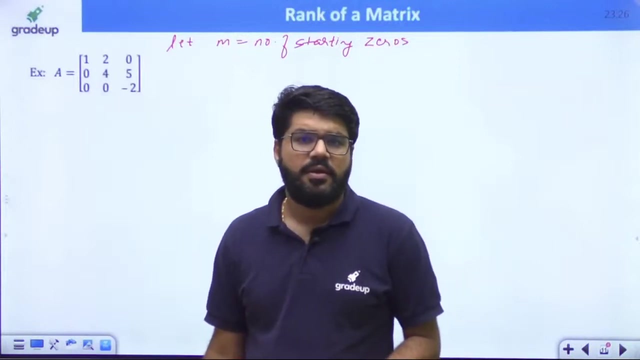 I am going to tell you a second alternate trick. will be wonders. Okay, will be wonders. Right, Right, right, right Now. guys, I just tried to listen- I think the voice was fine- Why it is creating the problem for students. I am not able to get that, Isn't it fine? 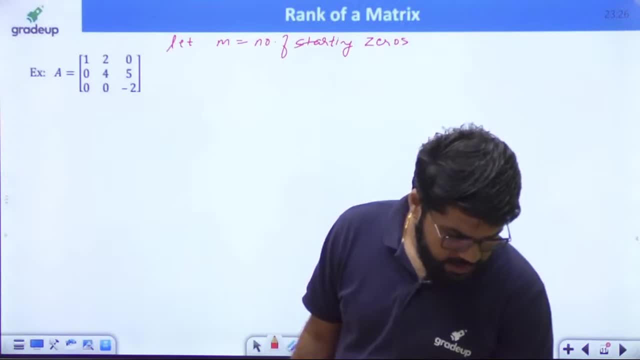 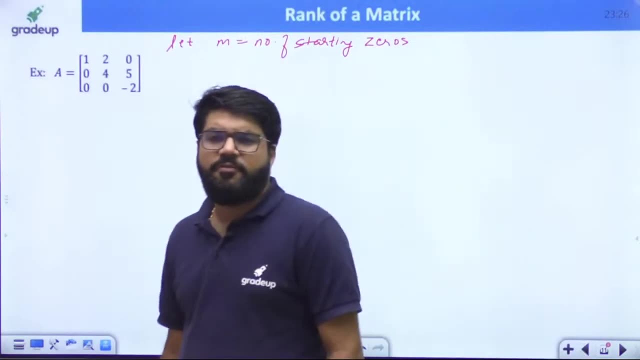 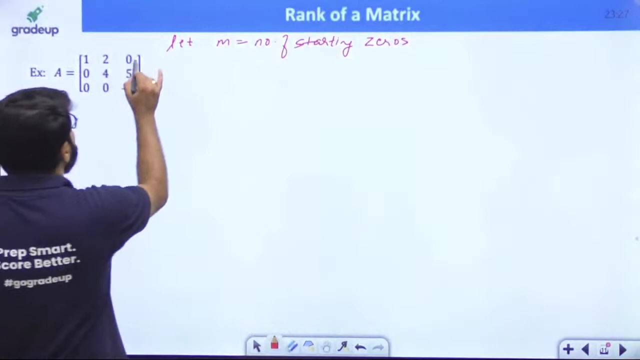 Let me again, again, again. Let me keep checking it. No, no, guys, voice seems fine for me. Maybe you can refresh once. guys, You can refresh it. Let m is equal to the number of starting zeros. Okay, so how many starting zeros guys in this? 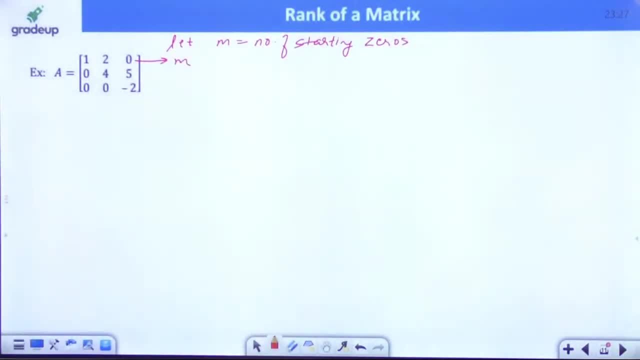 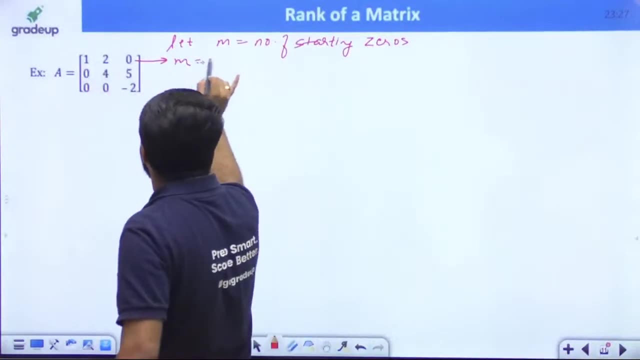 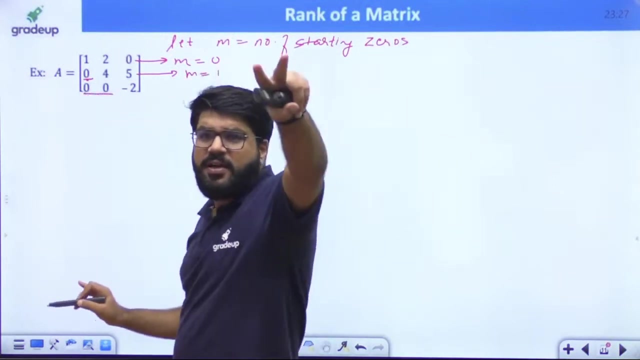 row: Okay. how many starting zeros here? Okay, starting means the beginning. Let's see the word clearly: Number of starting zeros, which is going to come in the beginning. So, how many starting zeros here, Sir? zero, How many starting zero? One M is equal to one. How many starting zeros here? 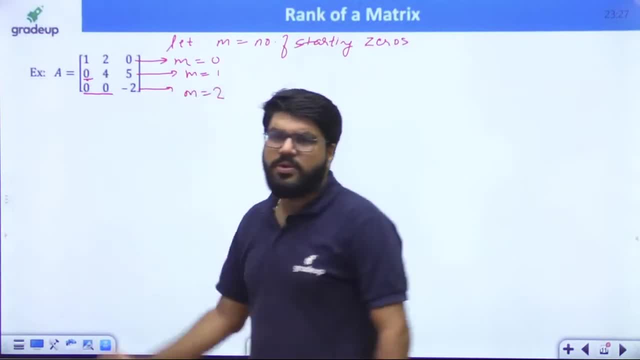 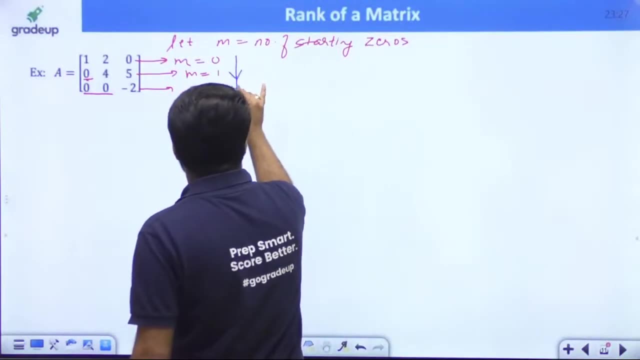 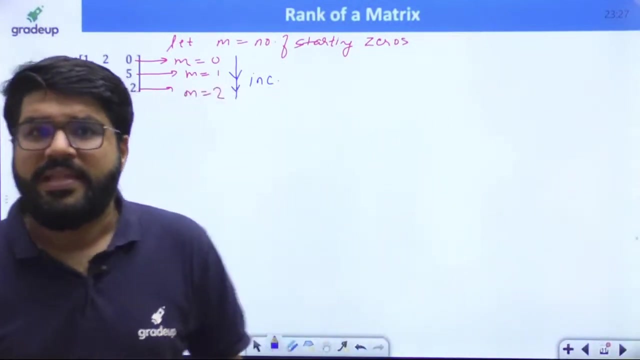 Sir, two M is equal to two M is equal to two. So do you see that the number of starting zeros are in the increasing order? Yes, sir, The number of starting zero is in increasing order And that is why it is in the echelon form. That is why it is said to be in echelon form, Right. 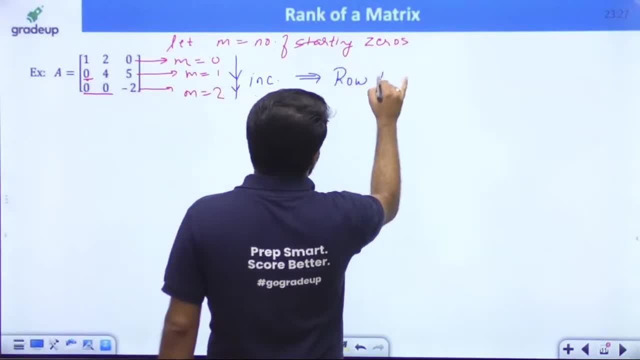 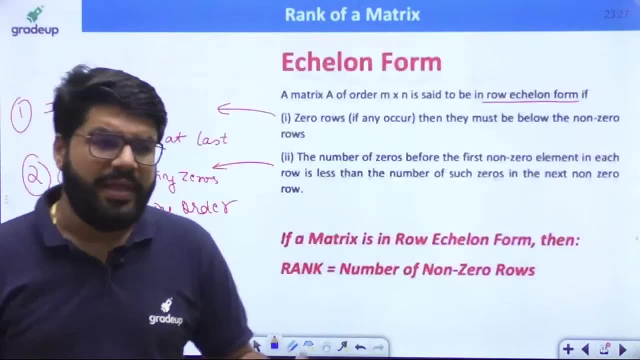 That is why this is clear Clearly in the row echelon form There are two conditions of the row echelon form. I will again repeat: There are the two conditions for the matrix to be in the row echelon form. Okay, If 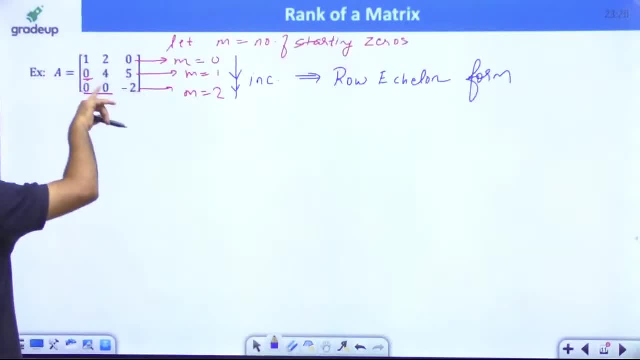 there is any row of zero, then it must be at the last. Sir, there is no row of zero. Row of zero means complete, full row of zero And the number of starting zeros must follow the increasing order. So, yes, zero one, two. increasing order: Yes, Okay, yes, So if it is in the row echelon form. 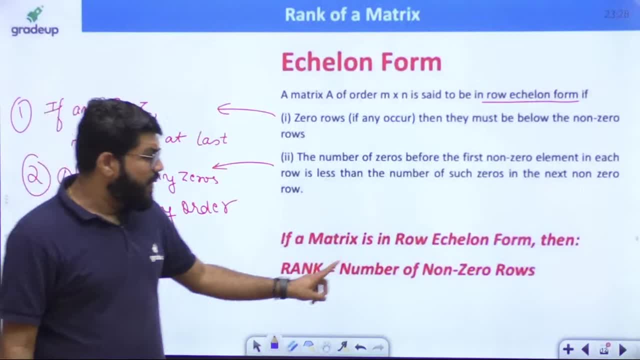 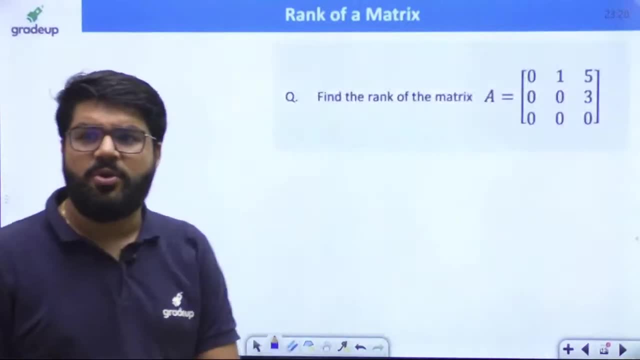 if a matrix is in row echelon form, then it must be at the last. So if it is in the row echelon form, echelon form, then rank is equal to number of non-zero rows. then the rank is equal to the number of non-zero rows. so how many non-zero rows you are able to see? okay, yes, akhil tej, determinant. 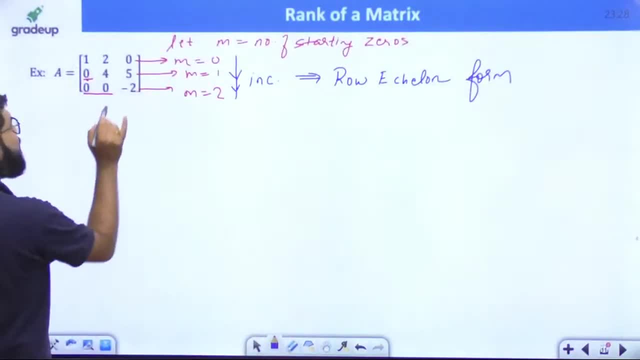 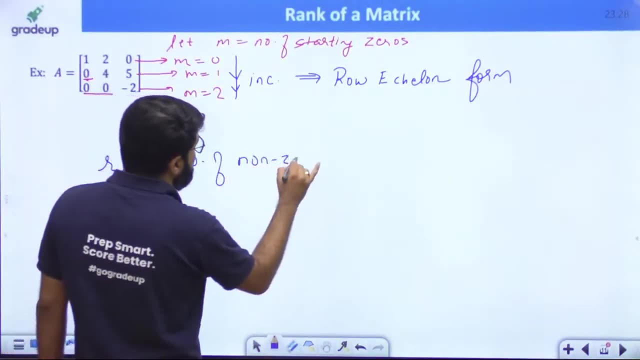 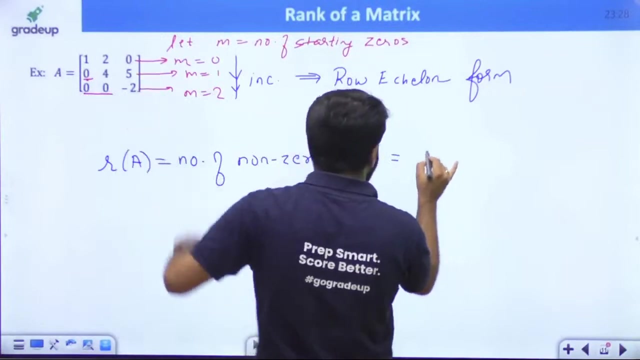 is minus a, maybe minus 8. agree, no need here. okay, what is the rank of the matrix? a is equal to, in the echelon form, number of non-zero rows. this is: this is applicable for echelon form number of non-zero rows. and how many non-zero rows, sir? one, two, three? it is three now, if this is understood. 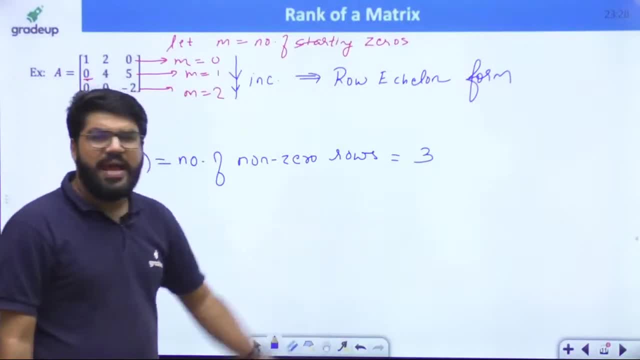 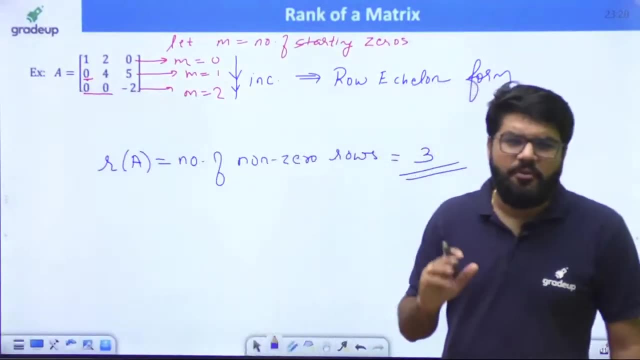 once. now let's try to apply on the next question. okay, the rank of this matrix is equal to three. the rank of the matrix is equal to three. so first i'm trying to explain you the echelon form, then some other things like determinant and all. okay, determinant and all, yes, yes, it will come for the 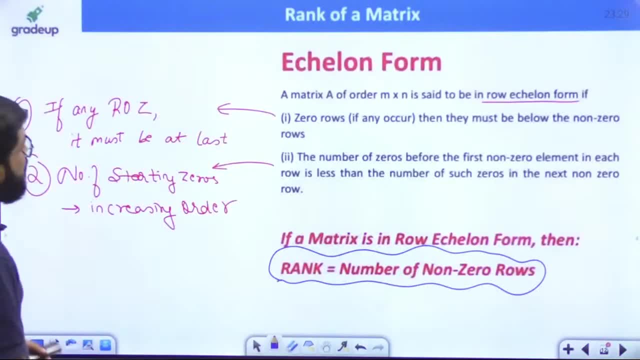 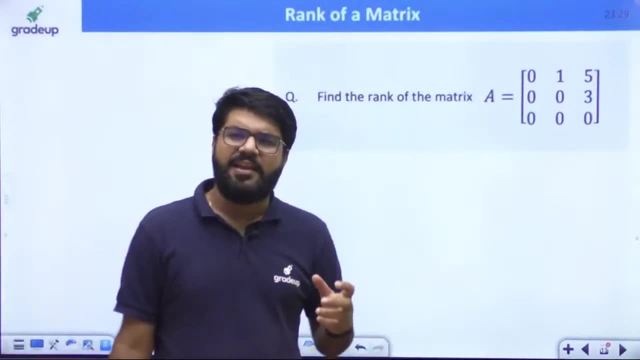 first case also vasu, don't worry, all other cases will come, need not worry. okay, here it is. find the rank of the matrix, everybody. first let us, you know, you know, impart in our brain what is echelon form, then determinants, dependency method. there are two, three methods. 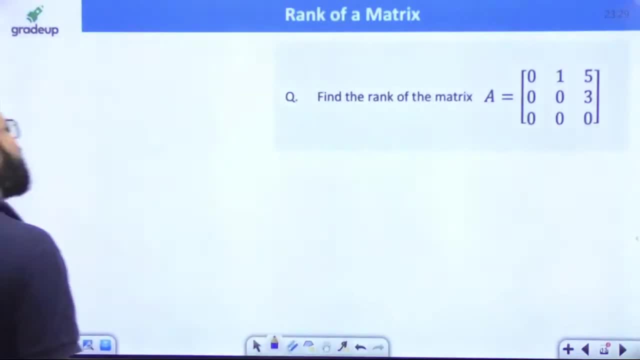 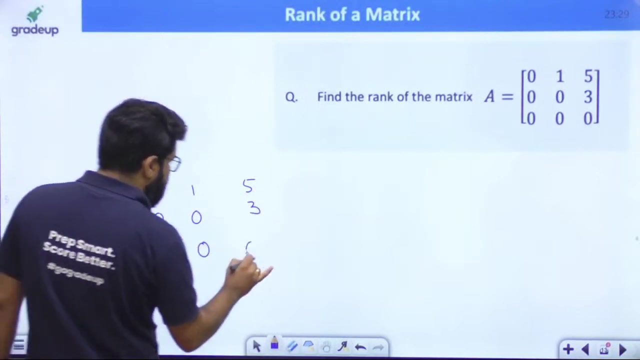 I am telling now, just let's wait, tada sotto more, to downright find the rank of the matrix: zero one, five, zero, zero, three, zero, zero, zero. tell me zero one, five. let me just copy it here: zero one, five, zero, zero, three, zero, zero, zero. what should be the rank of this matrix? what should be the 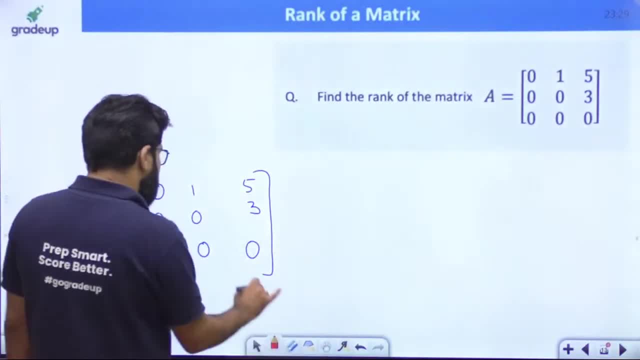 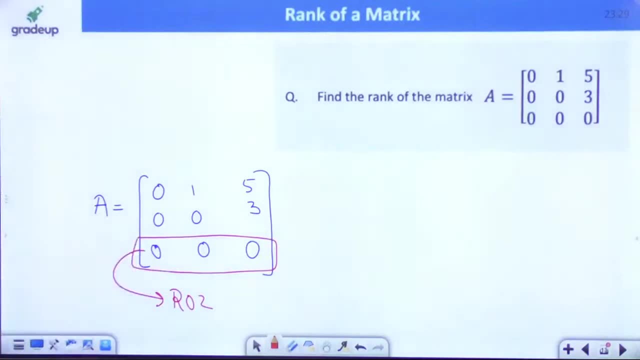 rank of this matrix, sir? what should be the rank of this matrix, sir? Sir, look, this is what is rho of 0.. This is what is meant by rho of 0,. okay, Complete rho of 0, and it should be at last. 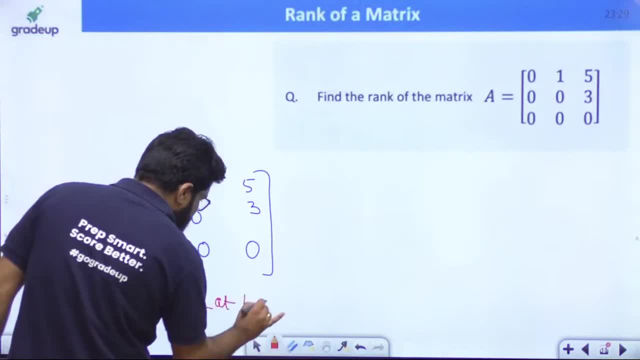 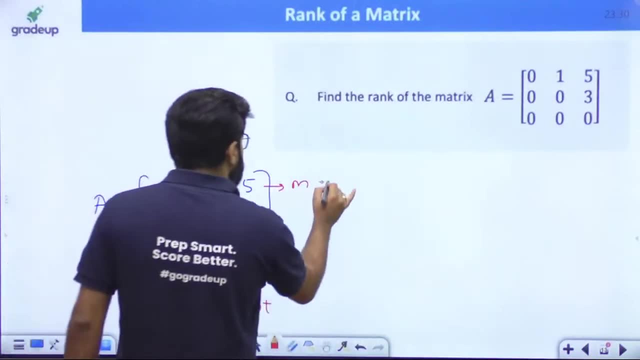 Yes, it is at last. Rho of 0 is at last. No issues, sir, Then M. I will keep the same definition. Let M is equal to number of starting zeros. Let M is equal to number of starting zeros. 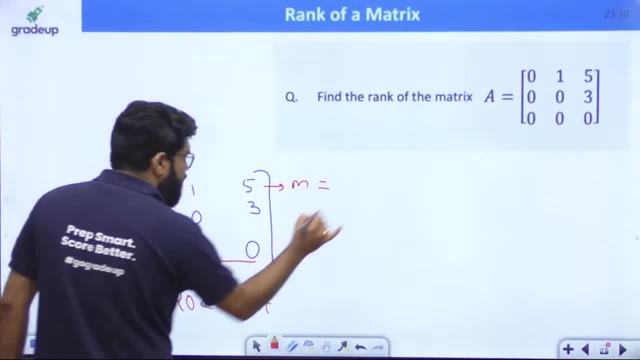 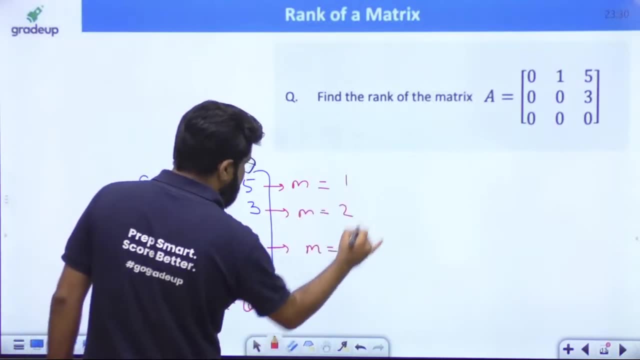 How many starting zeros are there? 1, then 2 and then 3.. So M is 0.. Sorry, M is 1.. Then M is equal to 2.. And then M is equal to 3.. Yes, it follows the increasing pattern. 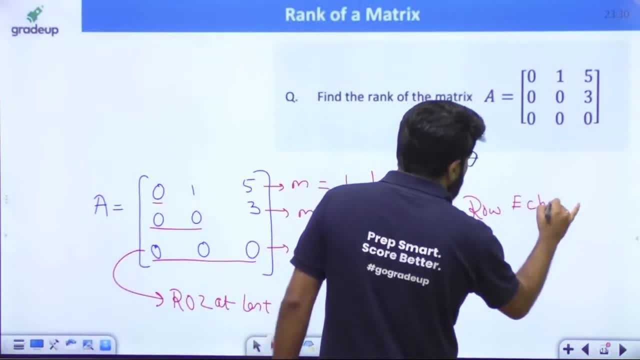 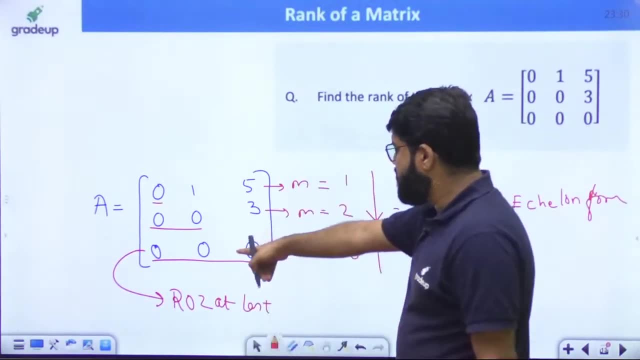 So that means your matrix is in rho echelon form. The matrix is in rho echelon form. Okay, so what should be the rank of matrix? Number of non-zero rows? The last one is 0.. How many non-zeros? 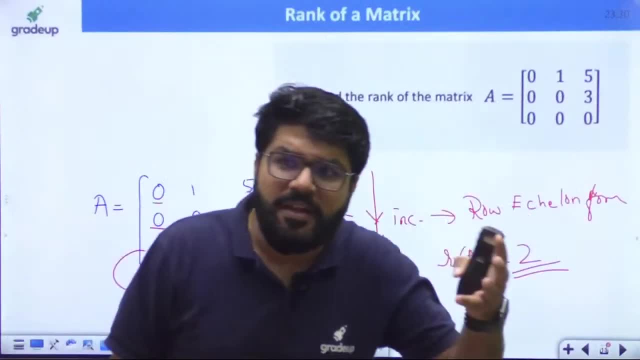 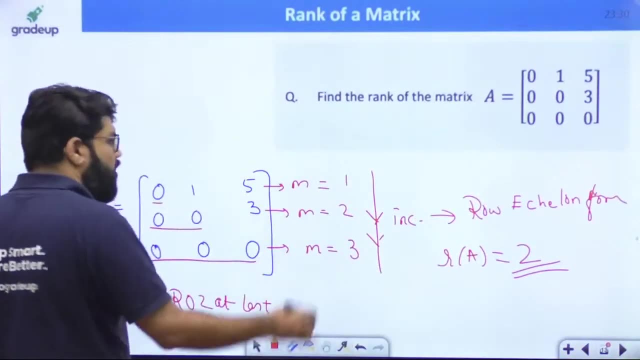 2 non-zeros. The rank of this matrix is 2.. See for your description. I am writing it Okay, but actually do you need to write down in the GATE exam? You need to just get the answer and mark the correct option. 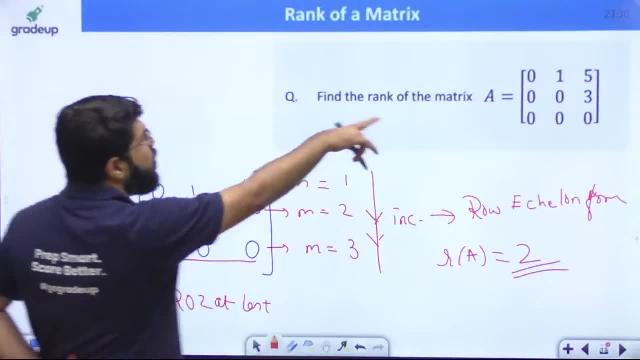 Or, if it is NAT, write down the answer. It's a matter of observation. Okay, okay. okay, Sir rho of 0 at last. Okay, Then 1,, 2,, 3.. Increasing or the number of 0?? 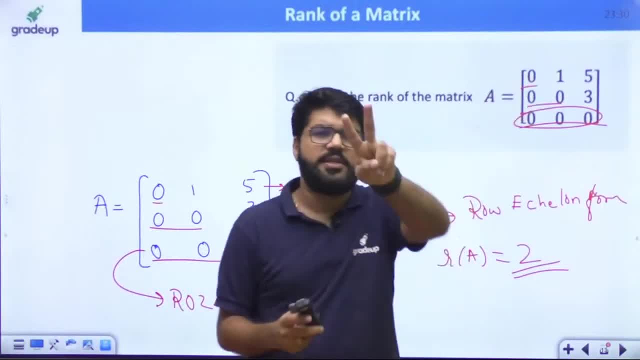 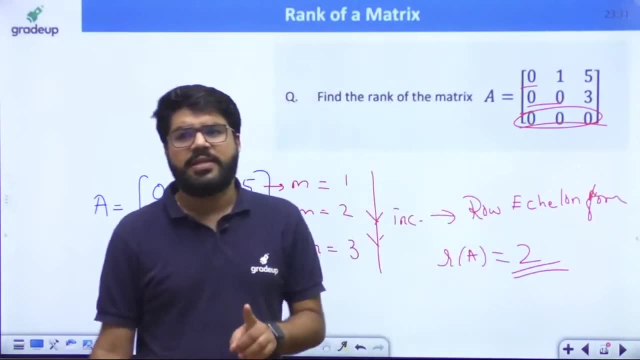 Yes, Rho echelon form. The answer is number of non-zero rows. Answer is 2.. Simple, So you don't have to write down anything. It's an observation-based question. Akhil Tej, I request you for the last time, please comment once. 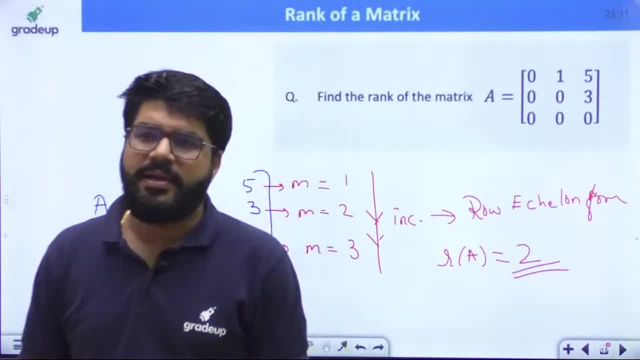 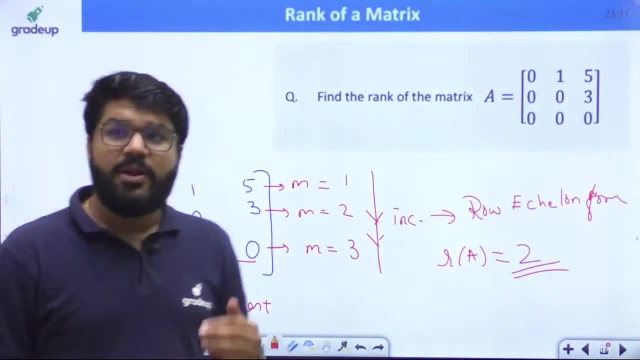 Please comment once I am able to get it clearly. Need not, you know, comment it repeatedly, Akhil Tej, Otherwise I will have to time you out Both, both. But rho of 0 is not necessary every time, Chandrashekhar. 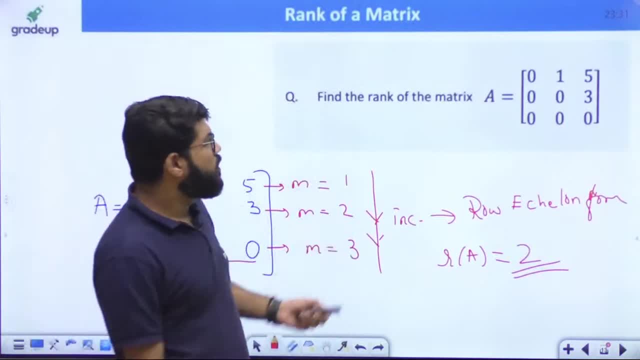 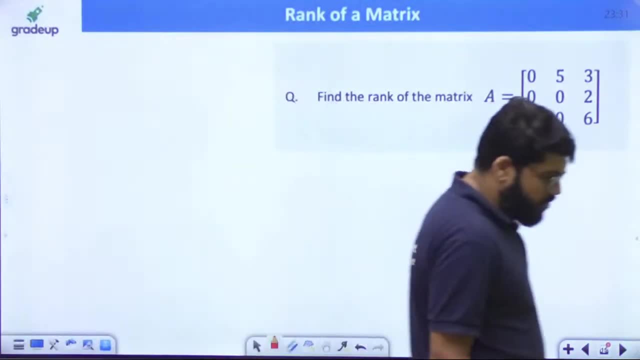 Whenever there is a rho of 0,, that must be at a last Right. Come on, Tell me the next answer. then. Tell me the next answer, then. What is the rank of the given matrix? What should be the rank of the given matrix? everybody. 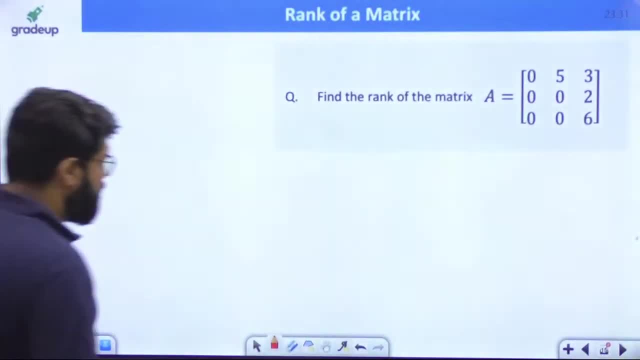 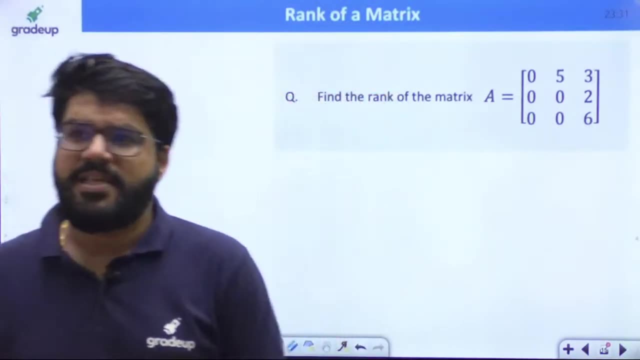 What should be the rank of the given matrix? Okay, First again, let us you know, practice some on echelon form, Then we will go to the determinant, And then we will go to the another trick of dependency and independency. 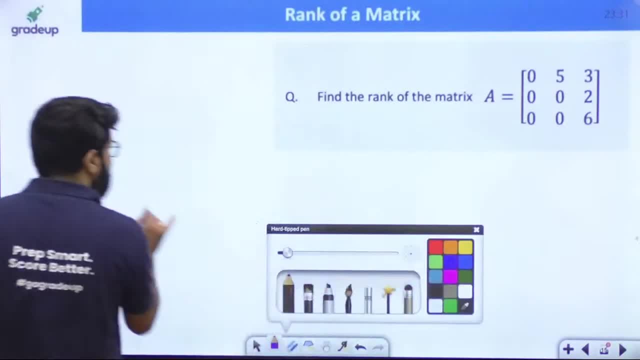 Method: 0, 5,, 3,, 0,, 0,, 2,, 0,, 0, 6.. Everybody, let us write down, Let us just copy this matrix here: It is 0.. It is 5.. 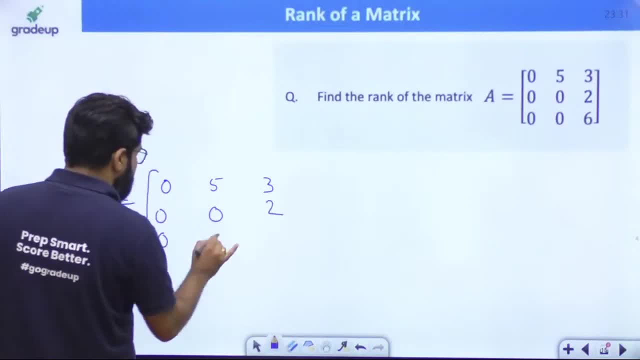 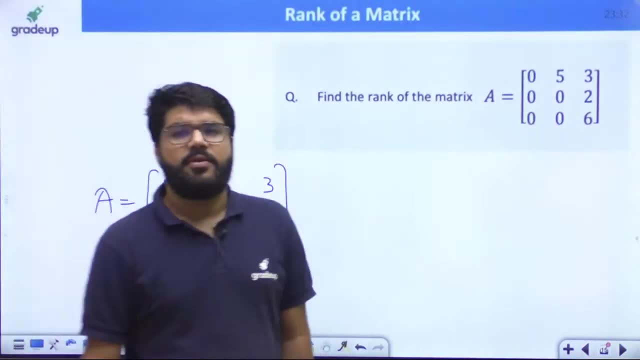 It is 3.. It is 0.. It is 0.. It is 2.. It is 0.. It is 0.. It is 6.. Is there any rho of 0?? Yes, tell me Right, Look. 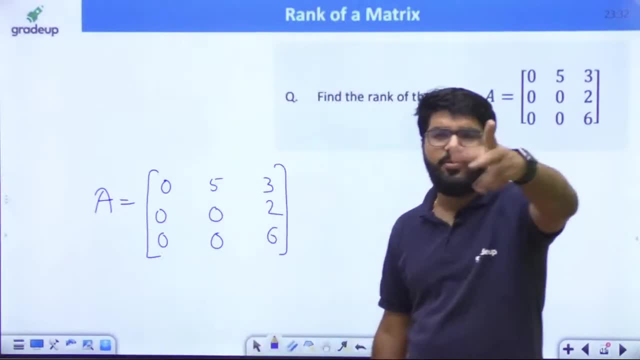 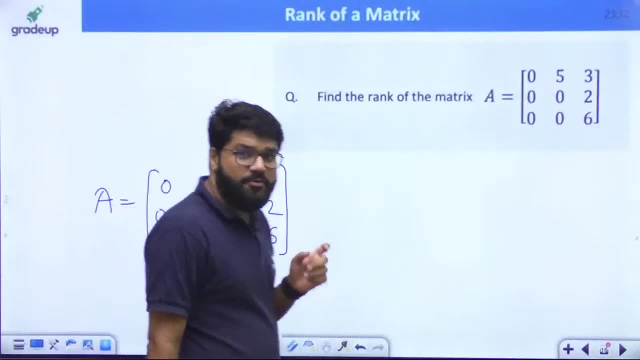 Confusion has come, Okay, Confusion. So you are getting the confusion. Some of you are telling 2.. Some of you 3.. So it is a fight. It is a fight between 2 and 3.. What is the correct answer, guys? 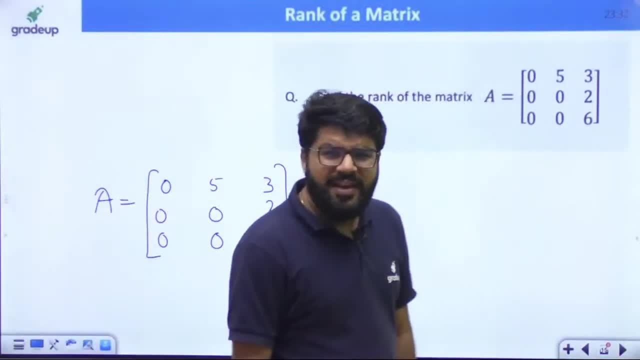 What is the correct answer and how many likes I see. Okay, Are you tired? 11.32, are we tired? I need to see the joy and let us see, No, the rank, What you are able to see. Okay, 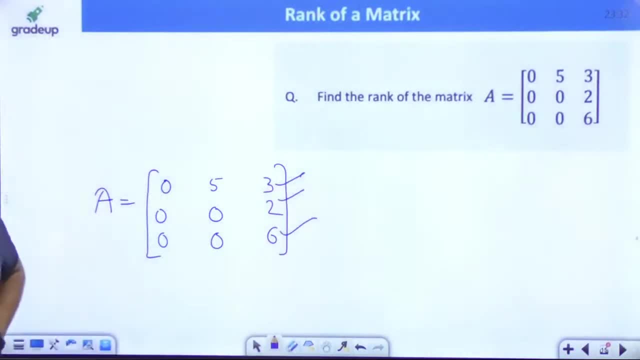 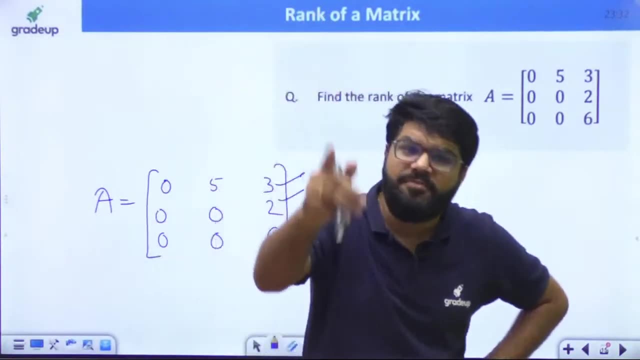 Rank is equal to number of non-zero rows. Maybe you are able to say That is why you are telling the rank is 3.. But rank is equal to number of non-zero rows if the matrix is in echelon form. If the matrix is in the echelon form. 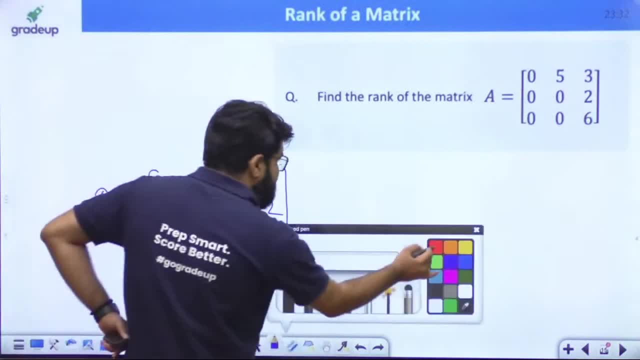 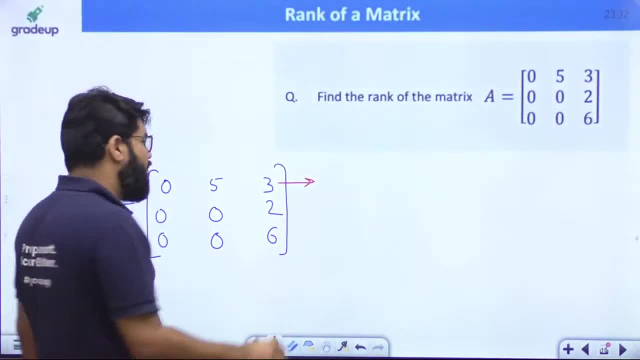 Is it actually following the echelon form? Is it actually following the echelon form? Right, Right, Yes, this method will also apply on 3 cross 4.. I will tell you. I will take the question of 3 cross 4 also. 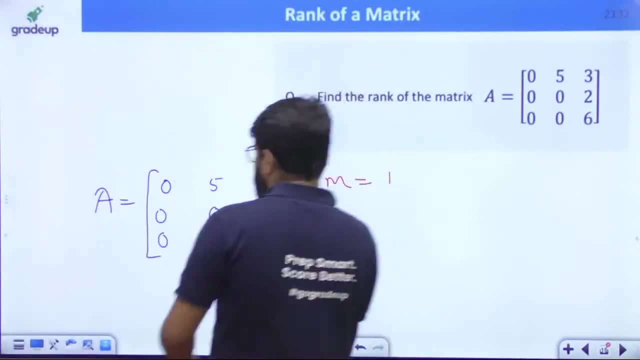 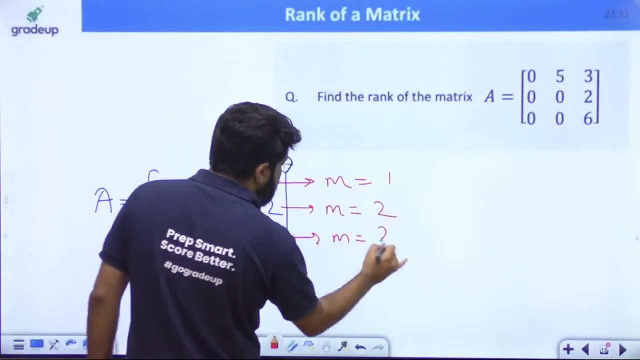 Don't worry How many m starting zeros: 1. Look, 1 starting 0.. 2 starting 0.. 2 starting 0.. m is equal to 2.. Then m is equal to 2.. Is it following the increasing order? 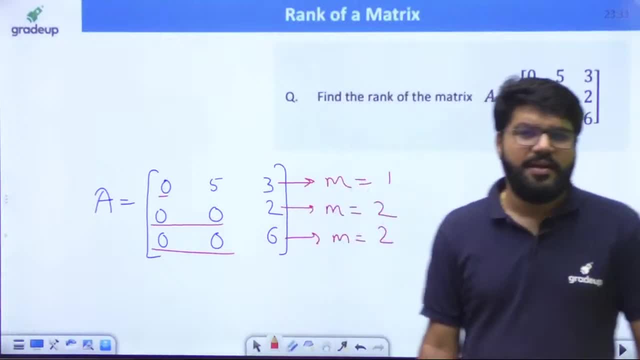 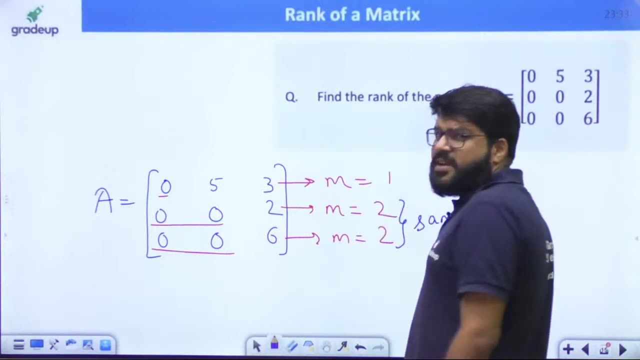 Okay, Is it following the increasing order? Everybody try, Try to understand. Is it following the increasing order? This is same. Increasing means strictly increasing. Not even equal, Not even same. Not even same. Okay, 1., 2.. 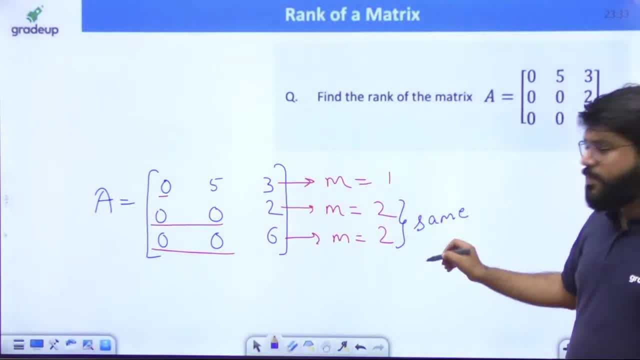 2.. 2 or 3 should be there, Or 2 or 4.. It should be increasing, Okay, But it should not be same. So this is not. If this is same, Then this matrix is not in the echelon form. 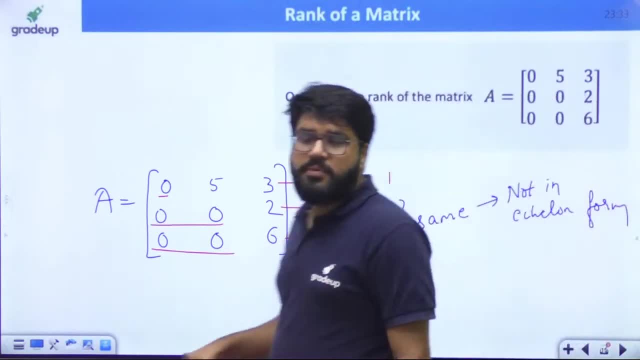 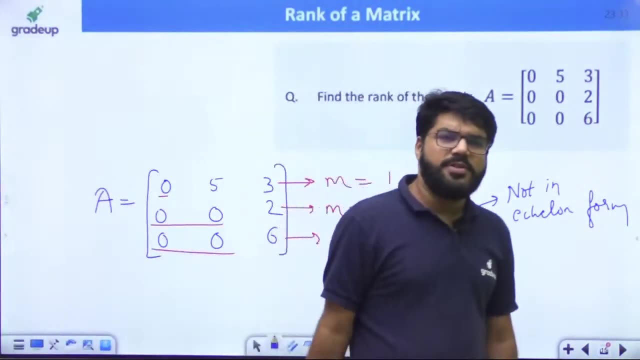 This is not in the echelon form. That is why Many of the answers were wrong. It is not in the echelon form. This is the problem. And then you are telling rank equal to number of non-zero rows. That is not applicable. 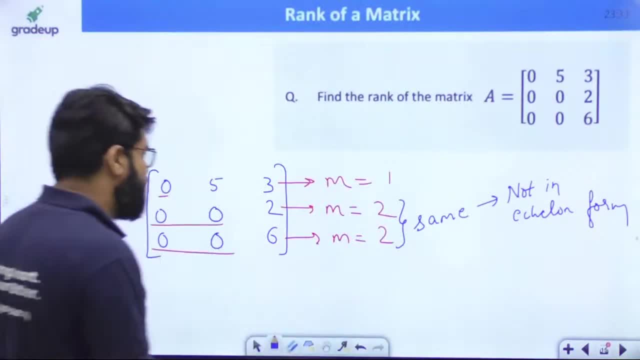 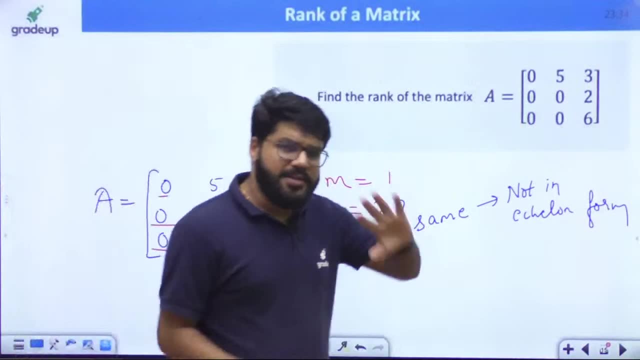 Because it is not the echelon form. It is not the echelon form, Everybody. Okay, So can I. Then how can I solve the question, sir? Then how can I solve the question? I will tell you. I will tell you more shortcuts. 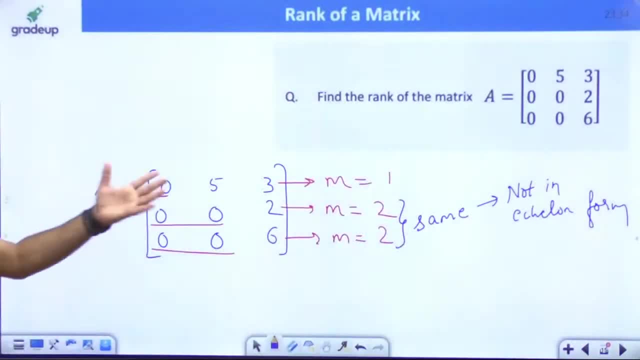 Okay, We will wait a little. We will take it to a little more shortcut. Okay, I think this is the third or fourth question only. So, if it is not in the echelon form, Can we convert it into the echelon form? 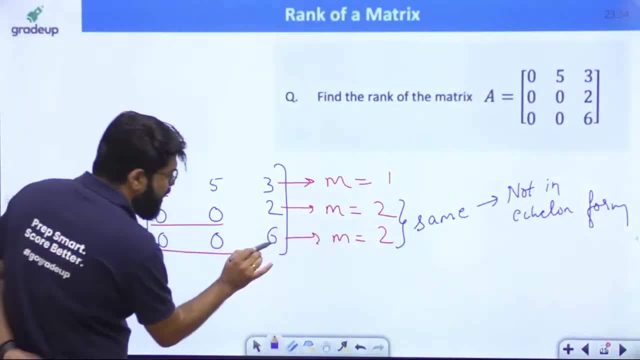 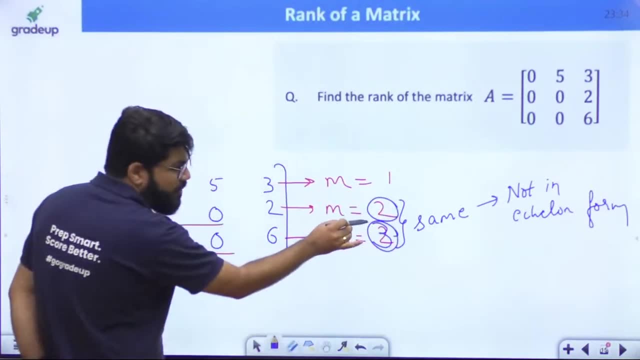 Let's try to understand. Can we convert it into the echelon form? Look If How it is converted into echelon form. There are two zeros here. If I make the three zeros here, If I make the three zeros, Then it will become the increasing order. 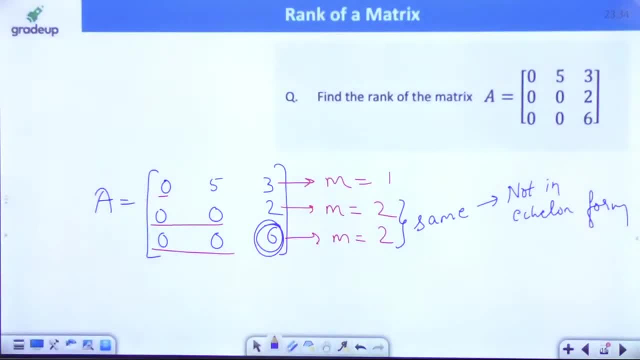 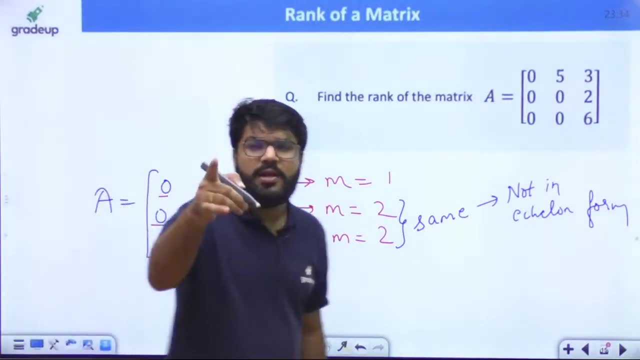 Yes, sir, How to make it three zeros. Let's convert this number into zero. Let us convert this number into zero. And how to convert this number into zero. This is the In the row three. I will use the row transformation. 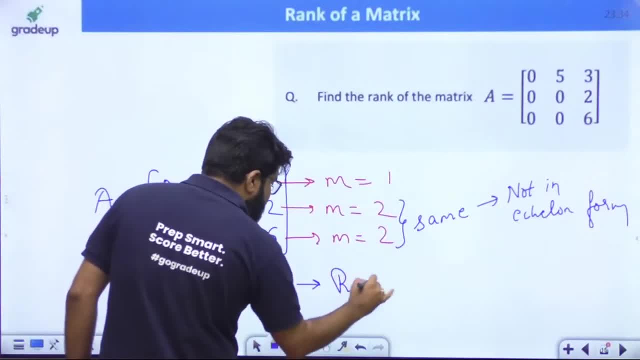 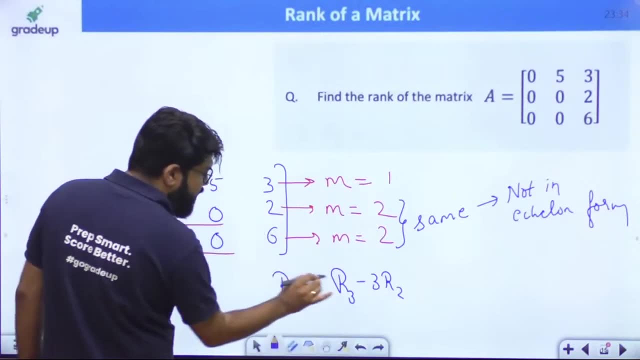 Elementary row transformation. This is R3.. Write down R3 as R3 minus 3R2.. Okay, Okay, 3 into 2 will become 6.. 6 minus 6 will be 0.. So R3 is R3 minus 3R2.. 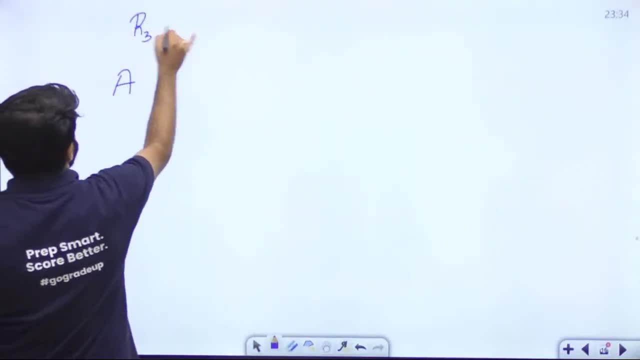 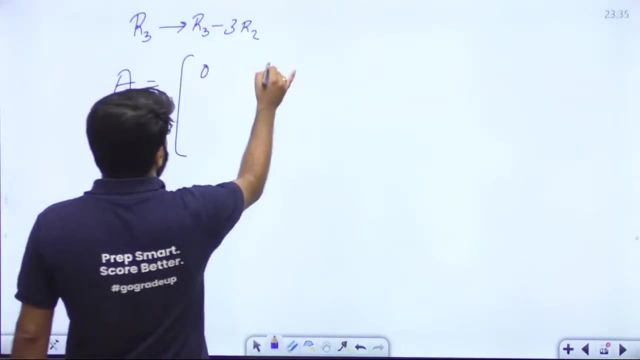 Let us do this transformation. Okay, Let us do the transformation: R3 equal to R3 minus 3R2.. After doing this, The matrix A will become 053.. Sir, it becomes 053.. Then 002.. 002.. 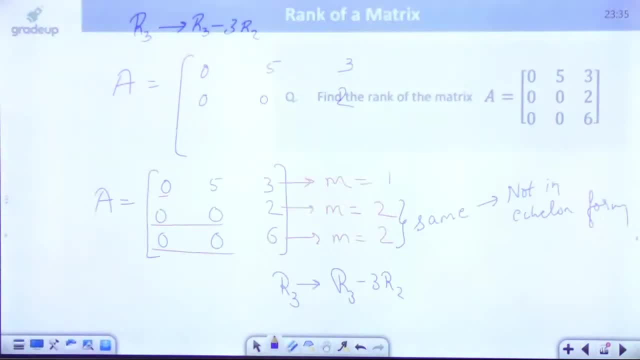 There is no change on the row 2.. R3 should be replaced Right. Okay, 0 minus 0.. 0 minus 0.. 6 minus 3.. 2's are 0.. So this is 0.. 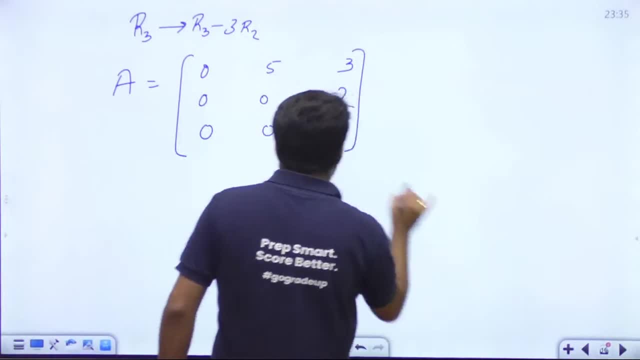 0 minus 0.. 0 minus 0.. This is 0.. This is 0.. Now have a look at this, guys. First of all, This is what. This is what is the ROZ. Now the matrix has ROZ. 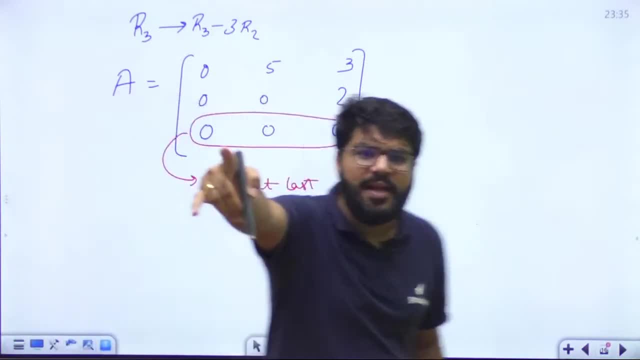 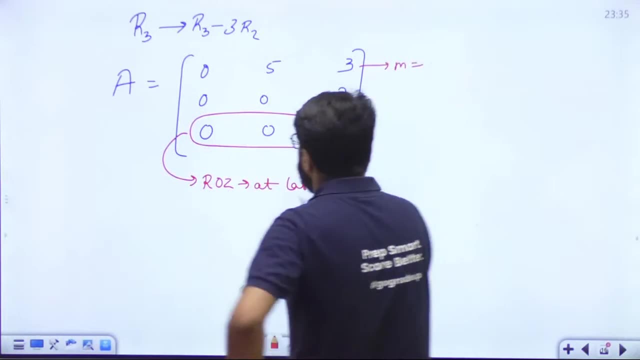 But that ROZ at the last, That row of 0 is at the last, Very good, This row of 0 is at the last. Then what is the number of starting 0's, Sir 1.. 1, 0.. 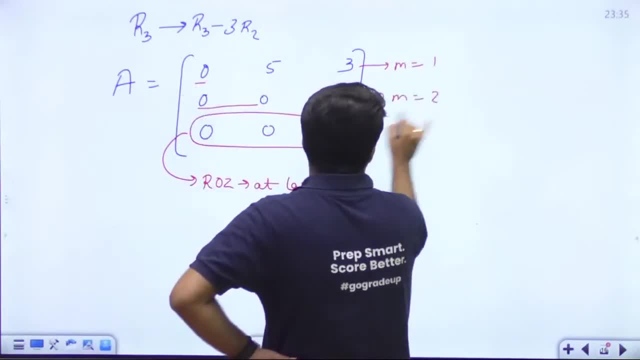 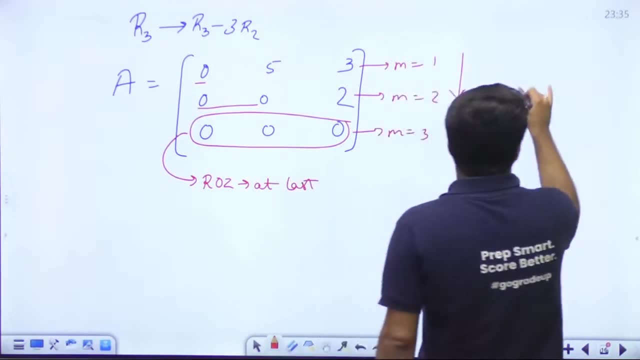 2, 0.. And 3: 0's M is 1.. M is 2. M equal to 3.. So how much it is Increasing or decreasing, How much it is, It is there in the increasing order. 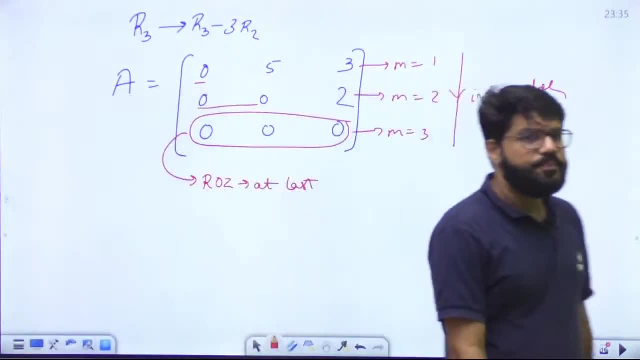 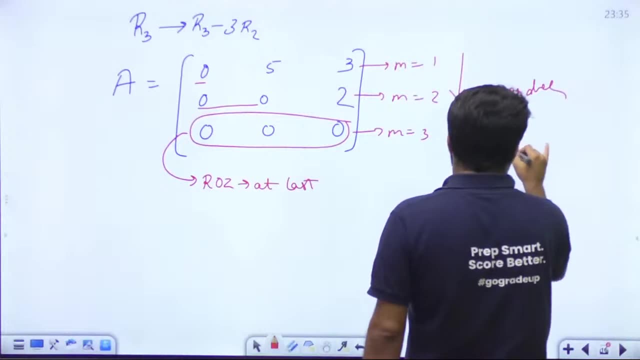 Right, It is there in the increasing order form. Right, It is there in the increasing order. And if the number of row of 0 in increasing Number of starting 0, increasing order. So yes, this is echelon form. Yes, this is known as the echelon form. 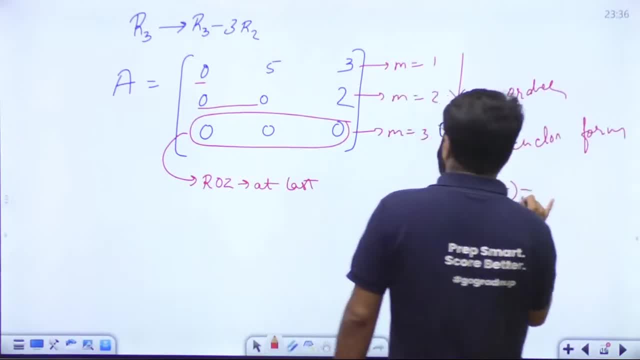 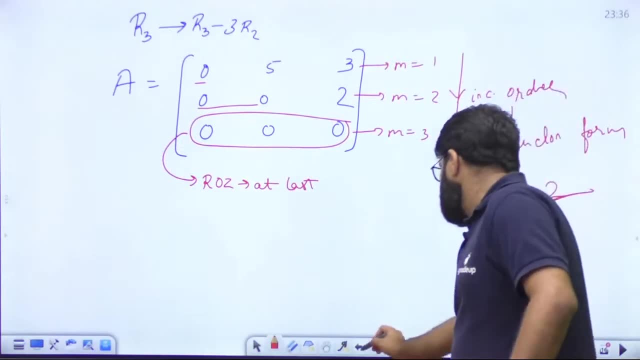 Okay, And if a matrix is in echelon form, What is the rank of matrix? Number of non-zero rows: 1 non-zero row. Second non-zero row. Third: non-zero row. So how many non-zero rows? Answer is 2.. 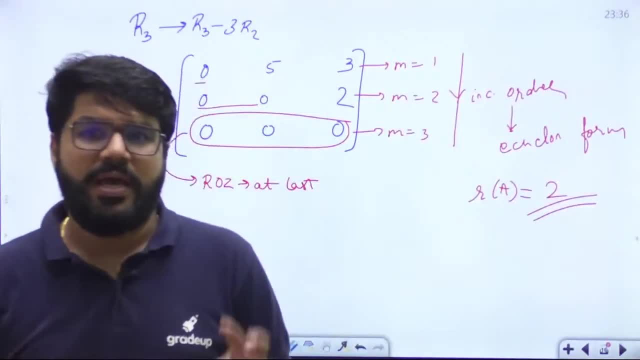 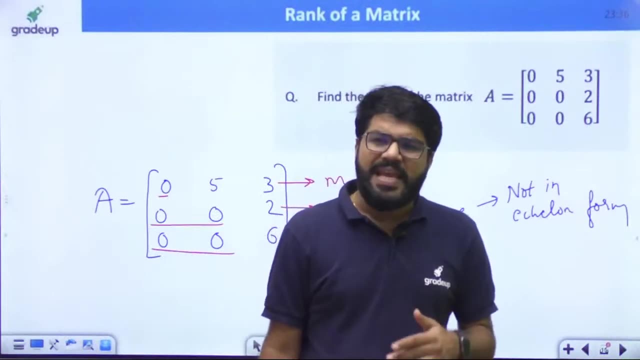 Answer is known as 2.. Correct Answer is known as 2.. Everybody Answer is known as 2.. So if it is not in the echelon, I have converted it to echelon. Okay, Sometimes echelon can be time consuming. 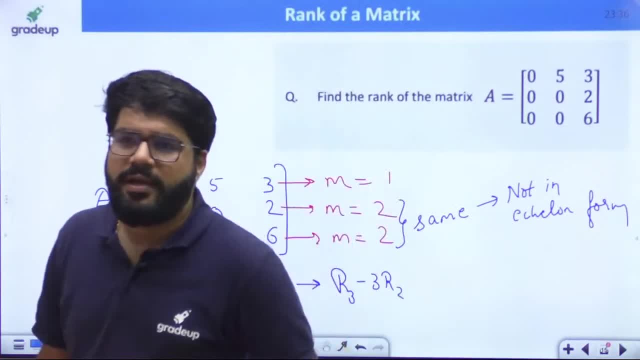 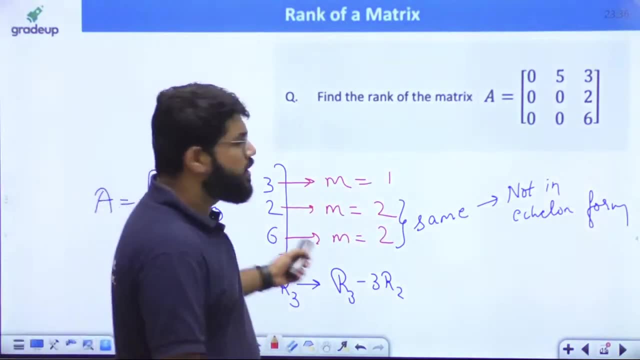 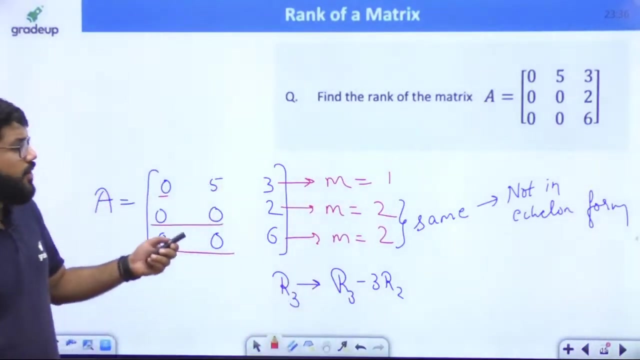 So I will tell you other tricks also. I will tell you other methods also. Right, Right, Okay, Okay, Okay, Okay, Come on PK once, Just Come in once, Okay, Once, Not more than once. I am able to read it. 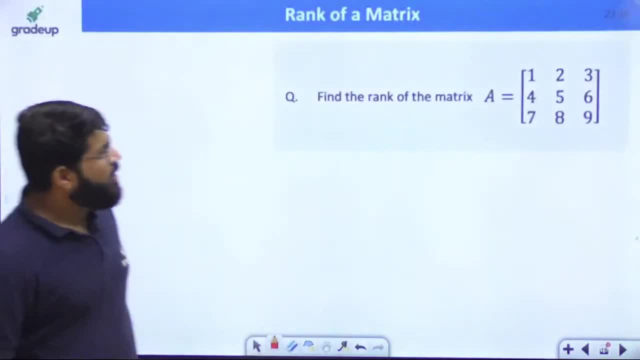 Don't worry, Let's go to the next question. Let's go to the next question. Find the rank of the matrix: 1,, 2,, 3,, 4,, 5, 6,, 7,, 8,, 9.. 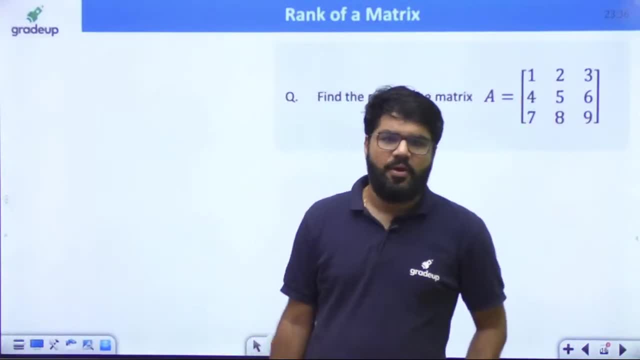 Now let's again take it with echelon form, And there is something new that we will add now. We will add something new after this. Let's add something new after this: Right: 1,, 2,, 3,, 4,, 5,, 6,, 7,, 8,, 9.. 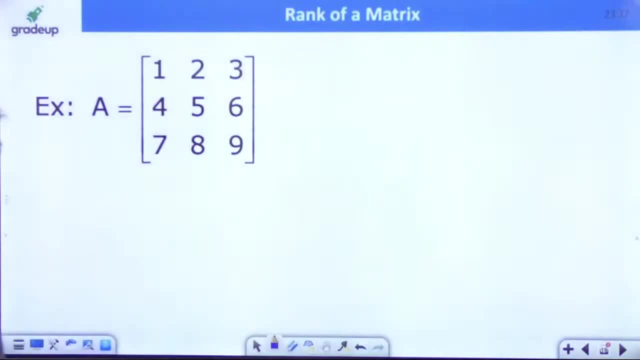 Now, first of all, let us try to understand this: 1,, 2,, 3,, 4,, 5,, 6,, 7,, 8, 9.. 1, 2,, 3,, 4,, 5,, 6,, 7,, 8,, 9.. 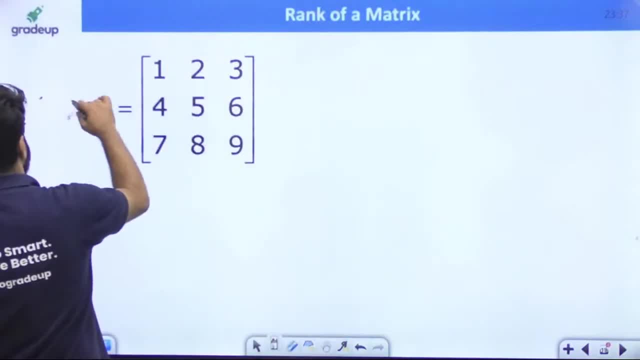 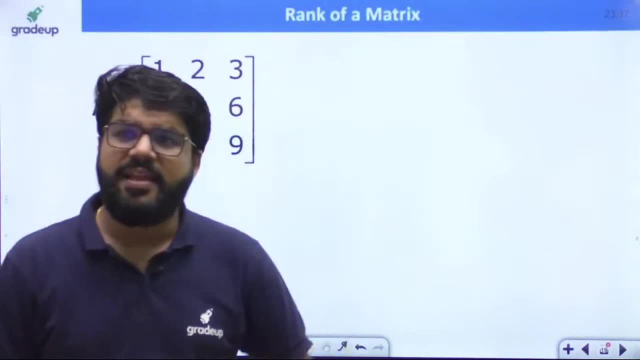 The same matrix has been copied here. Okay, 1,, 2,, 3,, 4,, 5,, 6,, 7,, 8,, 9.. Is there any row of 0?? Sir, there is no row of 0.. 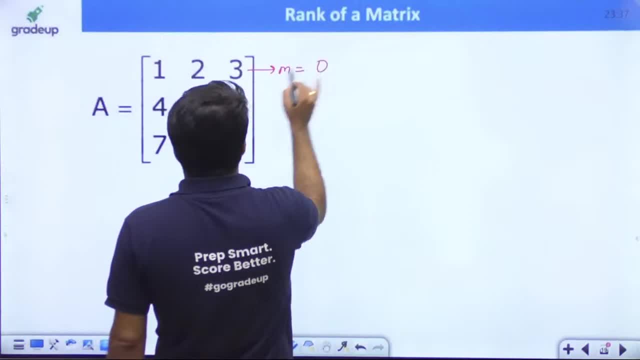 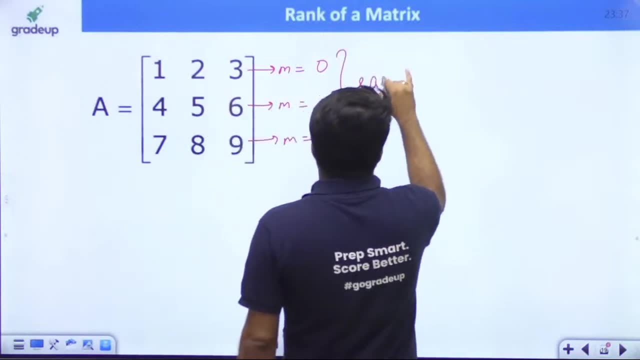 Sir, there is no row of 0.. But what about starting 0s, Sir? there is no starting 0.. Second row: No starting 0.. Third row: There is no starting 0.. All same, Okay, All same. 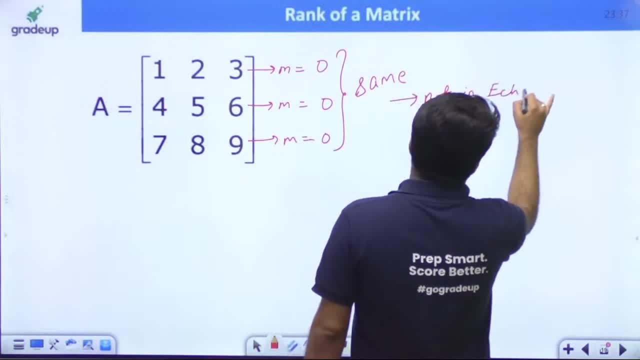 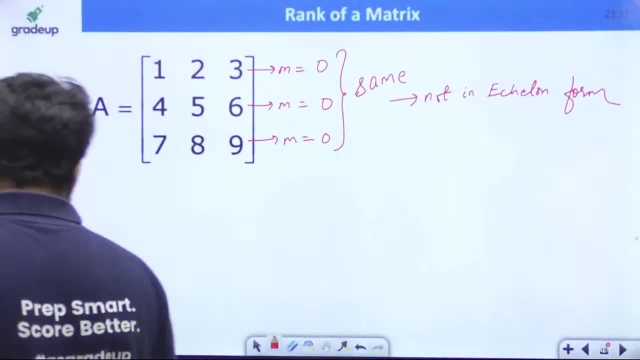 This is clearly not in the echelon form. This is clearly not in the echelon form. This is clearly not in the echelon form. Right, This is clearly not in the echelon form. Can I convert it into echelon, Try karte. 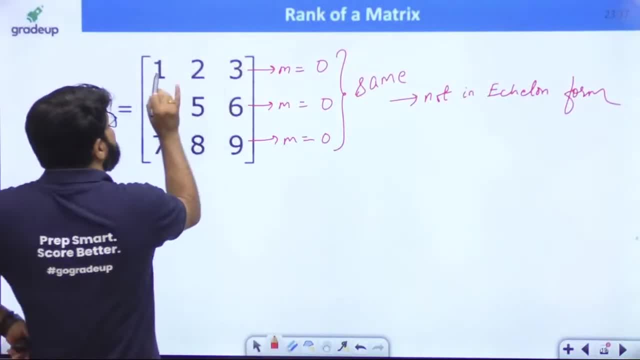 Try karte. Can I convert into echelon? So see, Echelon means, if this is, Look what you have to do, How many starting 0s- 0.. So next row there should be 1 starting 0.. 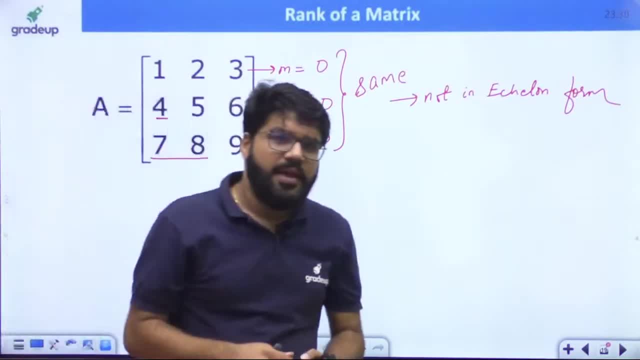 And next row there should be 2 starting 0.. To make it increasing, Next row, at least 1 starting 0.. And then for the next row, at least 2 starting 0.. 2 or 3.. However you are able to get. 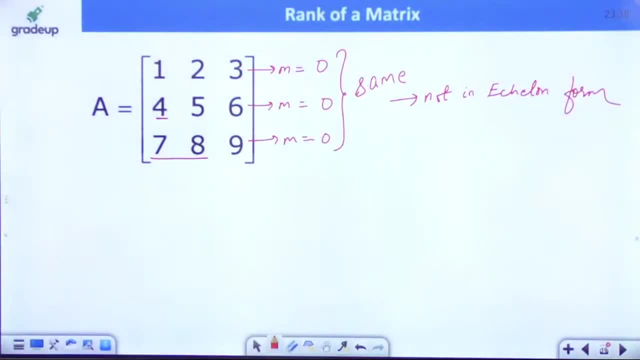 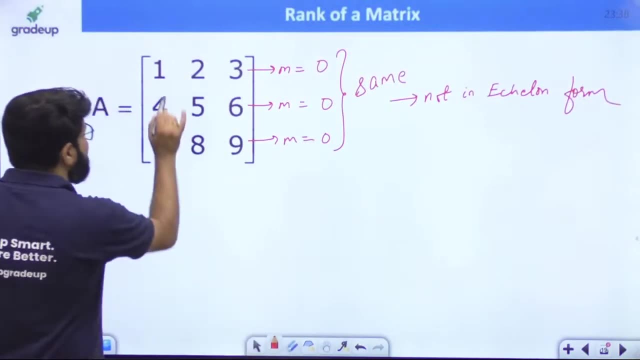 2 or 3.. But it should follow an increasing pattern. It should follow some increasing pattern. So what we are going to do now, Let's try to first convert. Okay, Let's try to first convert the elements of the first column. 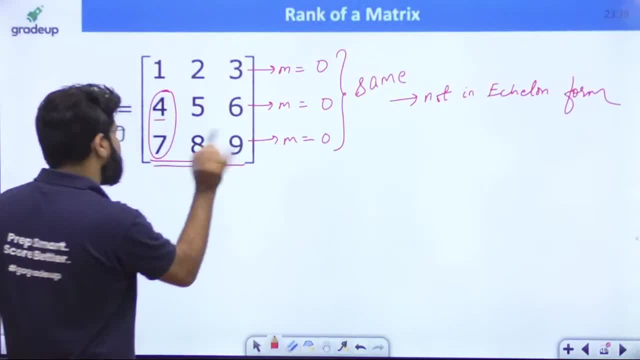 Okay, We need this And we need these 2 or these 3.. 2 or 3. That I don't know, Whatever comes, But let's try to start with the first column, So how you can convert 4?. 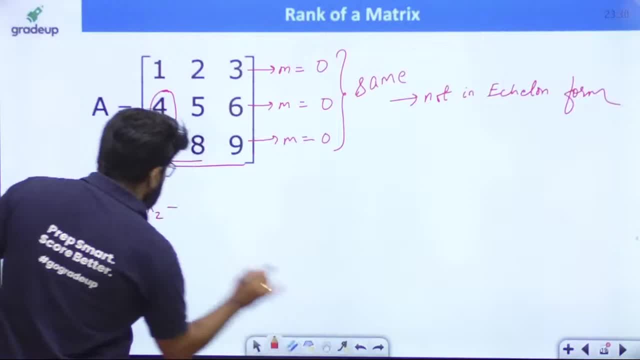 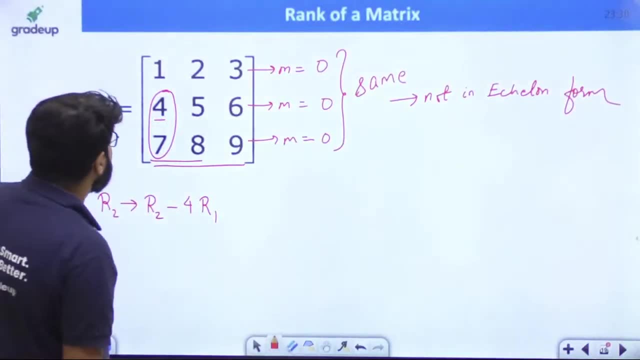 4. 4 minus 4. 4 into 1.. 4 minus 4 into 1. R2 minus 4 R1.. R2 minus 4 R1 should be R2.. Right R2 minus 4 R1 should be R2.. 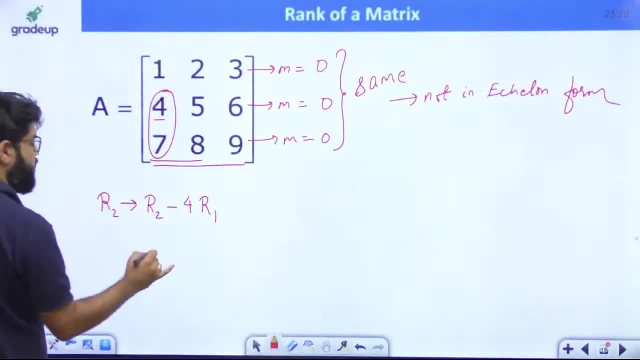 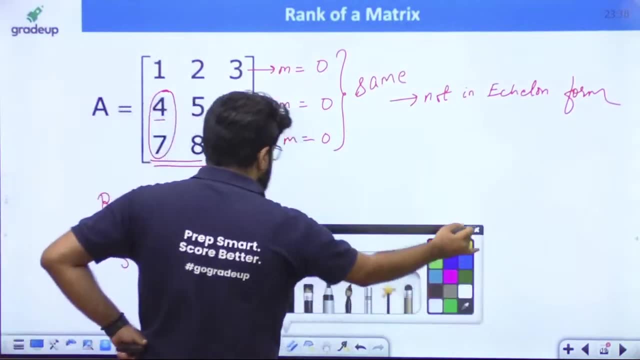 Then how do you convert 7 into 0? Using the first 7 minus 7 into 1.. That is R3 minus 7 times R1.. R3 equal to the R3 minus 7 times R1.. So let us do this. 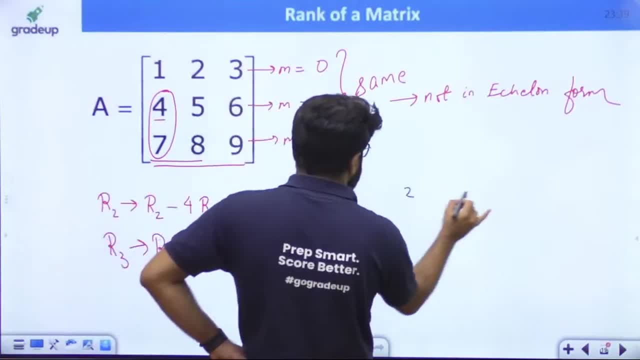 And let's see what is the matrix left. R1 is unchanged. This is 1, 2, 3.. 4 minus 4 into 1 is 0.. 5 minus 2.. 4 into 4 minus 3.. 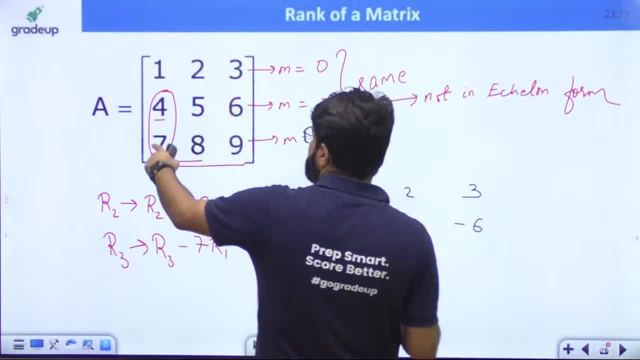 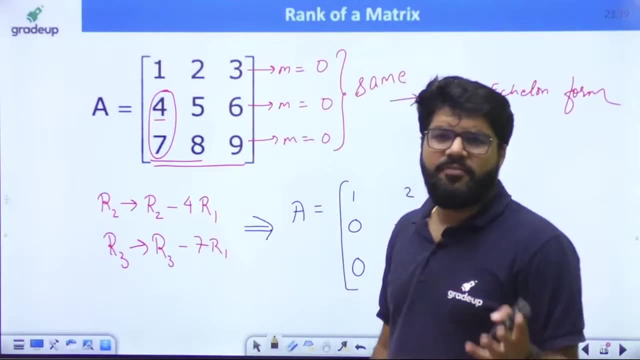 6 minus 4 into 3 minus 6.. 6 minus 12 is 0.. 7 minus 7 into 1.. R3 minus 7 R1.. Next step: R3 minus 7 R1.. Right, It can be different for column. 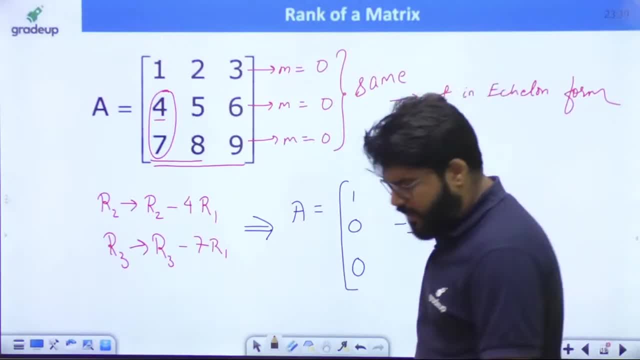 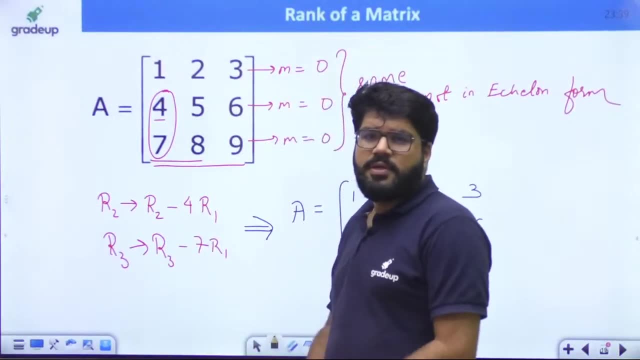 Column is also there, but we usually follow row echelon matrix. But there can be column echelon matrix also. Same rules. you have to reverse for the column Right. Right, Look, Ashok, It is helpful for some question. I clearly told you it is lengthy for some question. 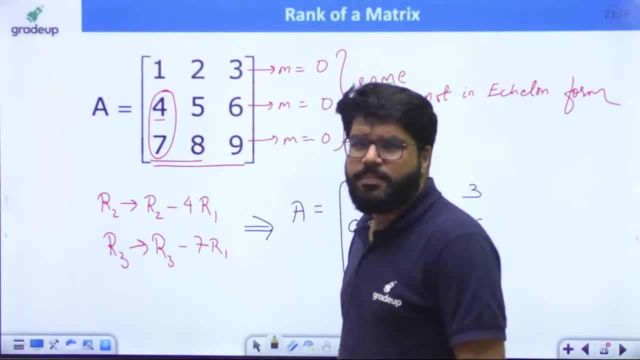 But I will tell you other methods also. Just be patient, Ashok. Okay, Just be patient, Okay, Ashok. you only come to teach independent rows and columns. I am telling you, I will tell you all the methods, Ashok ji. 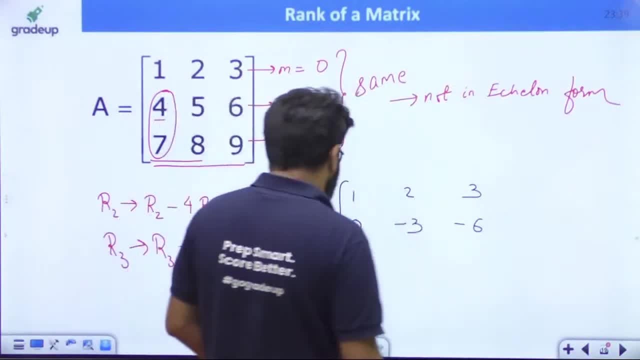 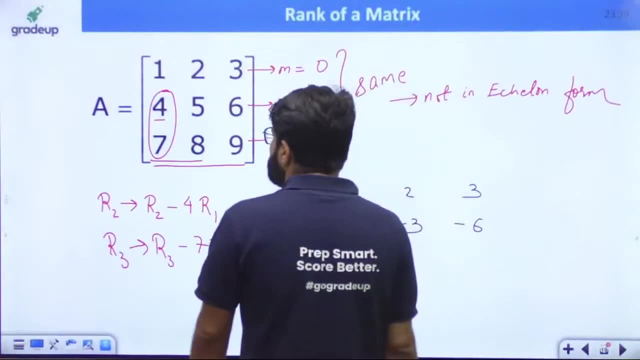 Do one thing: you come here and show up and then you come and teach here. Okay, Some methods: dependency, independency will not help you. Some questions: row echelon will help you, So kindly keep the patience, Okay. So now 7 minus 7 into 1 is 0.. 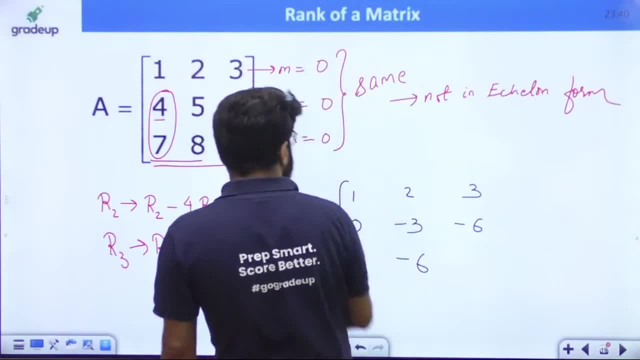 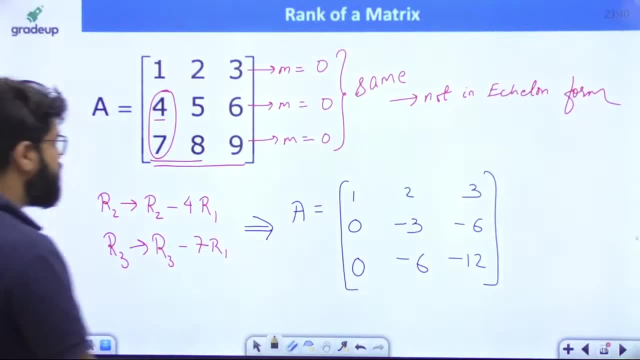 5 minus 2 into 7 is minus 6.. 9 minus 3 into 7 is 9 minus 21.. That is the minus 12.. That is the minus 12.. Okay, Is it okay? Now what is the number of starting zeros? 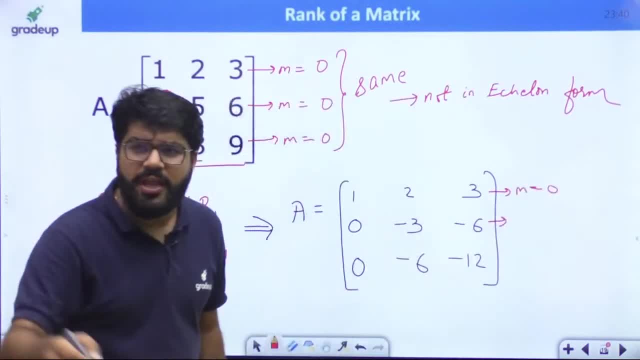 Sir, here it is 0.. Okay, don't write every time, I am just writing for your explanation. Okay, this is 0.. Then this is m equal to 1.. 1 starting 0, but again 1 starting 0.. 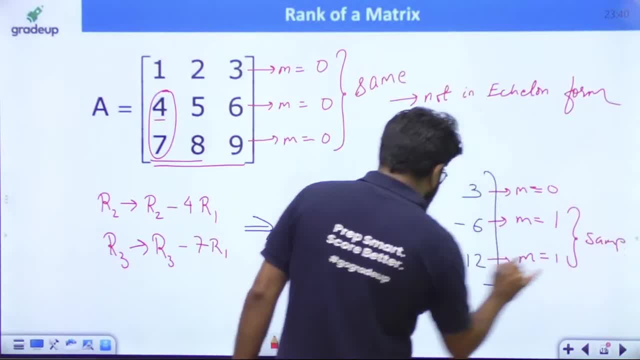 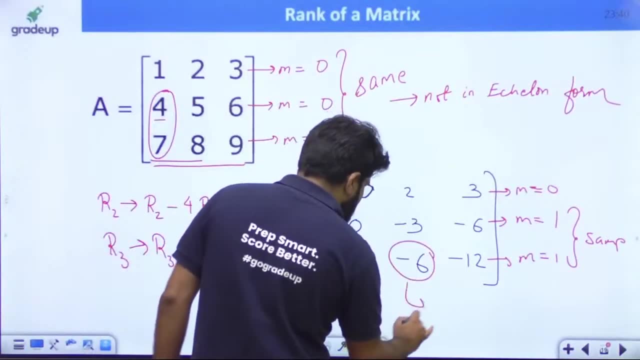 Sir, this is again same, same, same Same is not required. So what is the only thing? Let us try to convert this also into 0.. Okay, let us try to convert this also into 0.. So what I will do now? 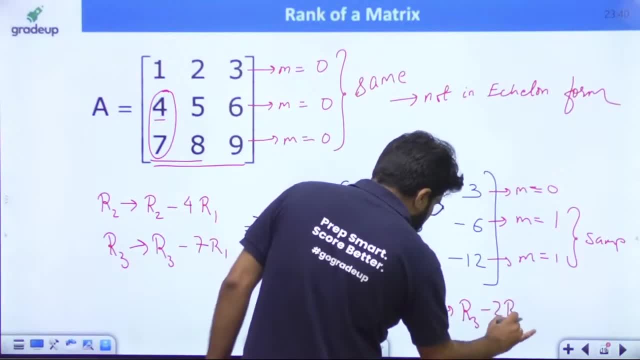 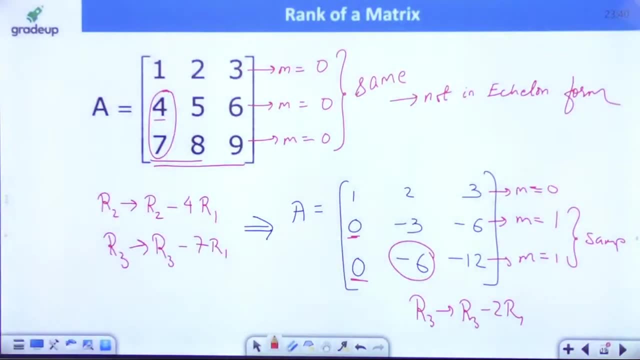 I will write down R3 as R3 minus 2 R1.. 2 into minus 3 is minus 6.. It will be same Minus 6 minus minus 6 will be 0.. Right, Okay, R3 minus 2 R2.. 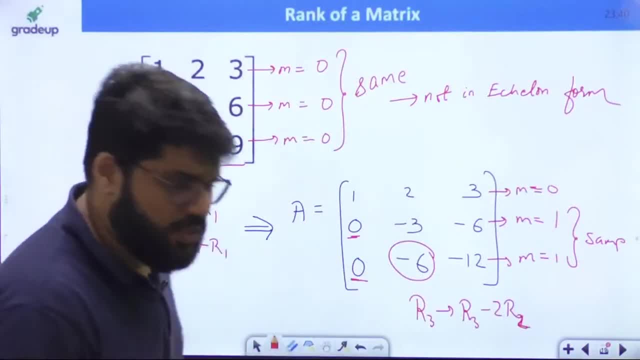 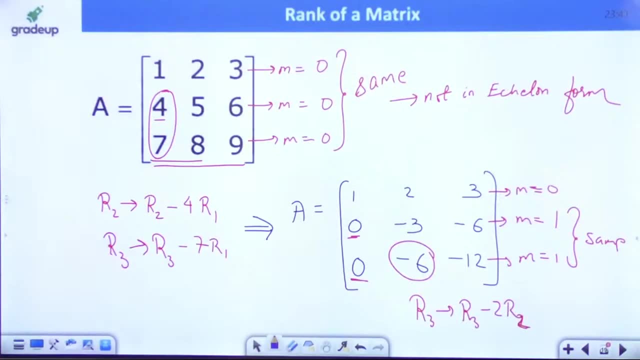 Sorry, 2 R2.. Right, No, no issues, Ashok, That is what I am just going to come up to. the method also, All methods: Determinant echelon method, determinant method and the dependency method. So come on. 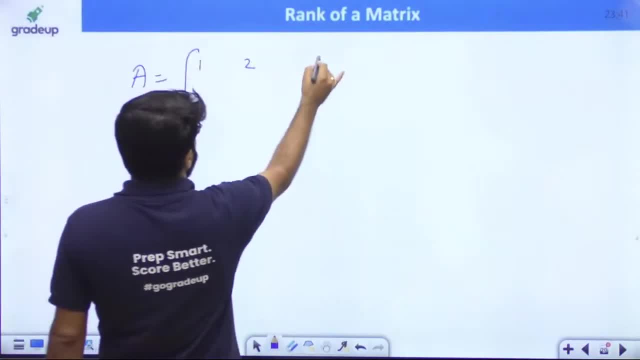 How much is the matrix after this, Sir? it is 1, 2, 3.. 1, 2, 3.. Next, 0 minus 3.. 1, 2, 3. Minus 6.. 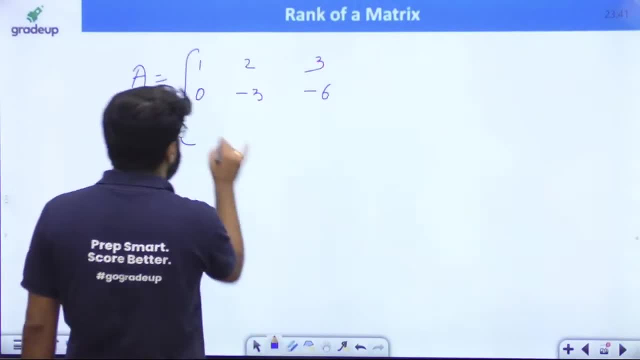 0 minus 3.. Minus 6. 0.. Then R3 minus 2, R2.. 0 minus 0 is 1.. Okay, Minus 6.. Minus minus 6. 0.. Minus 12.. 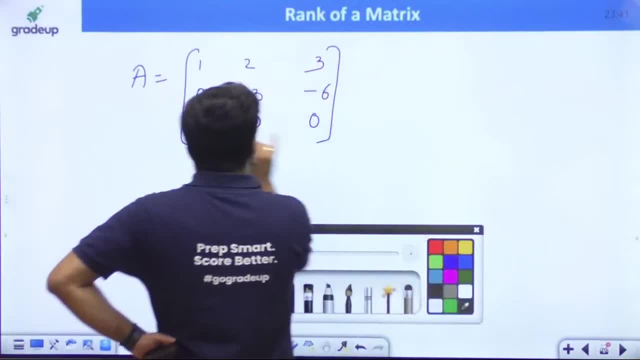 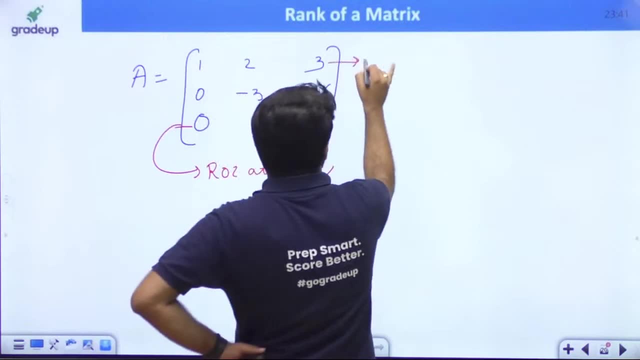 Minus Again, minus 12.. So this is 0.. Complete row of 0 obtained. Sir, there is a row of 0 also, No issues, But that is at last. So I am happy. Row of 0 at last. 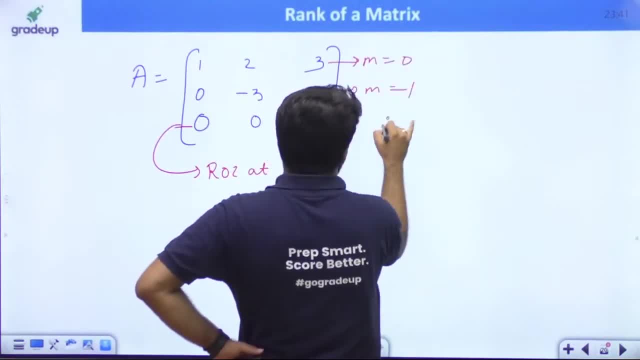 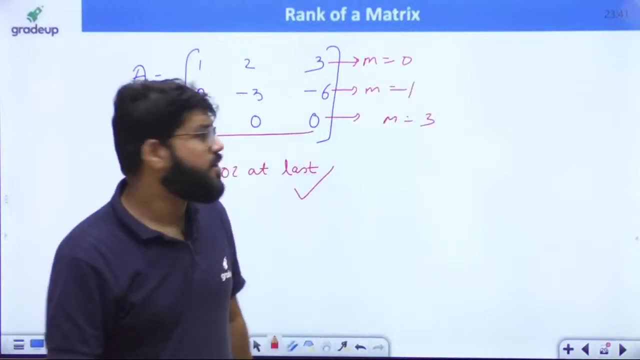 Number of starting 0 is nil. Number of starting 0, 1.. Number of starting 0,: 3.. But it is Whether it is 1,, 2, 3.. But it is in increasing order. Once a 3 together, it is in the increasing order. 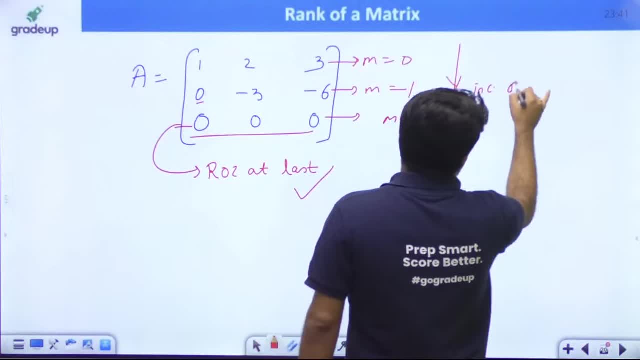 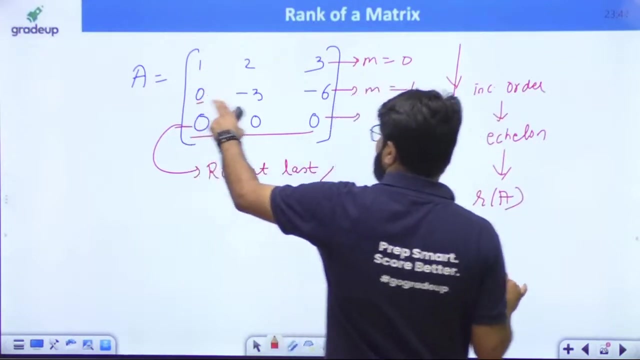 It is in the increasing order. So now it is in the Now it is what Increasing order. That means the matrix is in the echelon form, It is in the row echelon form. What is the rank of the matrix? 1, 2.. 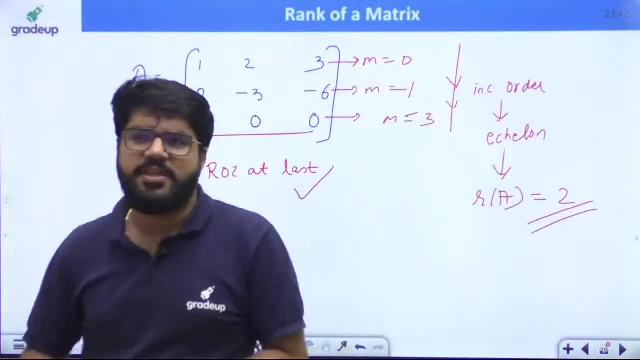 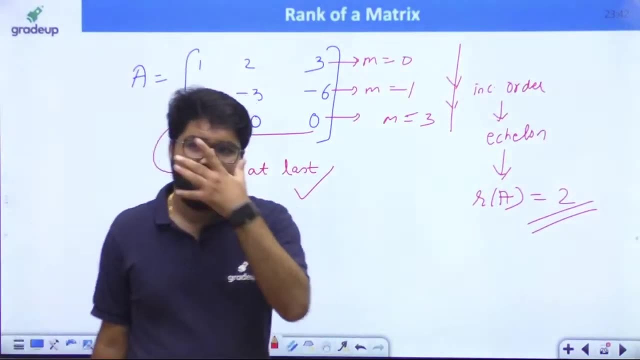 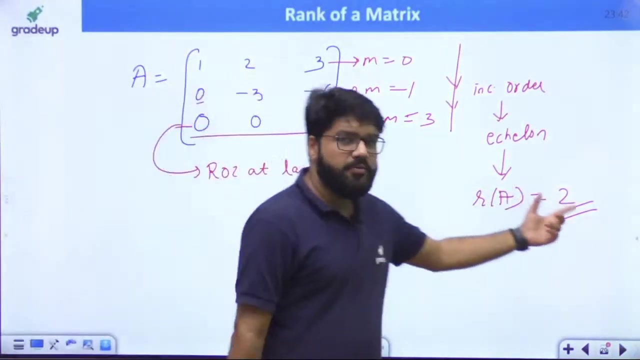 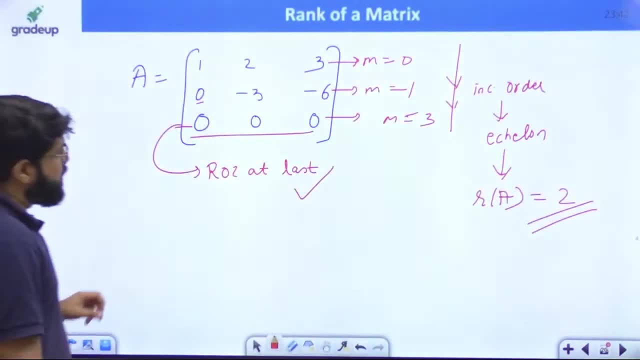 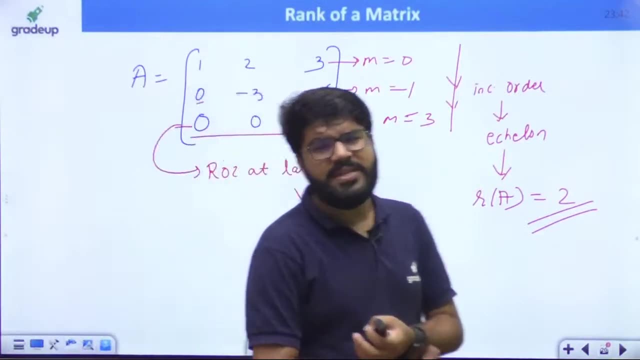 So it is 2.. Is it clear? Now going to the next. Now going to the next. Now let us observe some more points. Now let us go towards some different methods. I think row echelon method, because for some of the question it is just an observation. 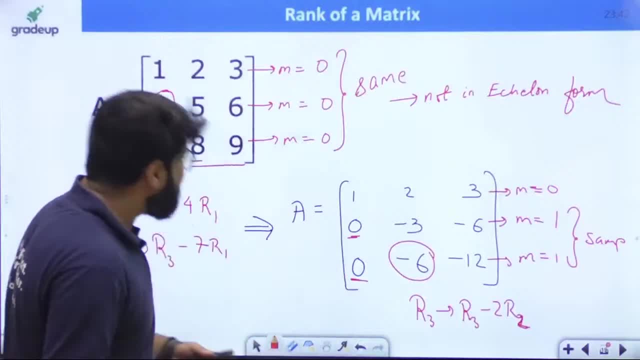 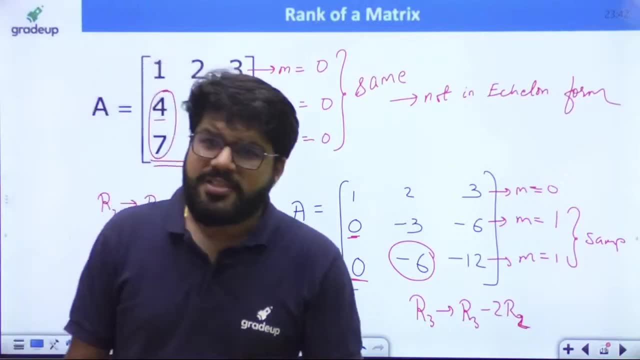 But where? What I am able to understand is that where I have to solve, Okay, Of course it is little bit time consuming, Okay, So can I do it without solving, Of course? if I am able to see by observation, then it is best. 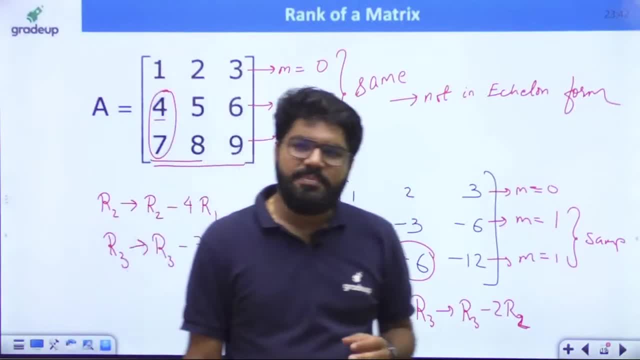 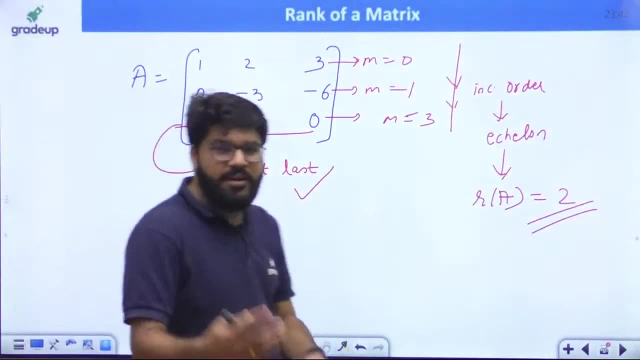 But if I need to solve, Okay, So can I skip this solution. Can I try something else? Yes, Let us try to solve something else now. Let us try to observe something else. Okay, Now, there are 2-3 different more methods. I will add. 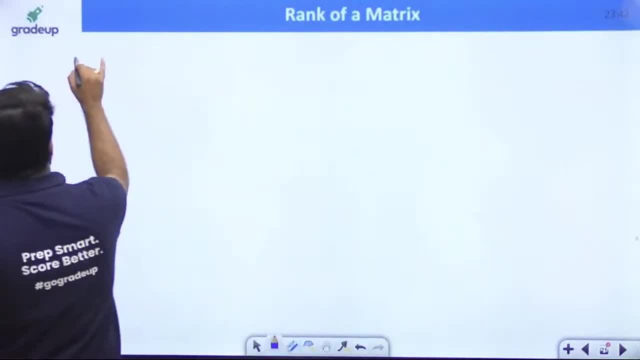 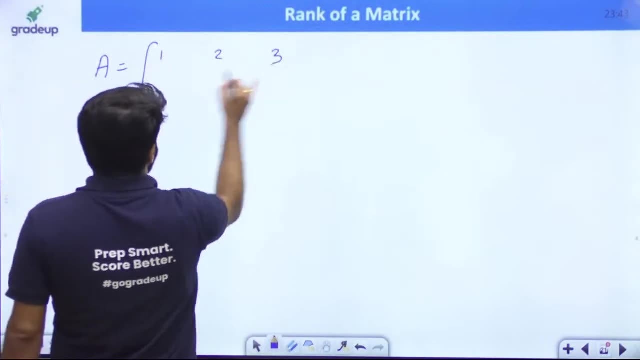 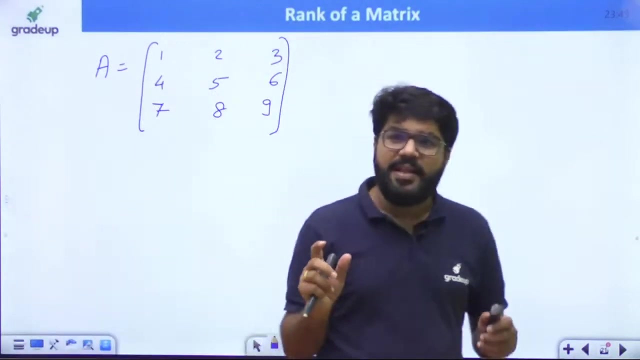 There are 2-3 different methods. I will add here. Pay attention. Okay, Same question. Same question: The matrix A: 1-2-3-4-5-6-7-8-9.. Okay, One is the basic definition method and next is the dependency method. 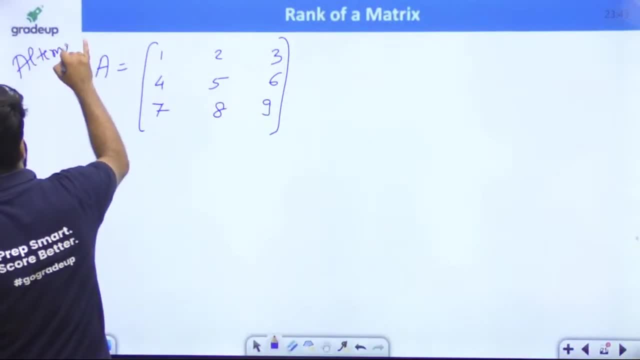 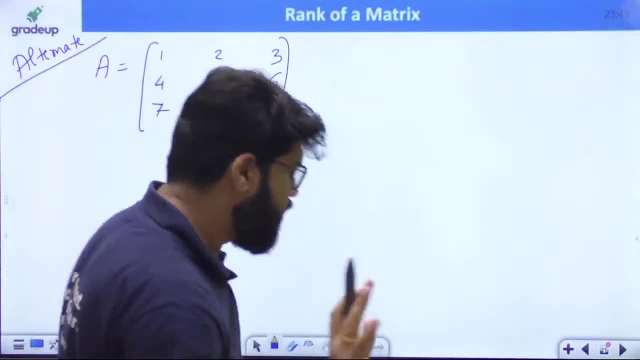 Okay, Now let us move towards alternate. We are going for the alternates now. We are now developing the alternates, And then we will take questions on alternate method. Just be concentrated now. Okay, You just have to concentrate here, Everybody. 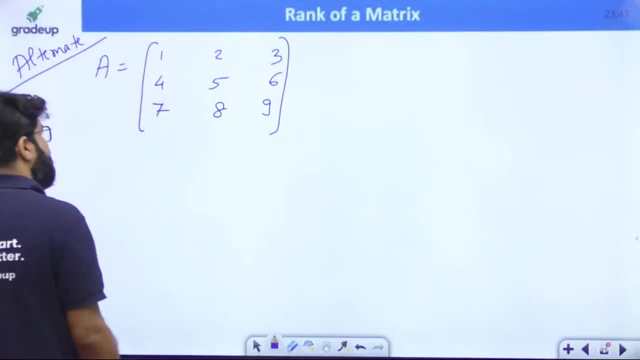 Right, Everybody. So see 1-2-3-4-5-6-7-8-9.. Okay, Before I tell you the alternate method, everybody try to recall. Recall what basically rank will be. Recall what is the one liner answer you can give for the rank? 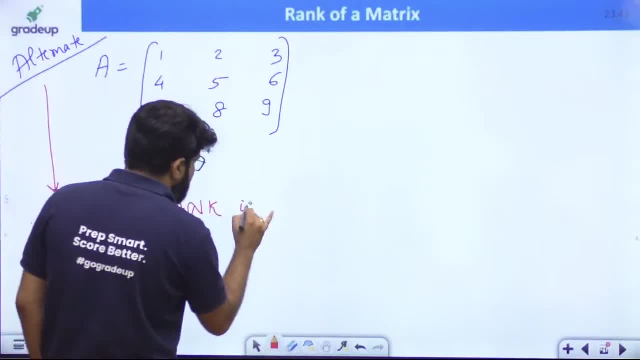 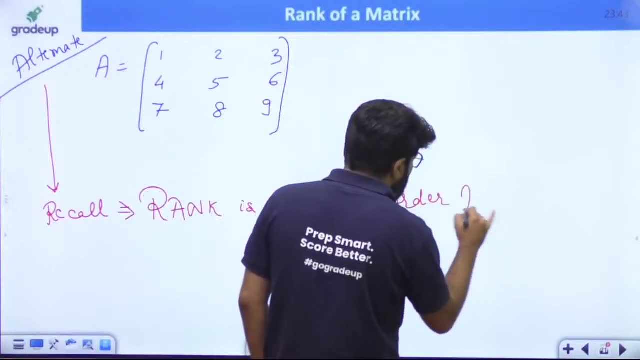 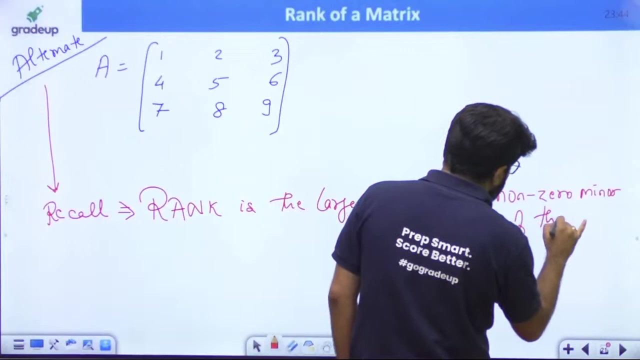 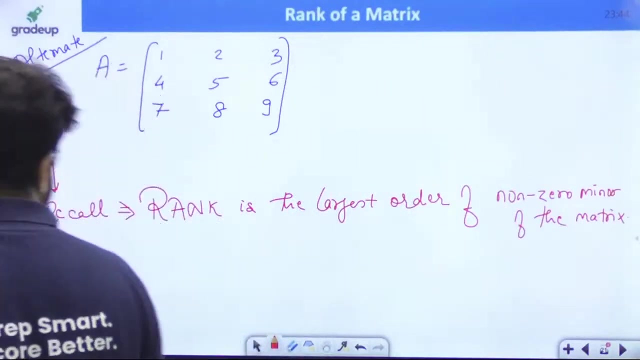 Recall that the rank is the largest order of non-zero minor of the matrix. Rank is the largest order of non-zero minor of the matrix. Just let us try to recall the basic liner about rank, Basic one liner about rank. Now, Now. 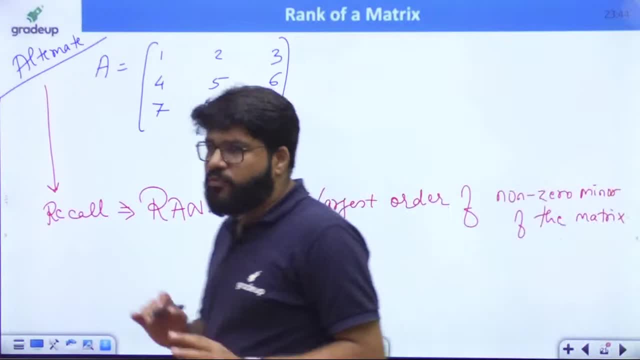 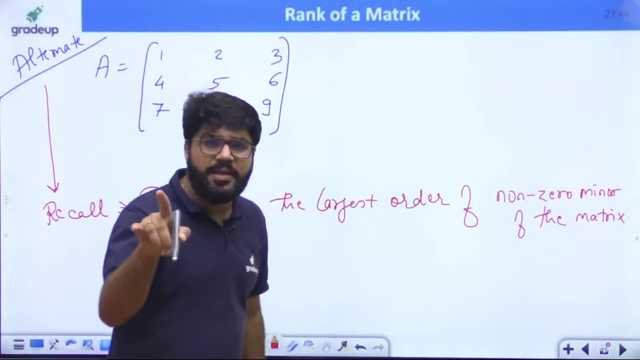 I will tell you a simpler method. Next will be even more simple, But let us try to follow the basics now. What does basics say? What does basics say That rank is the largest order of non-zero minor of the matrix. Okay, 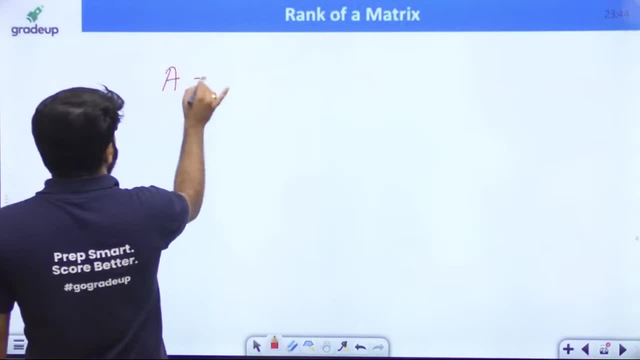 For this, For particular matrix here. Here the matrix A is 3 cross 3.. Here, the matrix A is 3 cross 3.. Okay, So what is the largest minor of 3 cross 3? Is it 0 or not? 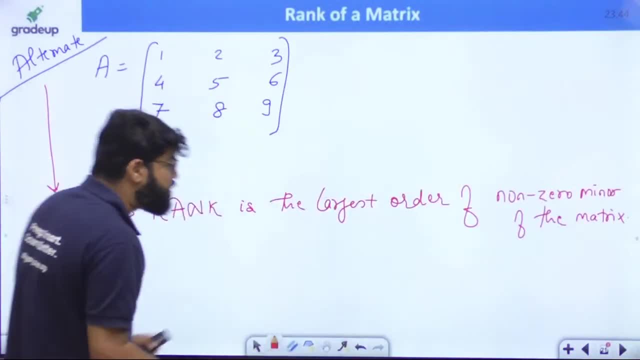 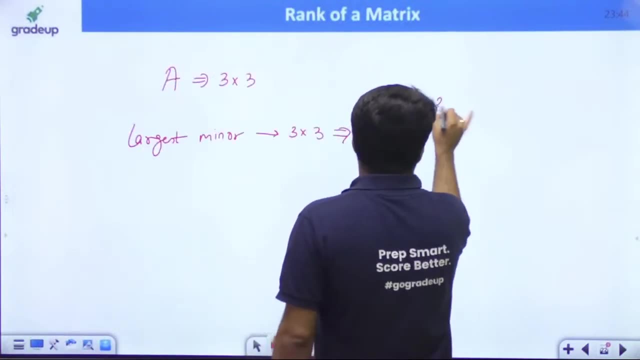 I am not talking about that. Rank is the largest order of non-zero minor. But first let us see what is the largest minor of 3 cross 3.. It is a 3 cross 3 minor only That is known as the determinant. 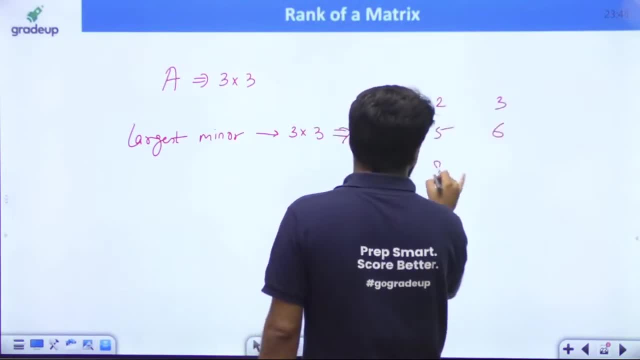 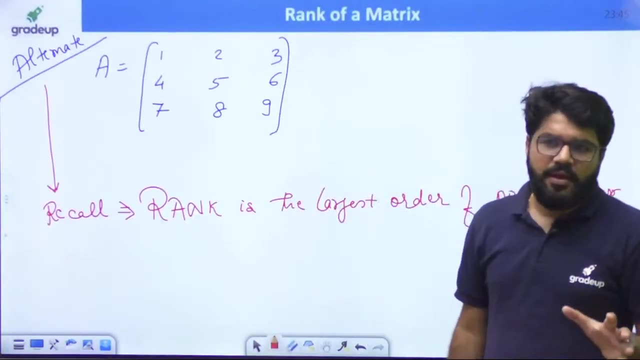 1-2-3-4-5-6-7-8-9.. Okay, Just to make you revise. Just to again make you revise. What is the general definition of minor By combining square or non-square matrix? What is the general definition of minor? 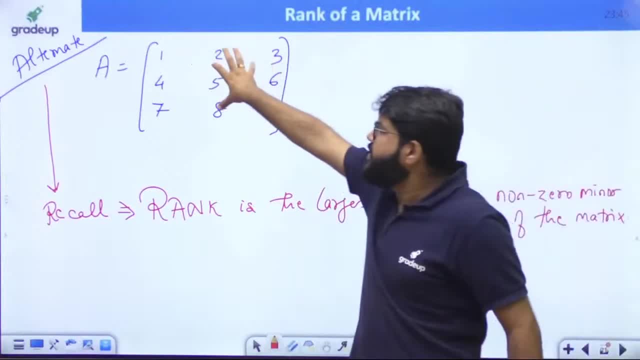 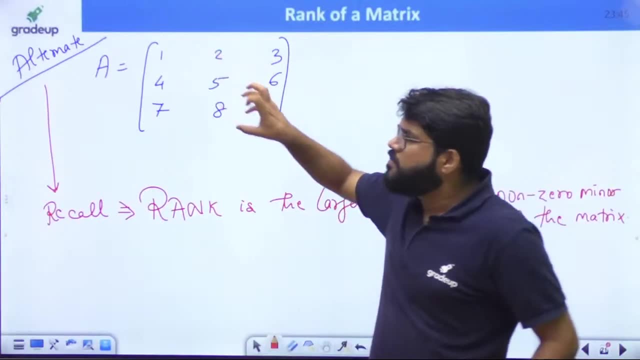 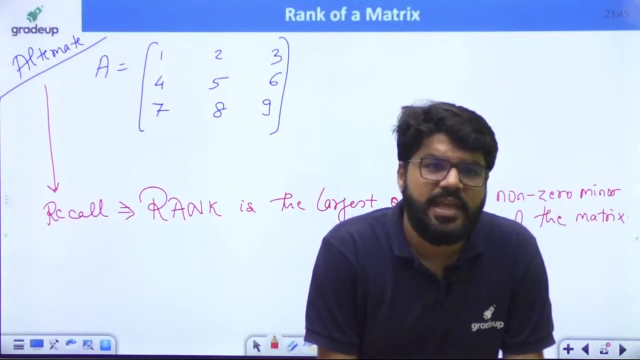 Minor is any determinant. Minor is any determinant which can be extracted from the matrix. Okay, Any determinant which can be extracted from the matrix, Which you can extract from the matrix, Every determinant will be minor. Any determinant which can be extracted from the matrix. 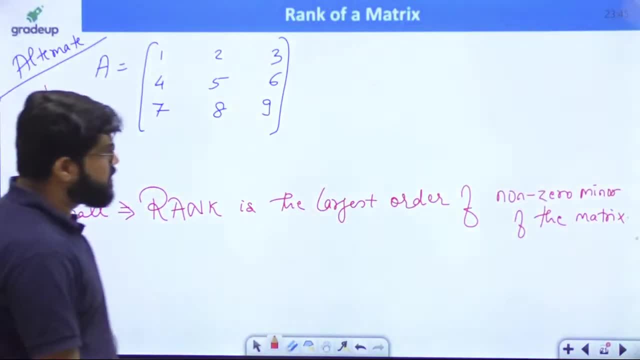 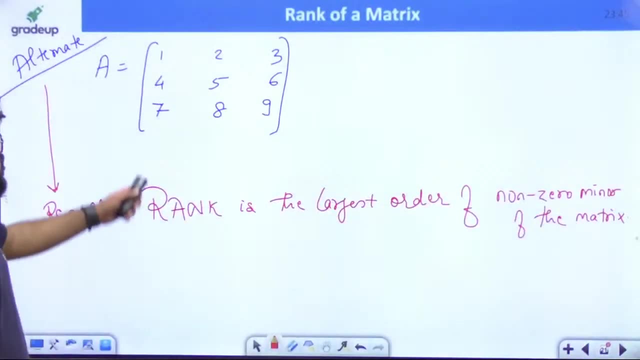 Is known as the minor of the matrix Right, Is known as the minor of the matrix Got. it Is known as the minor of the matrix Right. So what is the largest possible determinant? Take the complete determinant 1-2-3-4-5-6-7-8-9.. 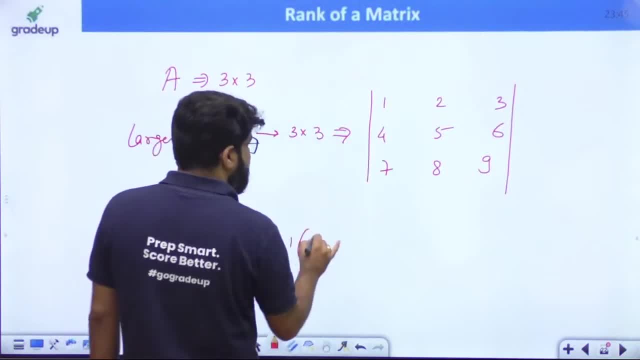 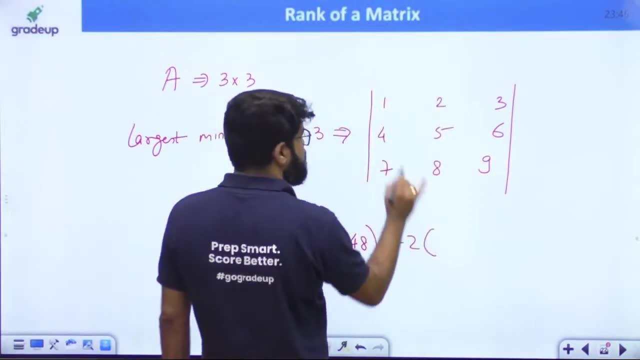 Okay, Let us try to calculate this determinant. Okay, This is 1-5-9-45-8-6-48.. I am just solving this determinant Minus 2.. Expanding about the first row, Minus 2.. 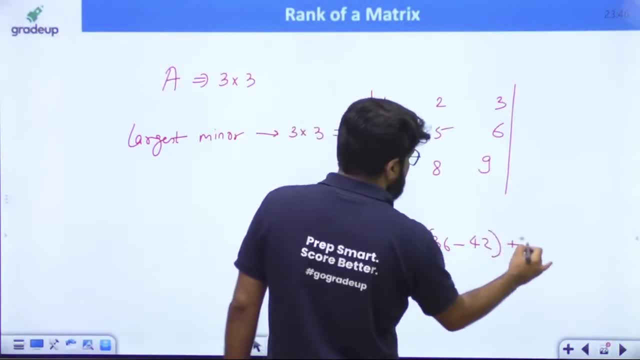 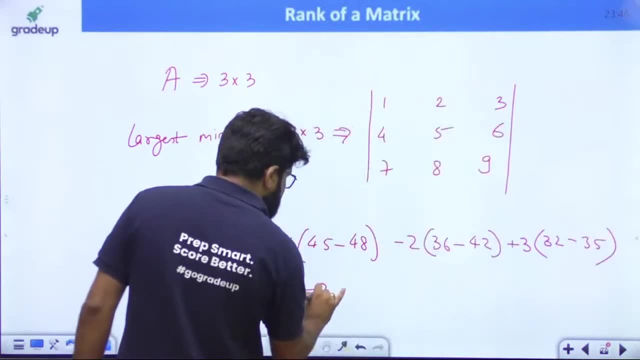 4-9-36-6-7-8-9.. 6-7-42.. Plus 3. Sir, 4-8s are 32.. Minus 7-5s are 35.. What is the value of this determinant then? 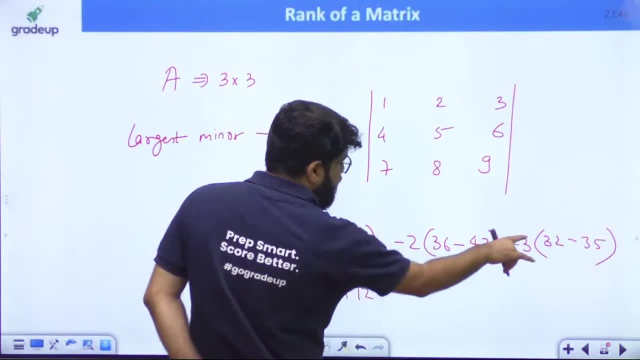 This is minus 3.. Minus 6 into minus 2.. Plus 12.. Minus 3 into plus 3.. Minus 9. And this is 0.. So there is a 3 cross 3 minor which is 0.. 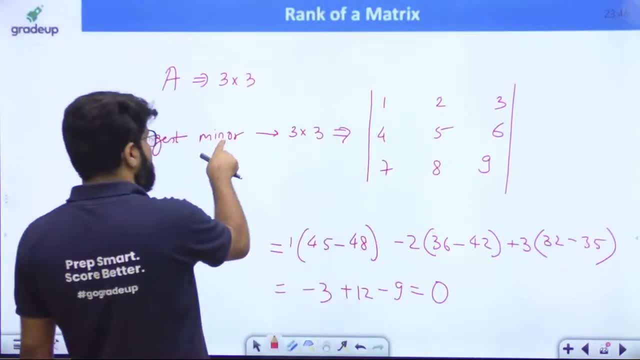 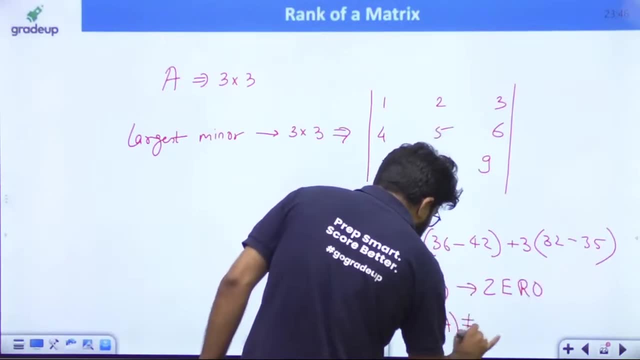 So can rank be equal to 3?? Okay, There is a 3 cross 3 minor, And this is 0.. This is 0.. There is only 1 3 cross 3 minor, and which is 0.. So rank cannot be 0.. 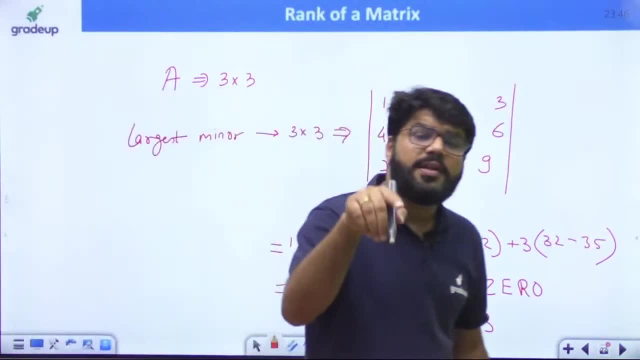 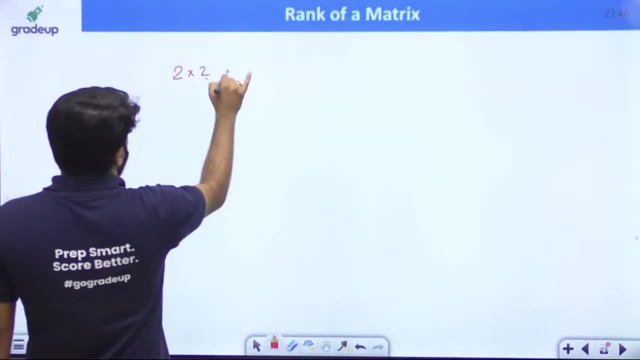 Rank is equal to 3.. Rank is equal to the largest order of non-zero minor. Okay, Can I take the 2 cross 2 minor? Can I now take the 2 cross 2 minor from here? Take any 2 cross 2 minor guys. 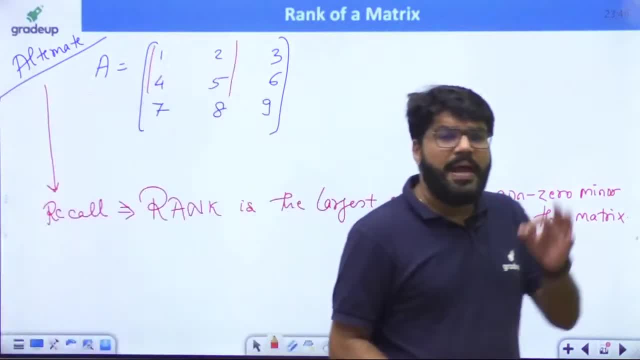 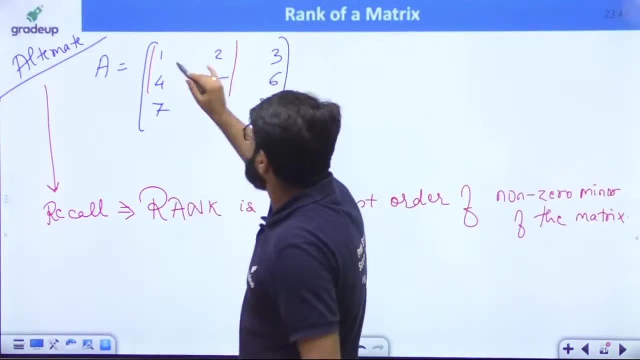 Let's take this. What I told you, What I told you, Minor is any determinant of any size which can be extracted from the matrix. So extract any 2 cross 2.. Let's take these numbers: 1-2-4-5.. 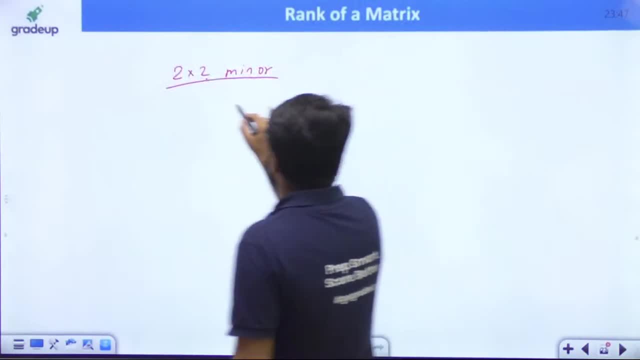 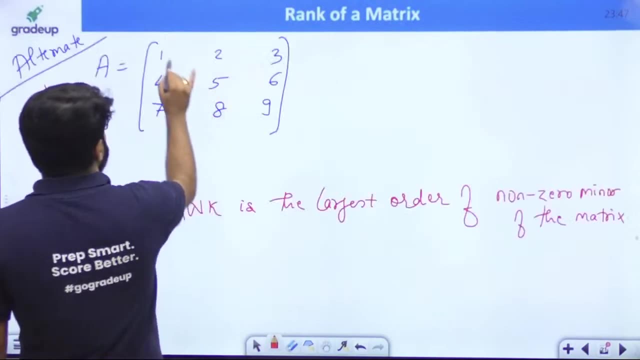 1-2-4-5.. Let's write here: Okay, 1-2-4-5.. Just to highlight this: Any 1. Okay, Take a 1-2-4-5.. What is this determinant? 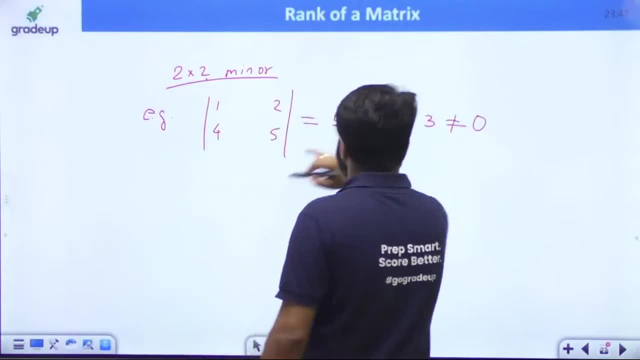 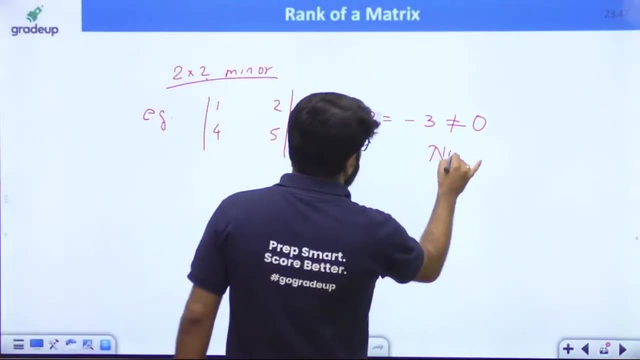 Cross multiply 5 minus 8 minus 3- non-zero. So I have a 2 cross 2 minor, which is non-zero, So the rank is 2.. Okay, This is non-zero, So there is a 2 cross 2 minor. 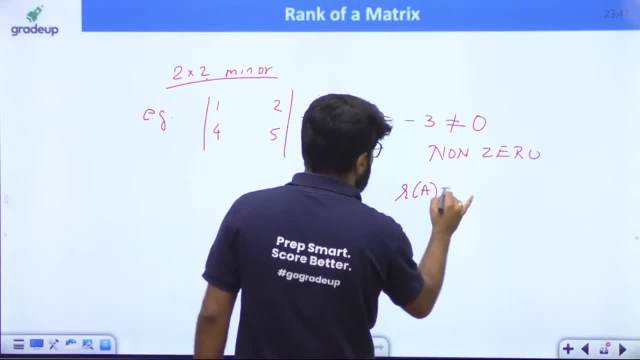 So there is a 2 cross 2 minor. So there is a 2 cross 2 minor which is non-zero. So the rank is equal to 2.. Now I will tell you something more simple. This is the basic concept, This is the basic definition. 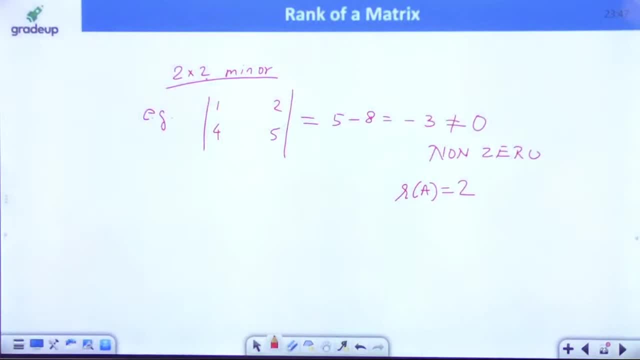 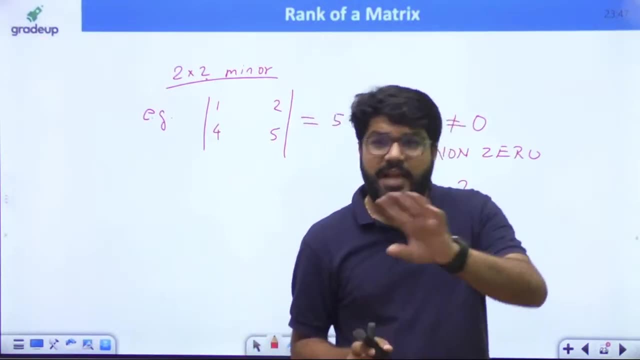 Rank is number of non-zero rows. Correct: Rank is number of non-zero rows. So I have See at least 1, 2 cross 2 minor is non-zero, rank will be 2.. At least You don't have to check all. 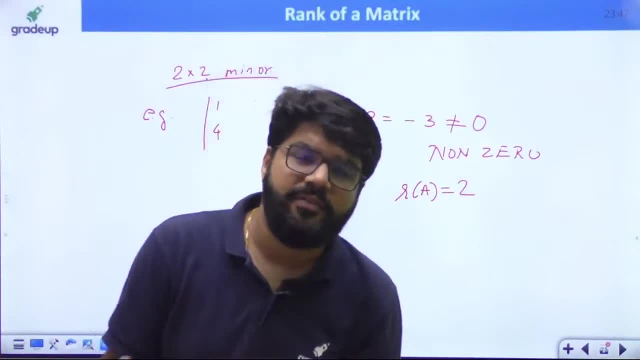 You don't have to check all. At least 1 non-zero minor of order 2 rank will be 2.. Getting it: At least 1 non-zero minor of order 2 rank will be 2.. Sir, can I make it even more simple? 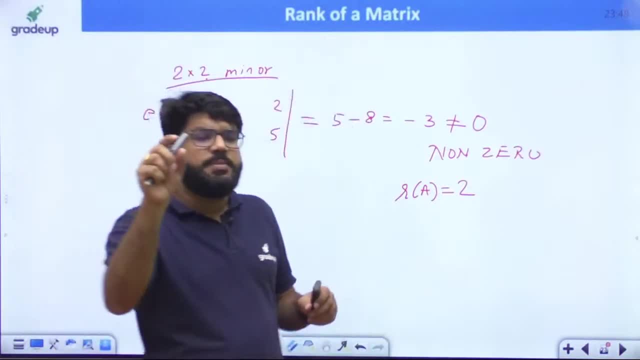 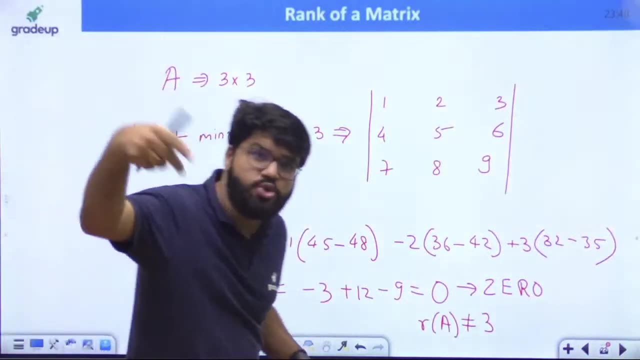 Yes, we will make it even more simple. Yes, we will make it even more simple. But before going to that simple point, one observation. One observation. Okay, Suppose, suppose, suppose, suppose, suppose, suppose, Think, Think. is that? suppose that if determinant was non-zero, 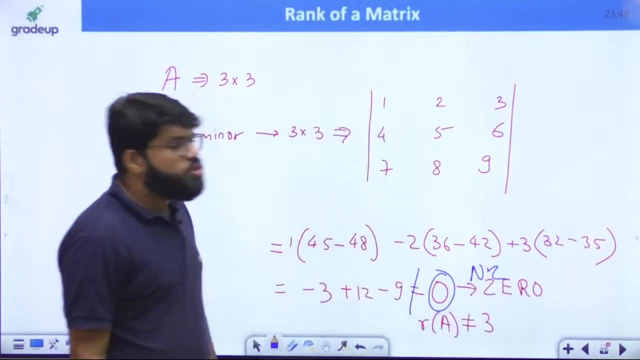 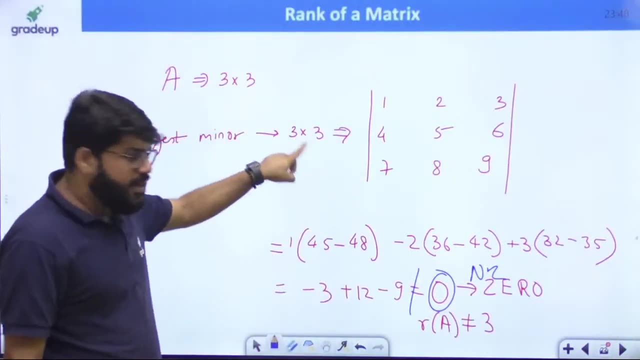 Suppose if it was non-zero. So what will I say? If the determinant was non-zero, then I say that there is a 3 cross 3 minor, There is a 3 cross 3 minor which is non-zero, And the rank will be equal to 3.. 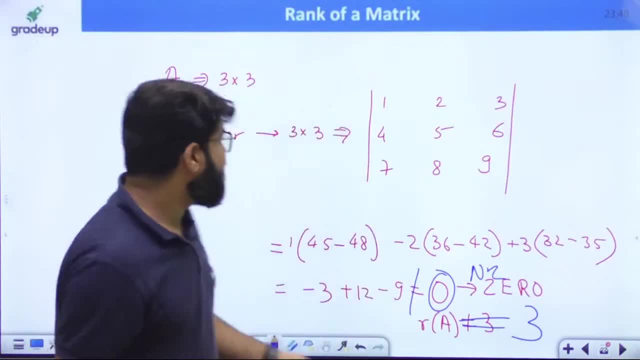 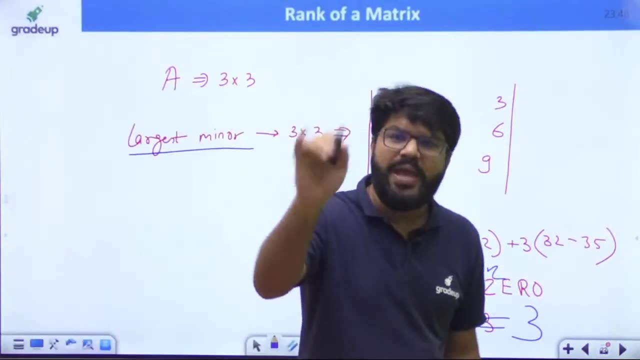 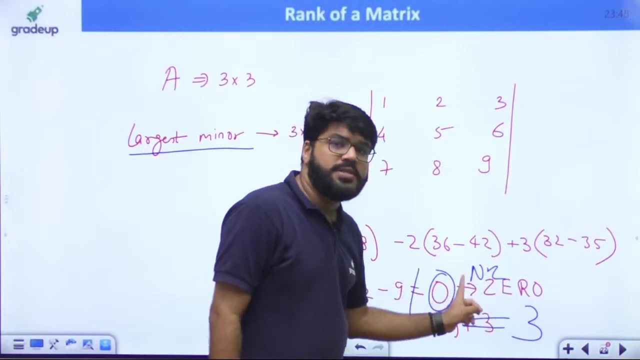 Right Rank will be equal to 3.. And the maximum possible rank is 3, because the largest minor is 3.. The largest minor is 3 cross 3.. So, guys, I can say that for a square matrix, For a square matrix like 3 cross 3, whenever the determinant is non-zero, 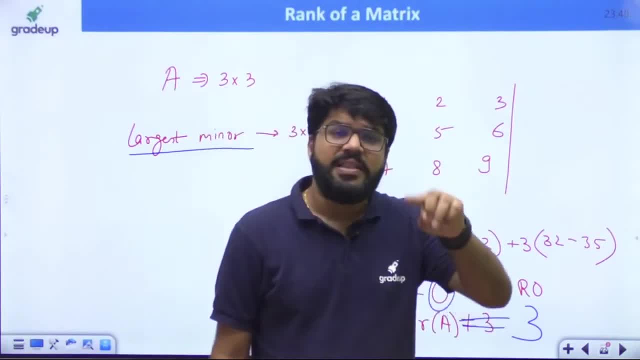 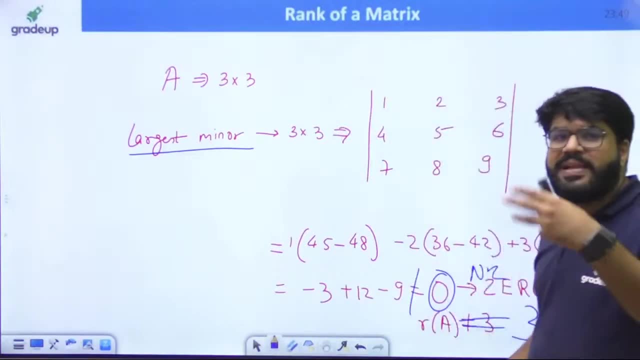 Whenever the determinant is non-zero, the matrix will have the full rank. Matrix will have maximum rank. What is the maximum? What is the maximum rank here? 3. Okay, And it will get the rank equal to 3.. It will get the rank equal to 3.. 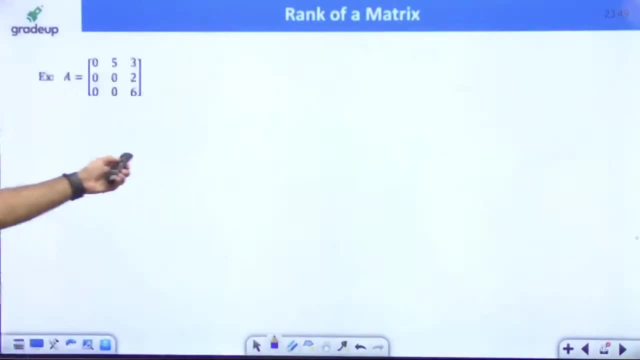 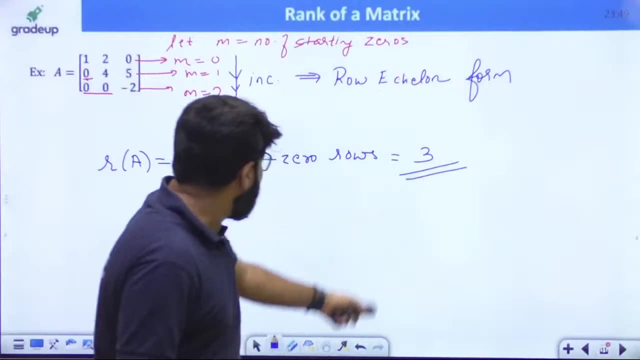 So let me tell you this point. Okay, Yeah, Let me show you with other examples. actually, Let's go to the first question. actually, Let's go to the first question. Let's go to the first question. Everybody Which I explained you with echelon form. 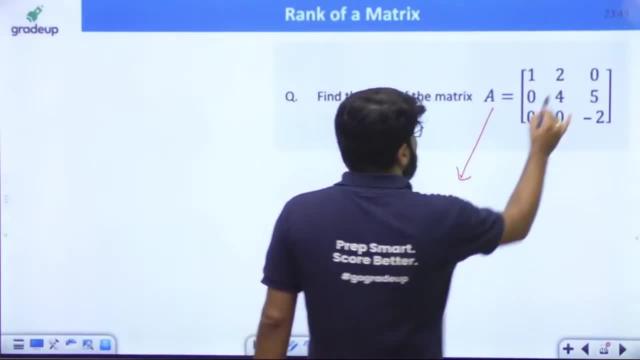 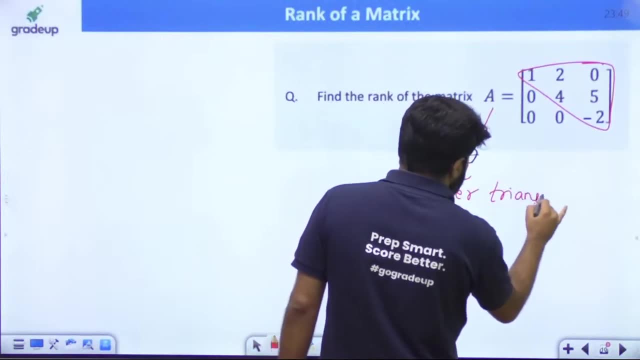 Let's see this with a shortcut. Everybody Have a look at this. Can I say that matrix A is upper triangular? Can I say that the matrix A is upper triangular? Can I say that the matrix A is upper triangular? Can I say that the matrix A is directly upper triangular? for the question number 1?? 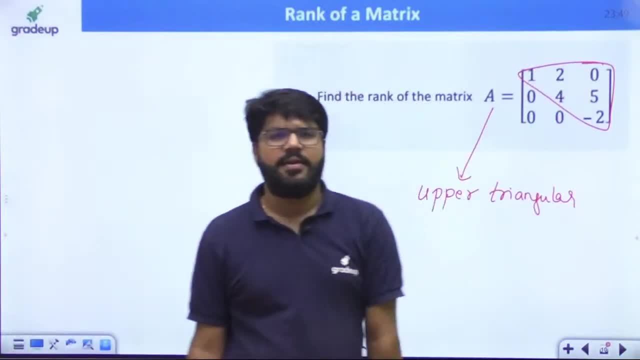 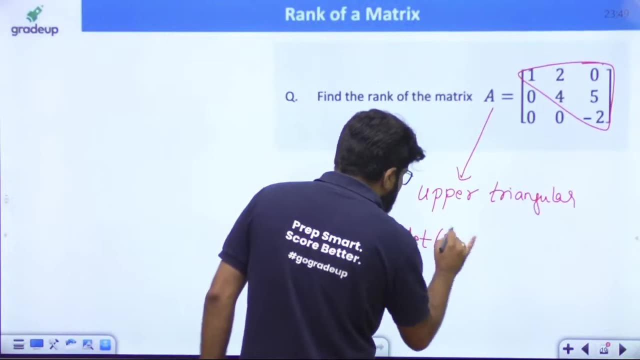 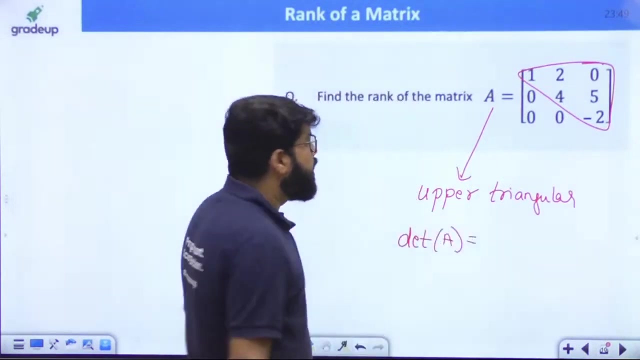 Yes, It is upper triangular. It contains the elements only in the upper triangle, Only in the upper triangle. Getting my point? So this is upper triangular matrix. Okay, So what is the determinant of any upper triangular matrix? Determinant of any upper or lower triangular matrix is product of diagonal elements. 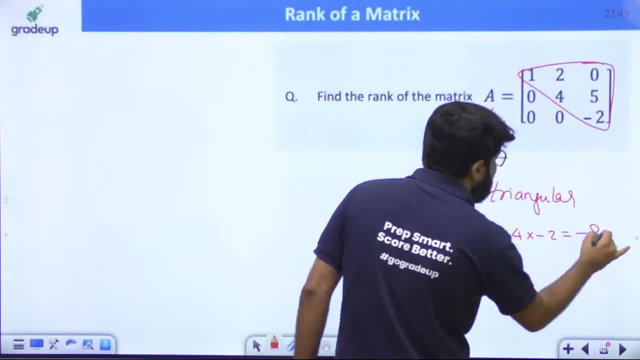 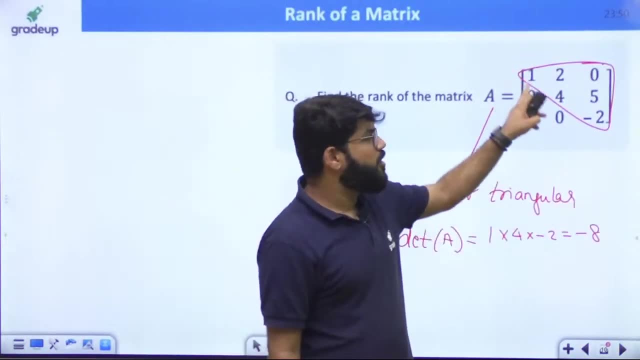 Is product of diagonal elements 1 into 4, into minus 2.. This is minus 8.. This is a basic determinant property. Okay, This is a basic determinant property. The product is the determinant of upper triangular matrix, is the product of diagonal numbers. 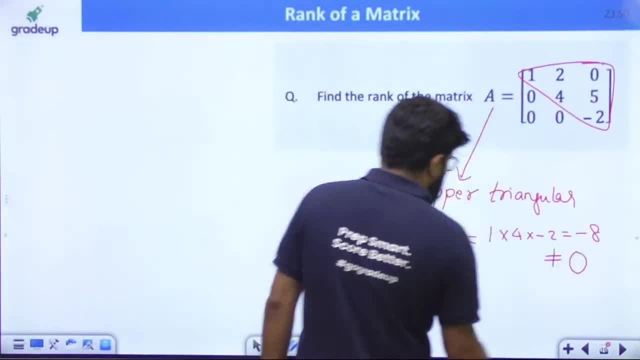 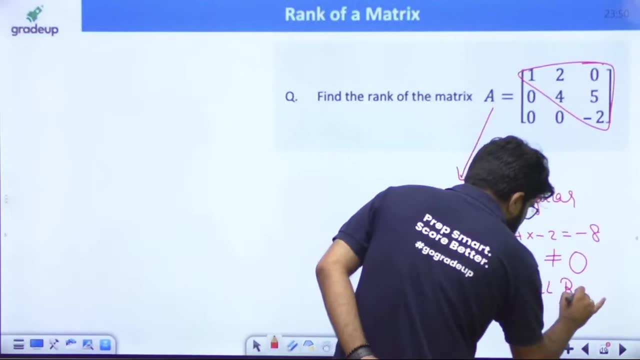 That is minus 8.. That is minus 8, which is non-zero. Right For a 3 cross 3 matrix. if the determinant is non-zero, it will have full rank. It will have full rank. What is the full rank? What is the largest possible rank? 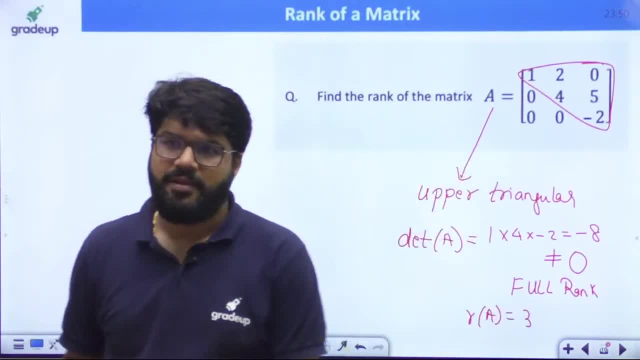 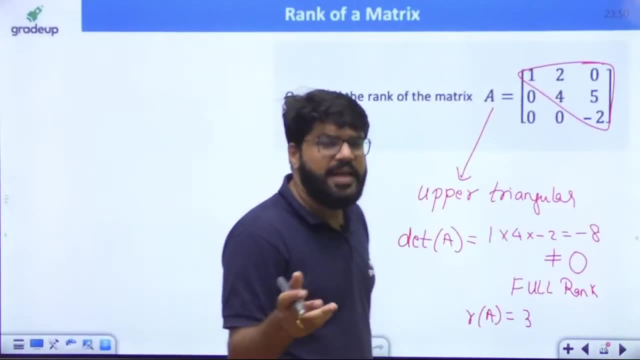 3.. For a 3 cross 3, the largest possible rank will be 3.. Got it, Got this Simple. So either echelon method Or either determinant method, Full rank method, Then dependency wala method coming up next. 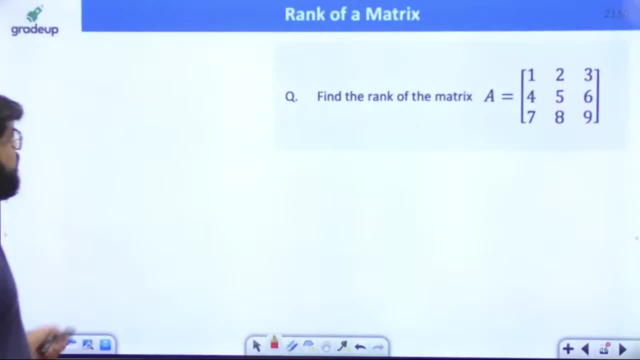 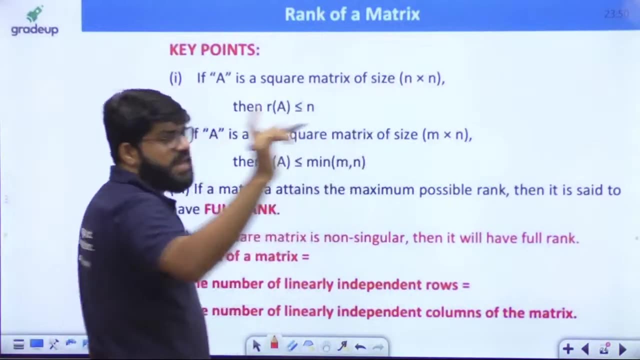 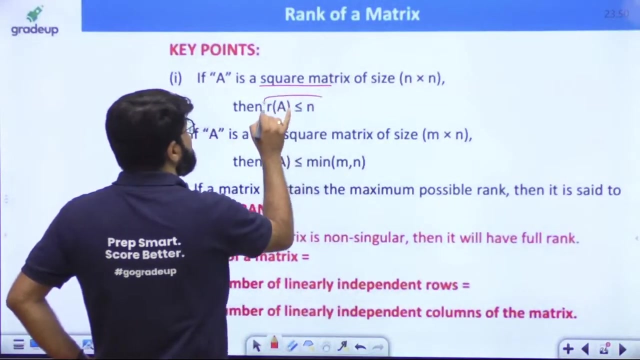 So let us go through one point here. Let us go through one point here before coming to this. Right Guys, Whenever A is a square matrix of size n, cross n. Right, Good evening. Whenever there is a square matrix of size n cross n, then rank is always less than equal to n. 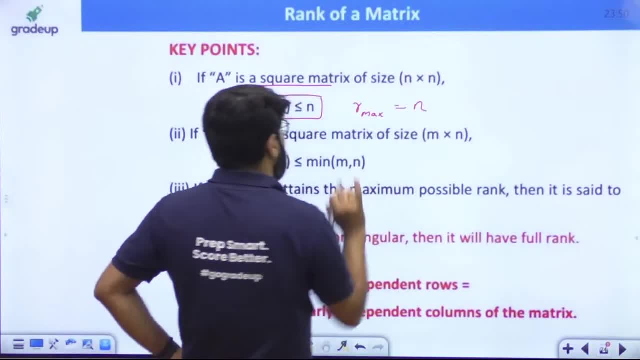 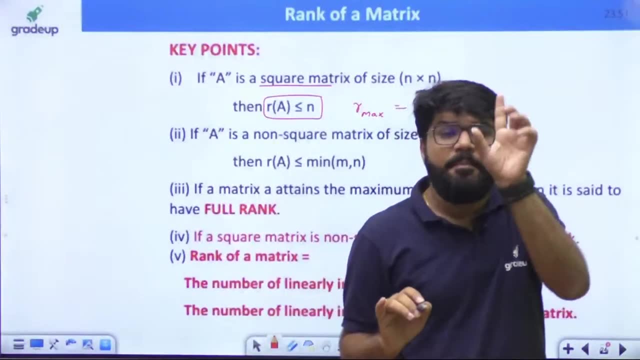 Means the maximum rank is equal to n. The maximum rank is equal to n. It is always less than equal to n. Like I took the example of 3 cross 3 matrix, The maximum rank of a 3 cross 3 matrix can be equal to 3.. 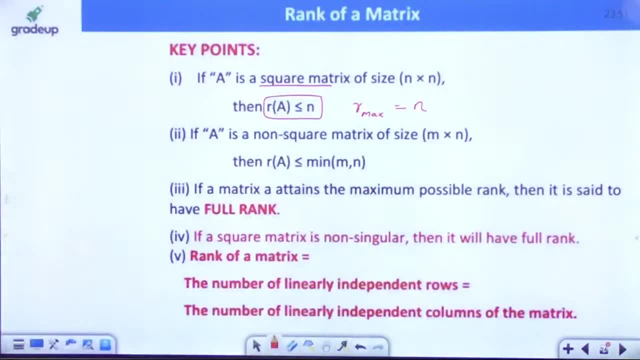 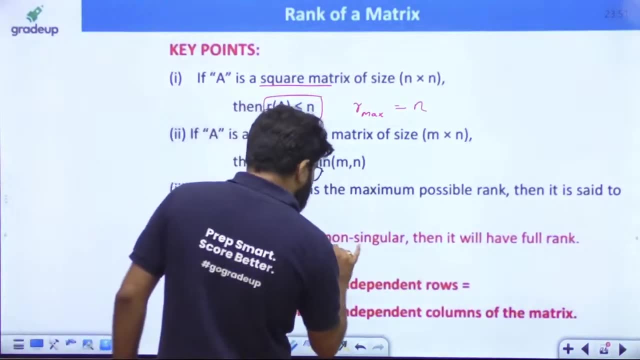 Maximum. Maximum Now, whether it is 3 or not, Whether it is 3 or not, See this. Okay, If a square matrix- Important point- If a square matrix is non-singular, What is the meaning of non-singular? 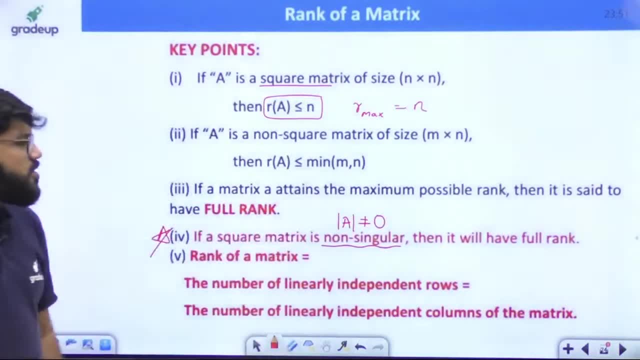 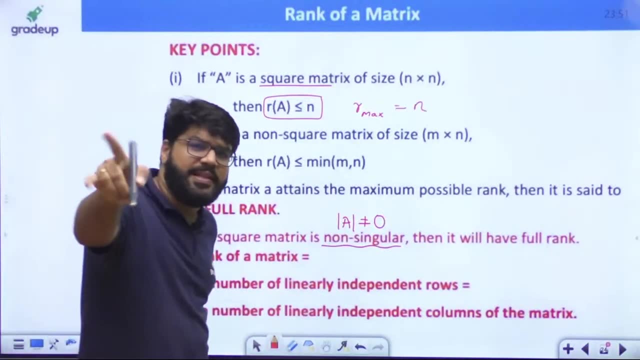 Determinant non-zero. If a square matrix is non-singular, then it will have the full rank. What is the meaning of full rank? Full rank, Right? No PK. If it is rank 2, then we take the largest one. It cannot be 1.. 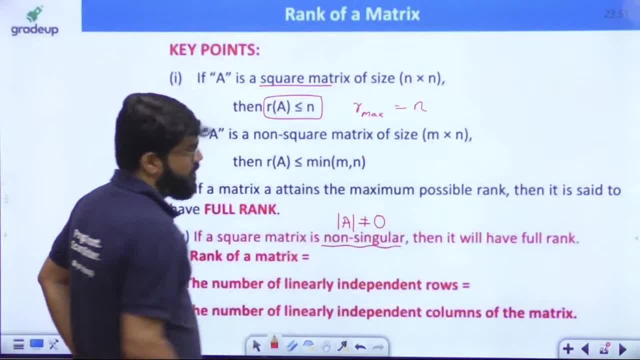 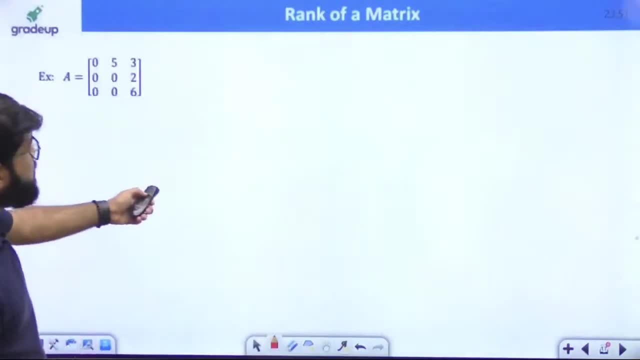 Right, If a matrix attains the maximum possible rank. Okay, If the matrix attains the maximum possible rank. Question number 1.. Okay, Question number 1.. Once again, I will jump to the question number 1.. Have a look at this. 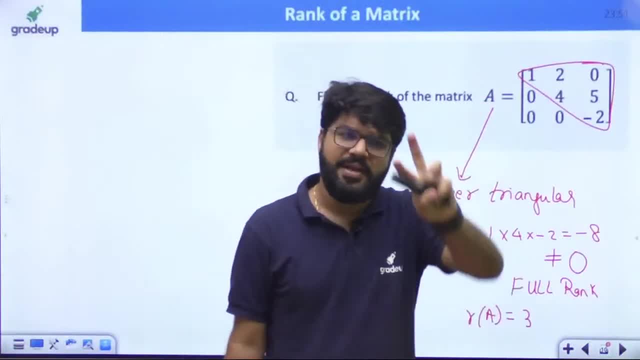 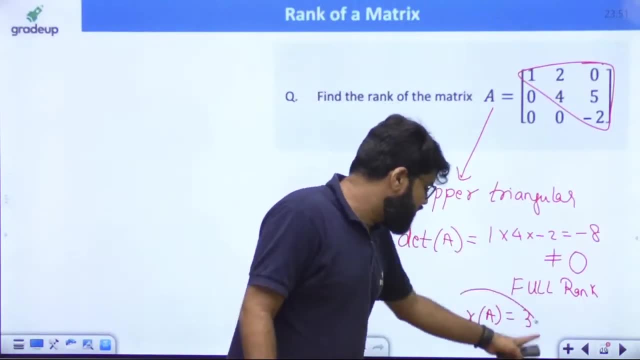 Okay, This matrix is 3 cross 3.. So what is the maximum possible rank, Sir, 3.. What is the determinant? Non-zero. So rank will be 3.. So whenever the matrix gets, Whenever the matrix gets the maximum value of the rank, 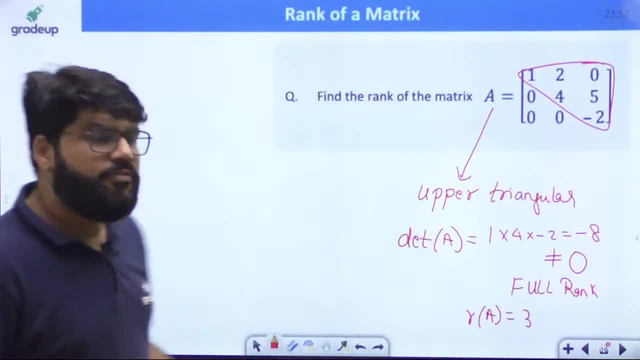 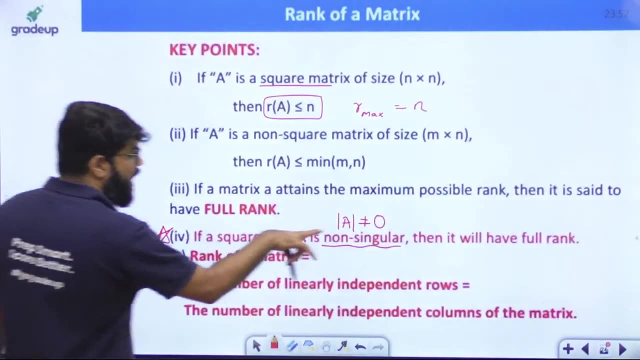 Then it is said to have the full rank. Then it is said to have full rank. And when will the full rank of the matrix be? A square matrix, Let's come to the point, Will have full rank if the determinant is non-zero. 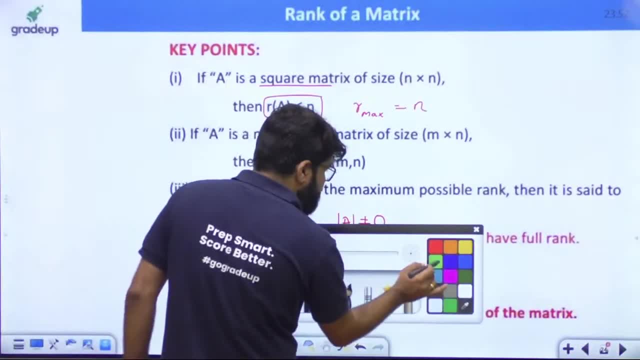 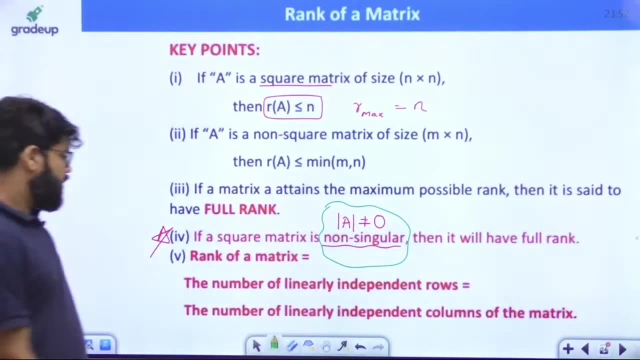 If it is non-singular, Important point: If it is non-singular. If it is non-singular, Right Okay, Now we are skipping the last point. This is actually very, very, very, very important. We will see this also. 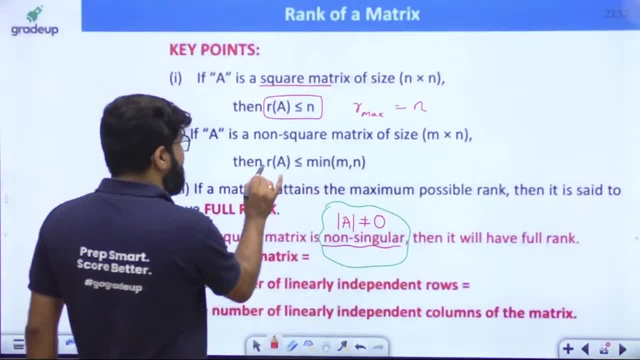 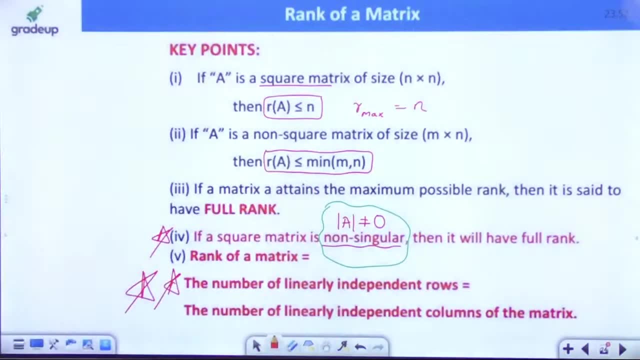 But if it is a non-square matrix of size- m cross n- Then what is the maximum value of the rank? Okay, That is minimum of m or n. Rank is always less than equal to minimum of m or n. Okay, Very good. 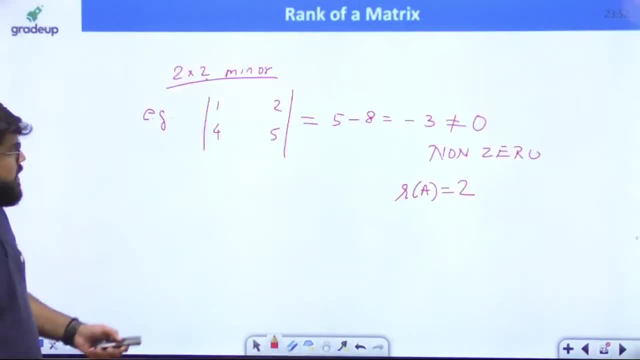 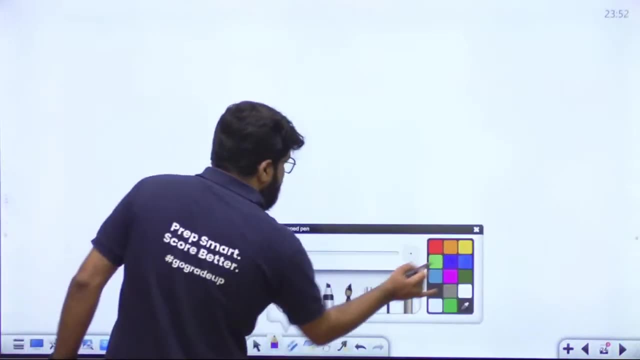 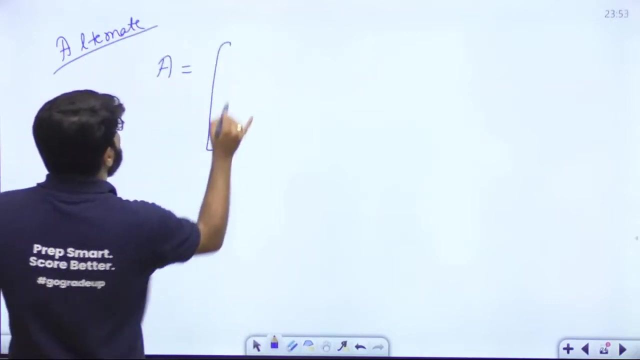 Now. Now Let's take another question. Before going to the another question, Let's learn one more method, And then questions, Then questions to follow. One more alternate method, One more alternate method, Same matrix. First, we will experiment on the same matrix. 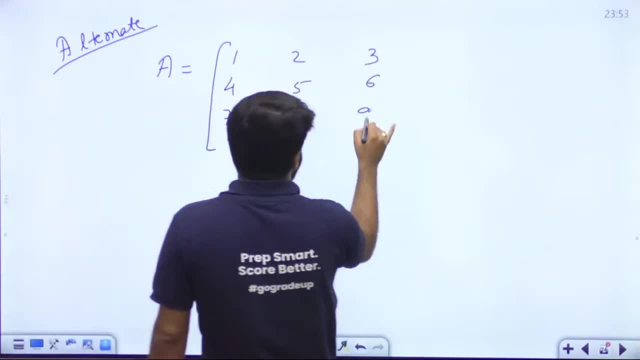 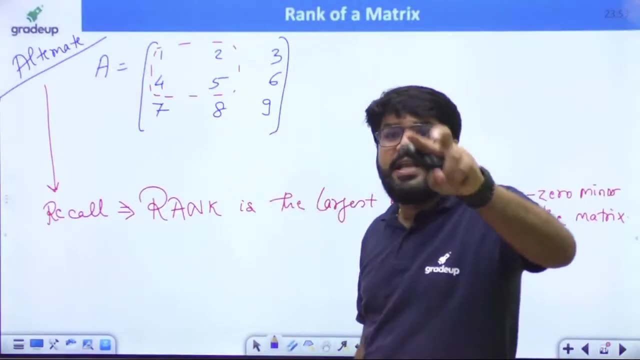 1,, 2,, 3,, 4,, 5,, 6,, 7,, 8,, 9.. Okay, Same matrix. I have solved this with the echelon form. I have solved this with the determinant method. 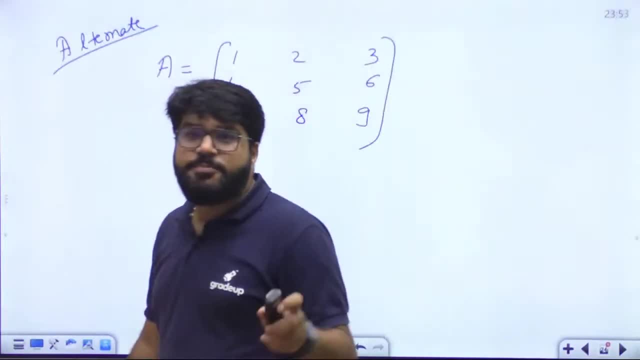 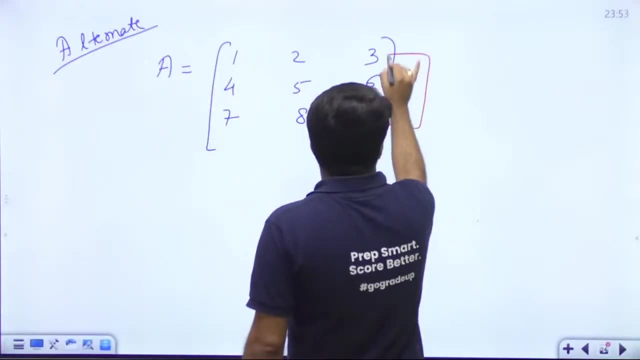 And now the third. Third Is observation Which may be simple for some, questions Which may be complicated for others. That is why I am telling you variety. Okay, Guys, Let us try to add R1 and R3.. Can we add R1, R3?? 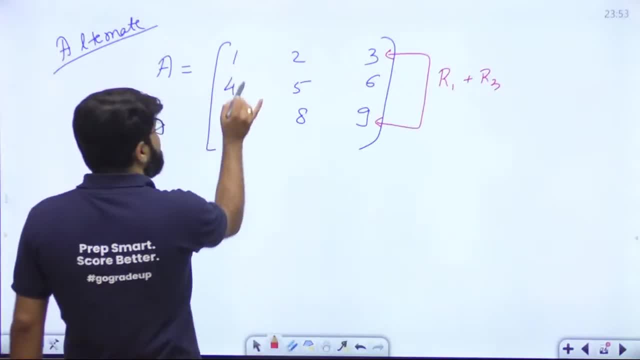 Let's try to add R1, R3.. Look, 1 plus 7 is 8. Which is double of 4.. Next, 2 plus 8 is 10.. 2 plus 8 is 10.. Double of 5.. 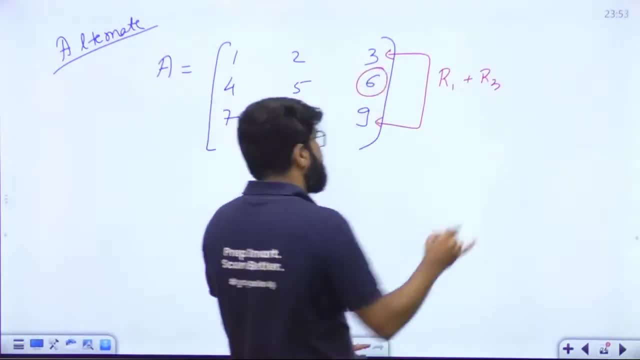 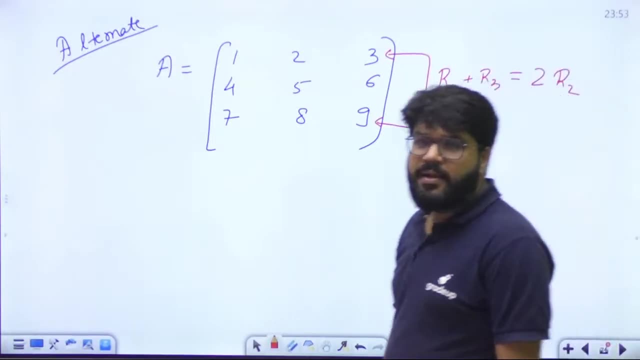 Right, 6 plus 9 is 12.. Double of 6.. So whenever I add R1 and R3. What I am getting? I am getting double of the row number 2.. I am getting double of the row number 2.. 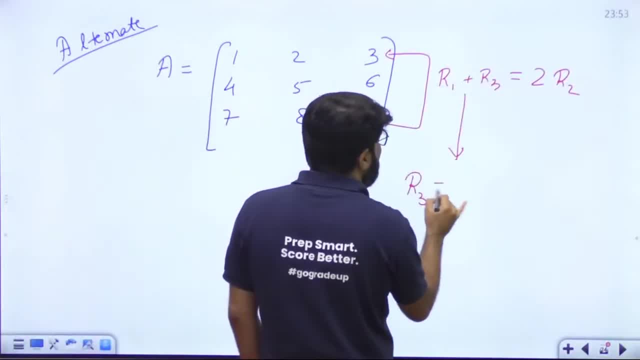 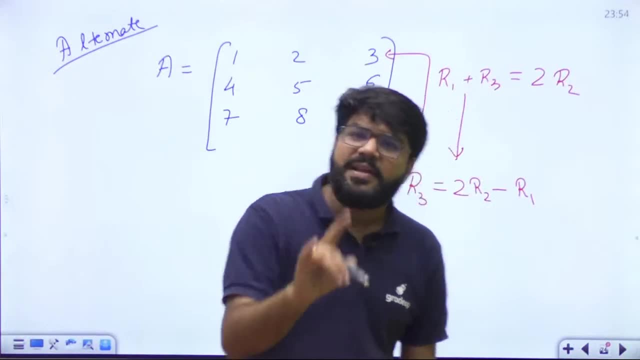 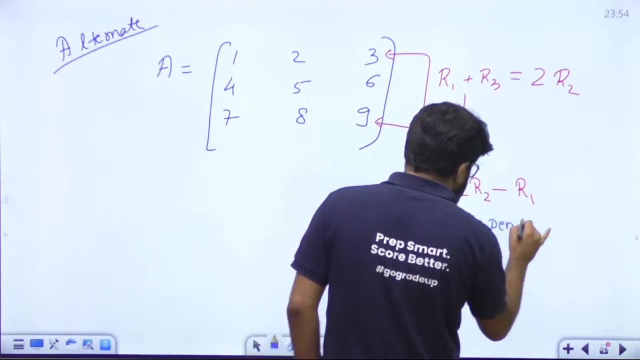 Or I can say that, Or I can say that R3 can be written as 2 R2 minus R1. Whatever, you have to rearrange That means That clearly means that This clearly means that This matrix has one dependent row. 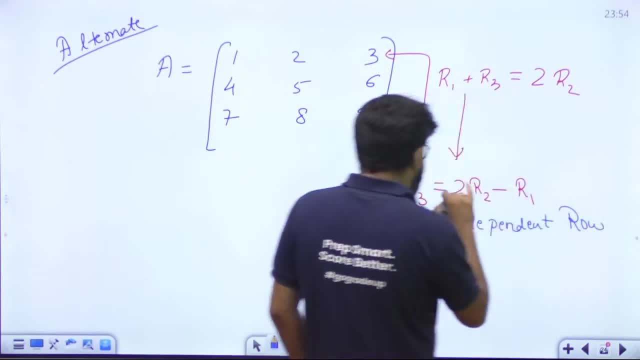 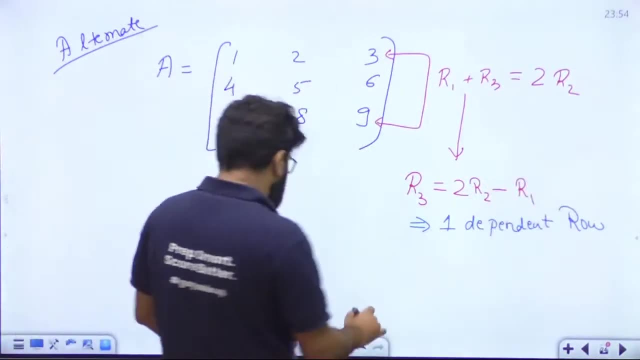 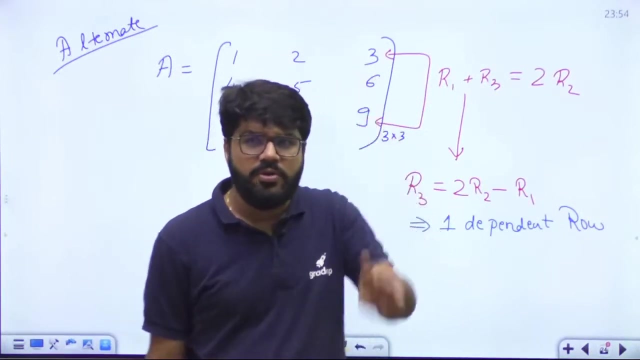 This has one row Which is dependent on the other two rows. So how many independent rows? It is a 3 cross 3 matrix: 3 cross 3.. It has 3 rows. It has 3 rows Out of the 3 rows. 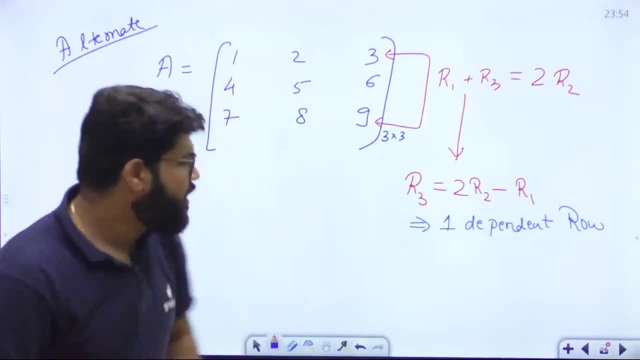 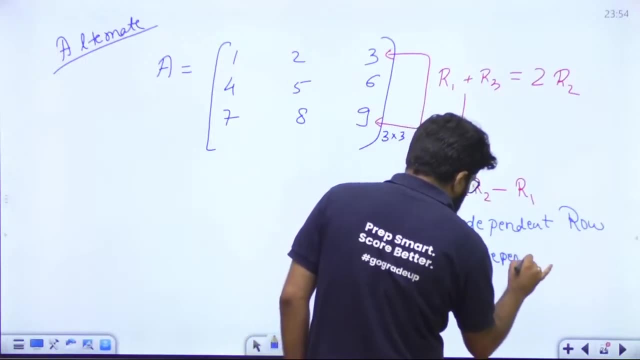 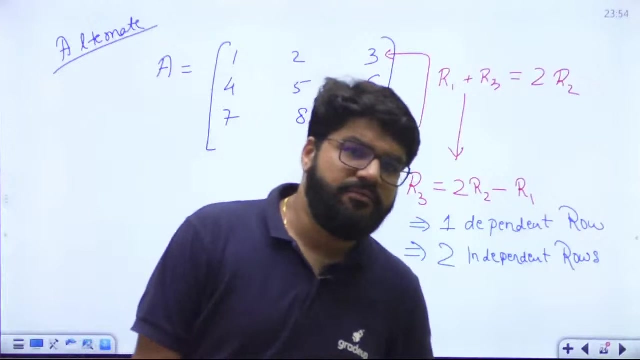 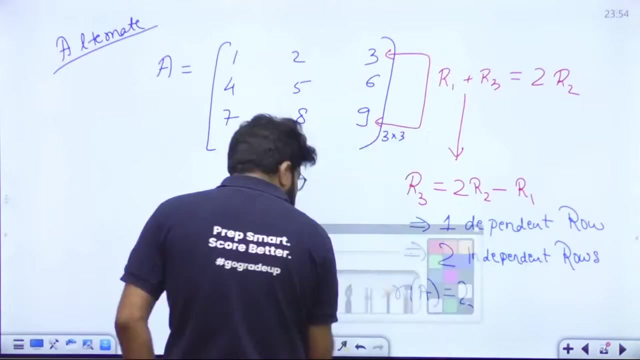 One is the dependent row. One is the dependent. How many independent? How many independent? It has 2.. 2. 2 independent rows. It has 2 independent rows, Everybody. It has 2 independent rows, Okay, And the rank of a matrix is always equal to. 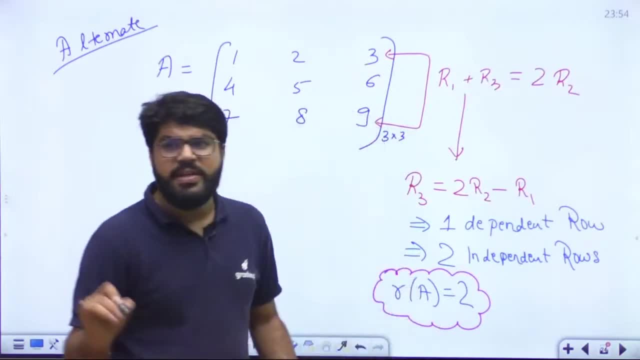 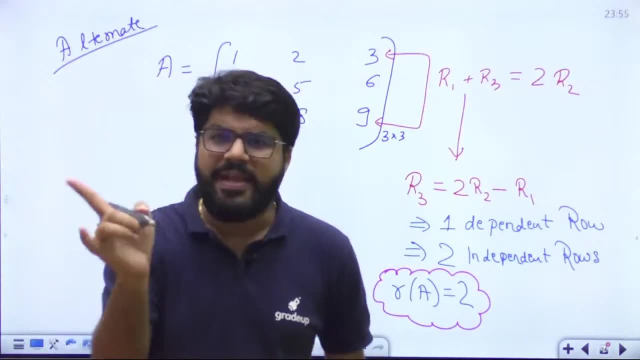 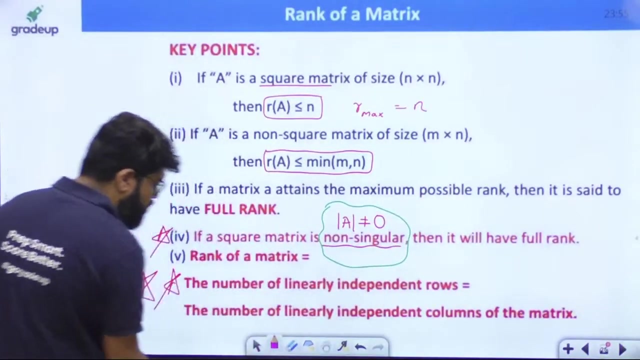 The rank of a matrix is always, Always, 100%, true- Is always equal to number of independent rows Or number of independent columns. Check any one: Either row to row or either column to column, The rank of a matrix is equal to number of linearly independent rows. 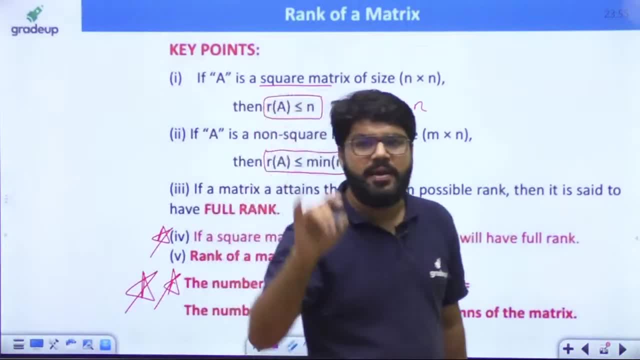 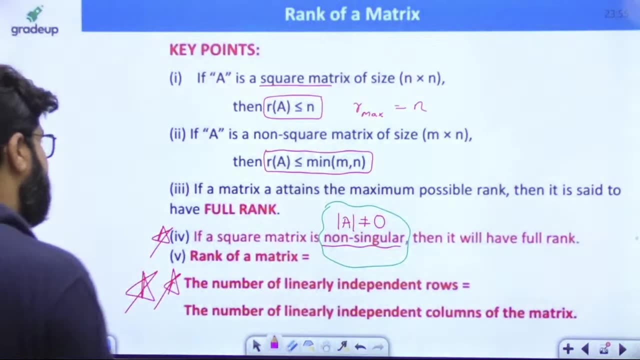 Or equal to the number of linearly independent columns of the matrix. Number of linearly independent columns of the matrix. Now, this can make some of your questions and some of your life easy. Can you say the answer for this? Now, these are: 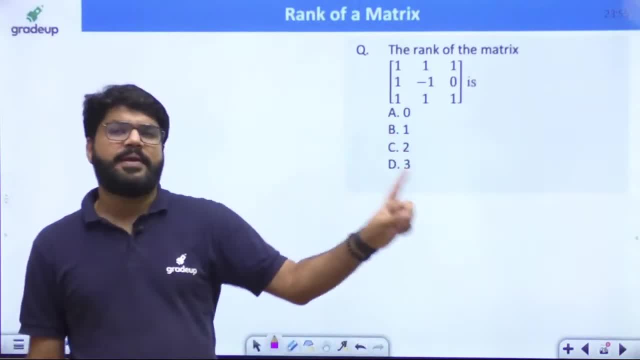 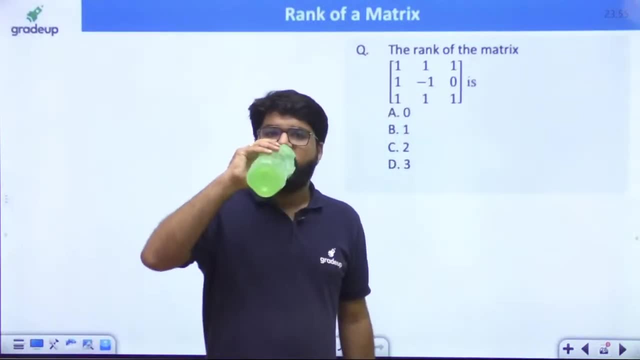 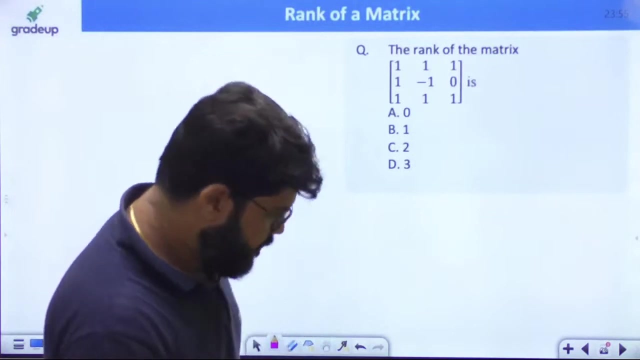 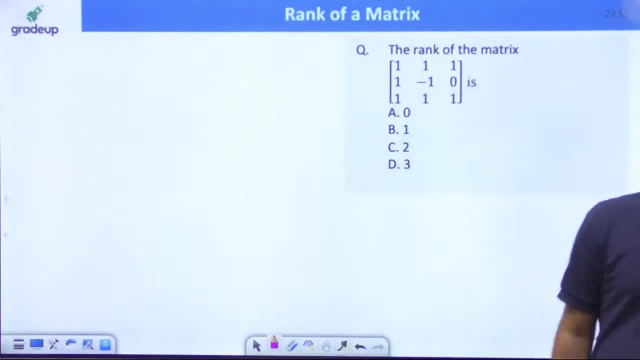 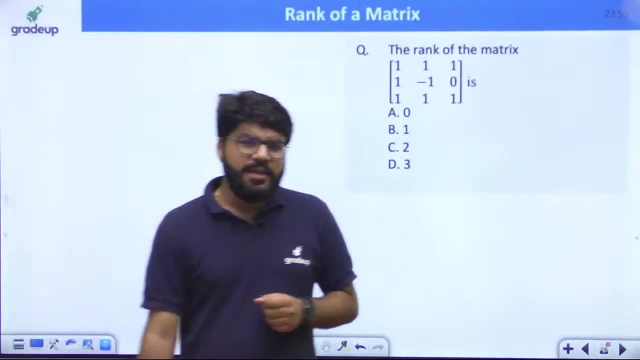 100 likes. Yeah, Great, Great, Great That, Josh. That shows your Josh, But I think it's not as high, Josh, as 10 pm. Should we shift? Should we shift to the 10 pm I'm expecting here? 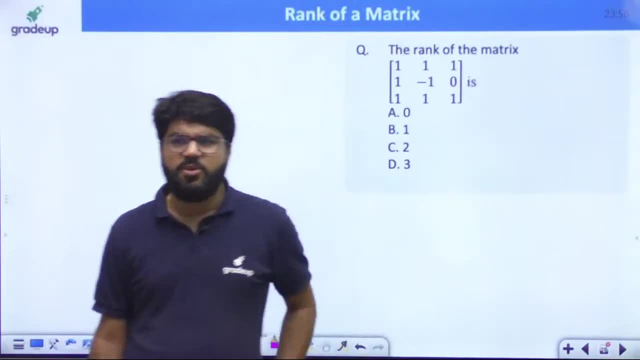 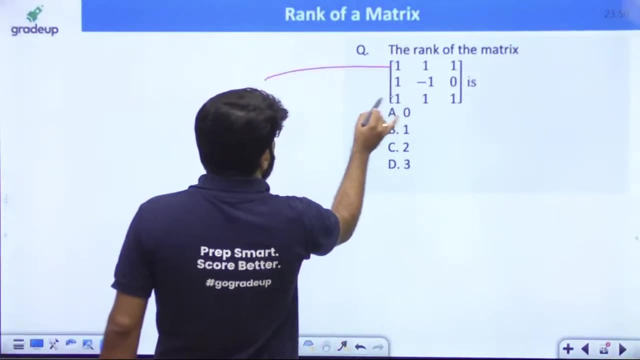 The late. I want to see the dedication of the students. I want to see the energy also, How much energy we are giving at any point of the time. But now, guys, have a look at this, Have a look at this, Have a look at this. 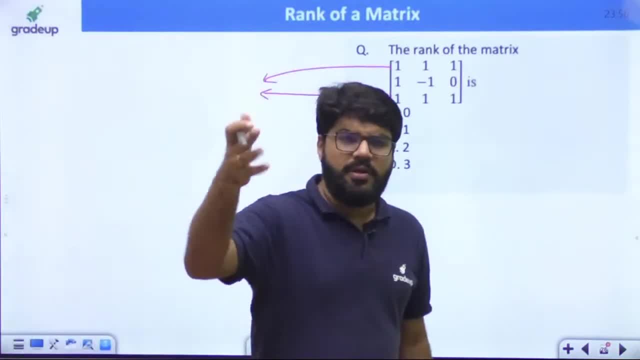 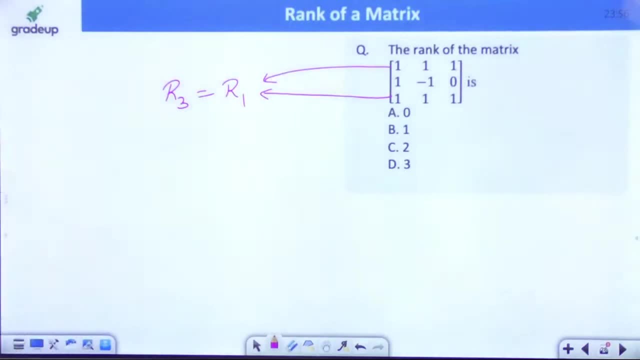 This is observation Now, no need to convert into a echelon form and all Not required. Not required. But I am able to see that the row number three same as row number one, Same R3. same as R1.. R3- same as R1.. 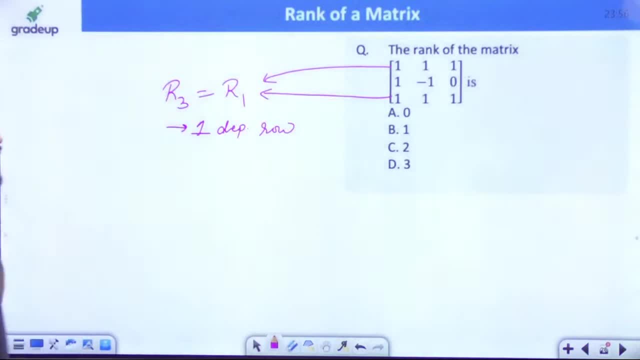 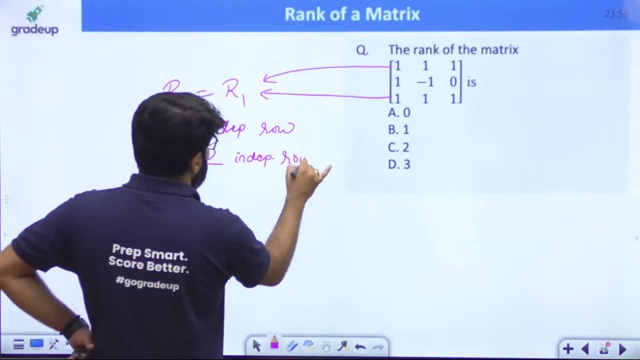 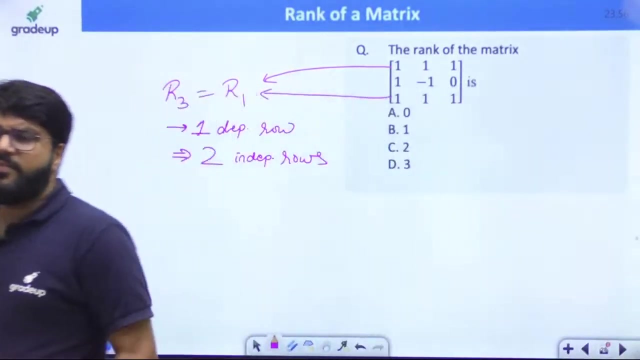 So there is one dependent row, R3, same as R1.. One dependent row, Okay, So two independent rows. How much? Two independent rows? Right, There are the two independent rows. And if there are the two independent rows, If there are the two independent rows. 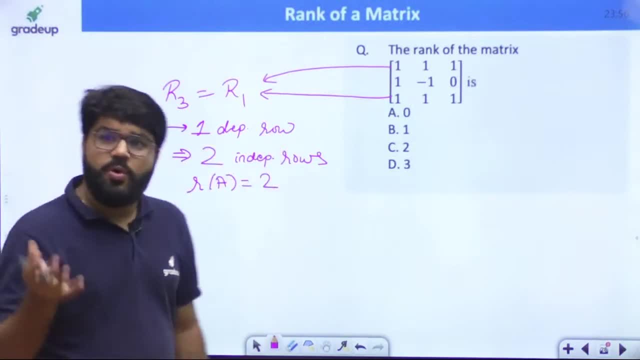 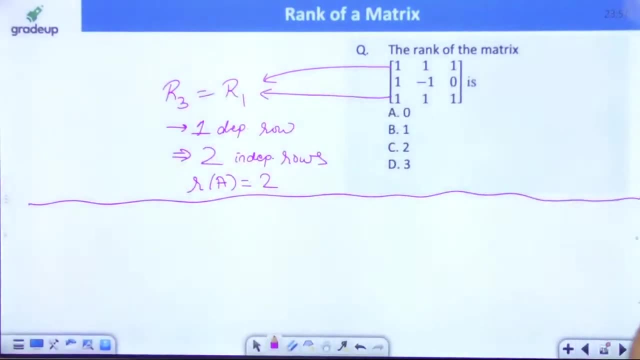 The rank of the matrix should be two. I will tell you both the ways, Come on. What can be the other? Other, other, other. No, I am not free at 8 pm. Okay, What can be the other? 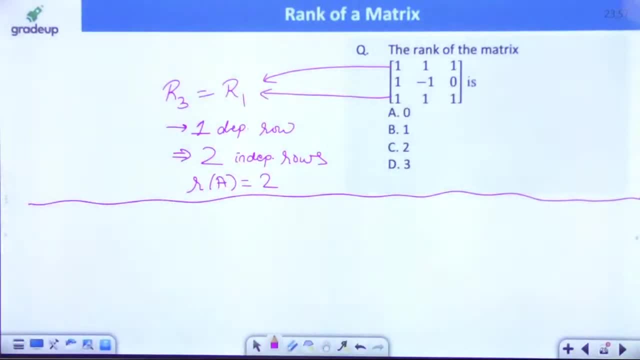 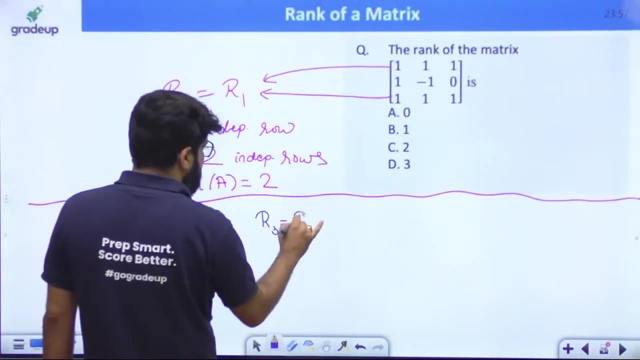 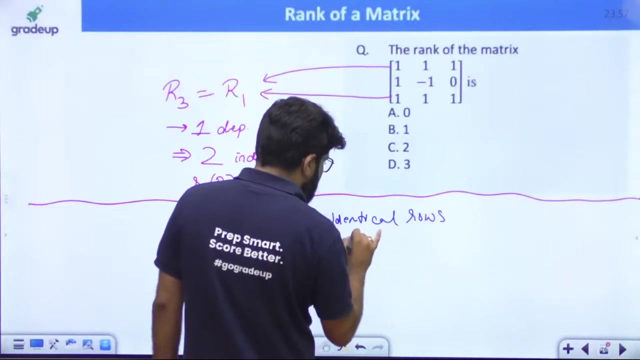 Rank is equal to two. So what should be the other method? Okay, Alternate, you can say this. Alternate, you can say this, Sir, R3 equal to R1 means identical rows Means identical rows. Whenever a matrix has identical rows, its determinant is zero. 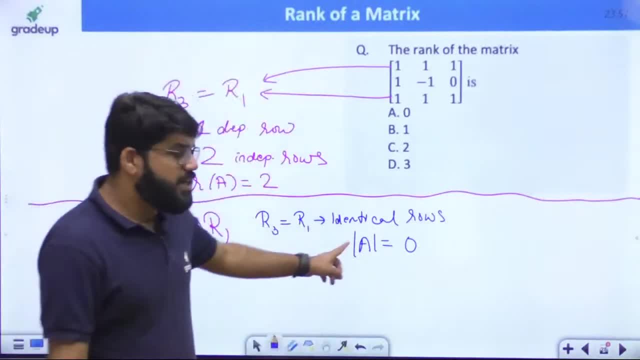 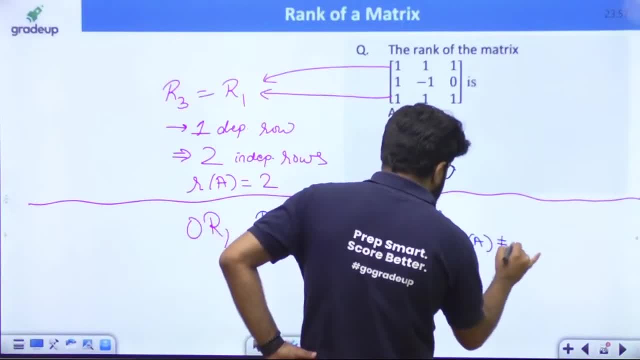 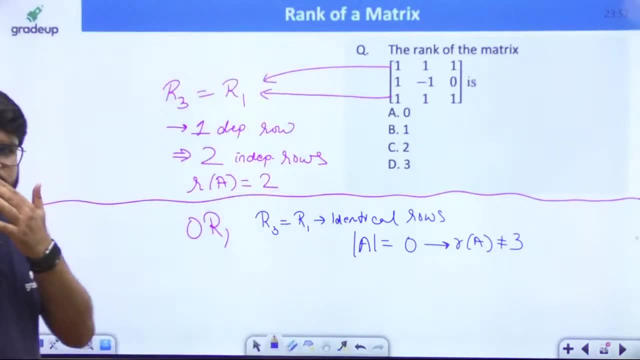 If the determinant is zero. So we should know that rank is not equal to three. Rank cannot be full. Determinant non-zero chahiye then we have full rank. Okay, Because it is clearly seen Vishnu. Okay, So determinant equal to zero. 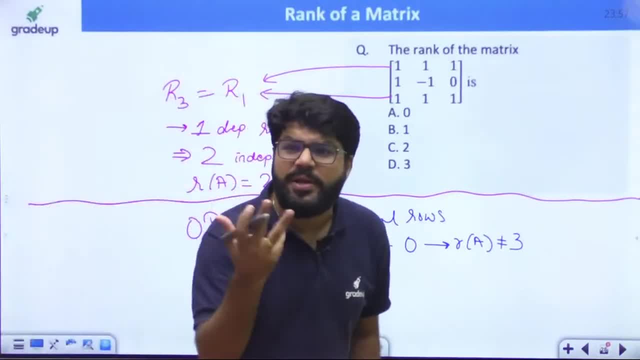 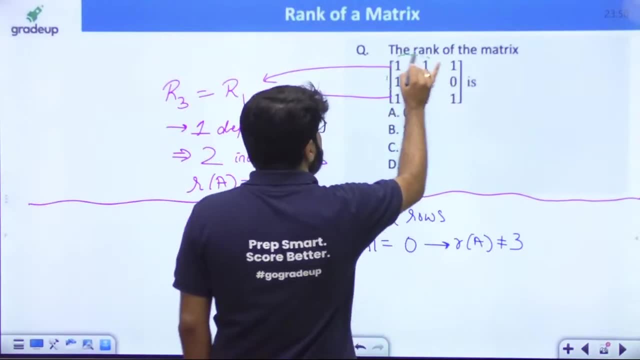 Rank is not equal to three. So rank three nahi hai. ye confirm, Is it equal to two? Is it equal to two, Koi chek karte nahi maine mula take any one, Take any one. Let's take this determinant. 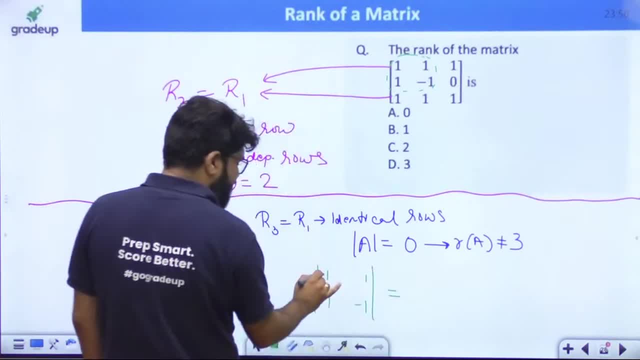 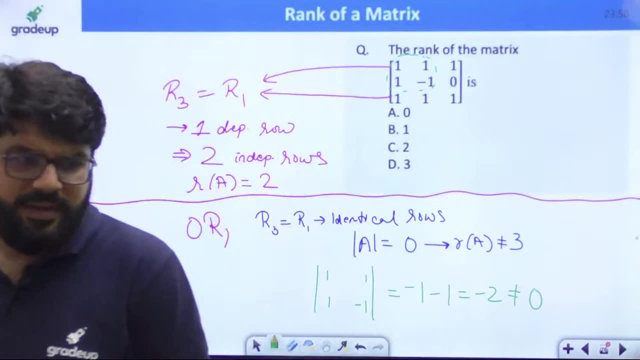 One One, One minus one. Let's take any two cross, two minor Cross multiply minus one minus one is minus two, not equal to zero. I hope this green color is visible. Yes, I think it is visible. Now I have a two cross, two minor, which is non-zero. 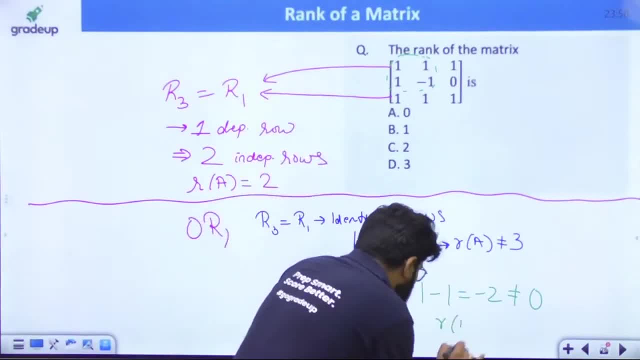 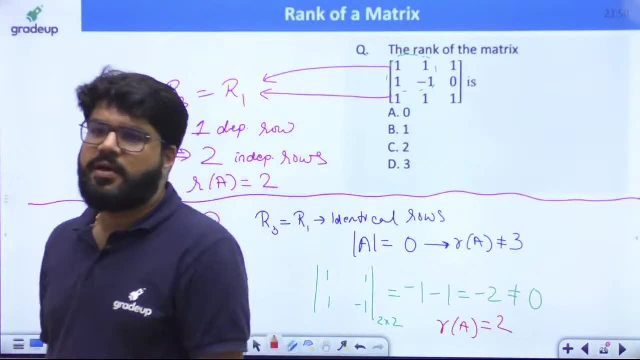 And if there is one, two cross, two minor, which is non-zero. So the rank, Sir, So the rank should be two. Yeh dekhiye, yahan se bhi bol diya: Rank is two, Rank is two Right. 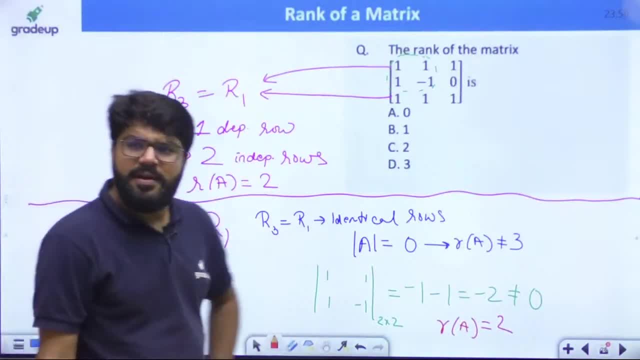 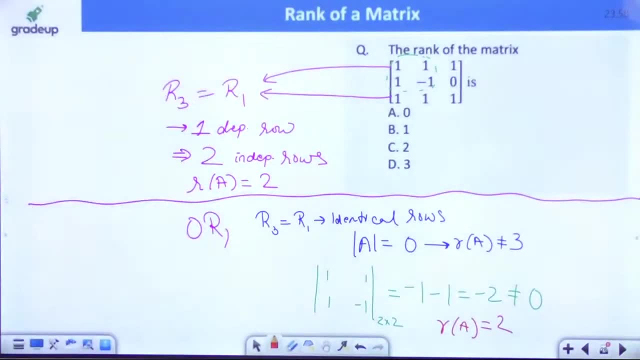 So one dependent rows either by the dependency method or either by the basic determinant method. again, Correct. Both the methods are explained. again for the same question. Again for the same question. both the methods are explained, Explained. Got it Chalo great hai. 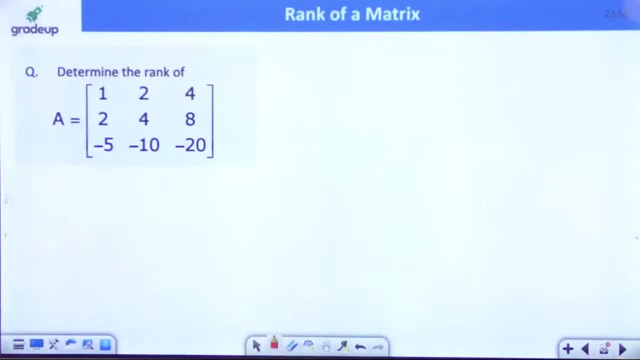 Next, Next, Next, Next question: Have a look at this and answer me. Determine the rank of this matrix Everybody. Determine the rank of this matrix Everybody: One, two, four, two, four, eight minus five minus ten minus twenty. This will lead to an important point. 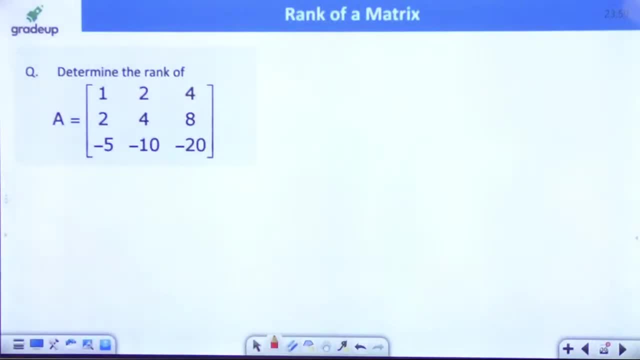 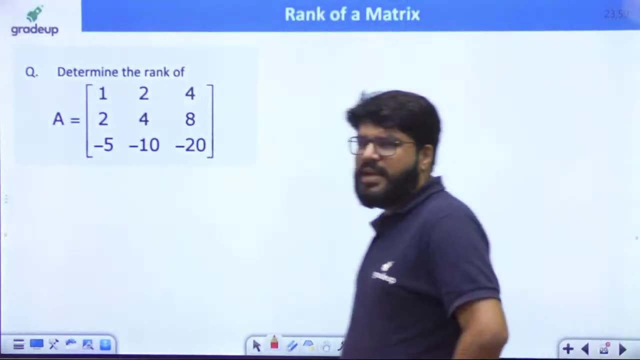 This will lead to an important point, Hai Deva. This will lead to some more important conclusion. Everybody, What is the rank of this matrix? Everybody, answer me. I'm waiting for your answer. then I will begin. Let me know the rank of this matrix, waiting for your. 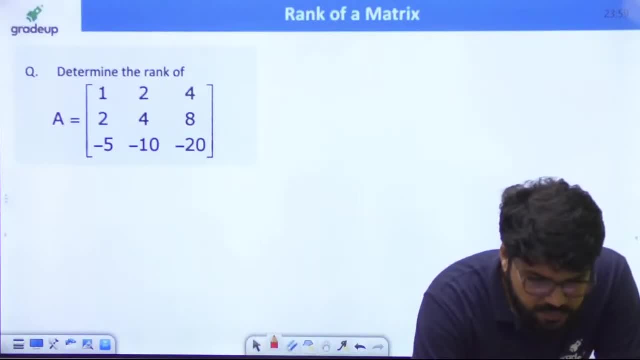 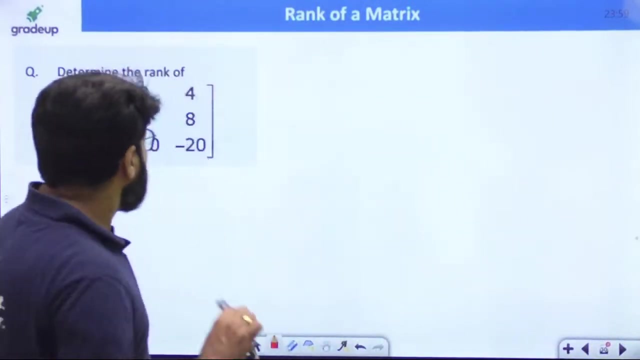 comments. Yes, Just waiting for all of your comments. It depends on question to question. Just that is why I've given the variety, and practice will set that into the mind. Okay, guys, So many of you are coming up with the answer as one. 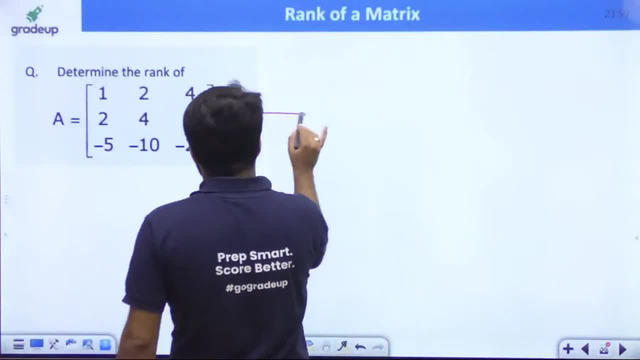 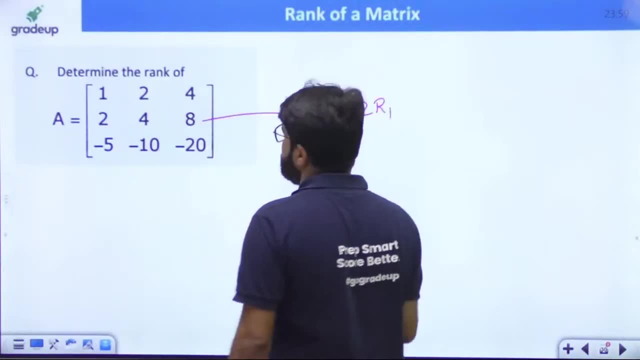 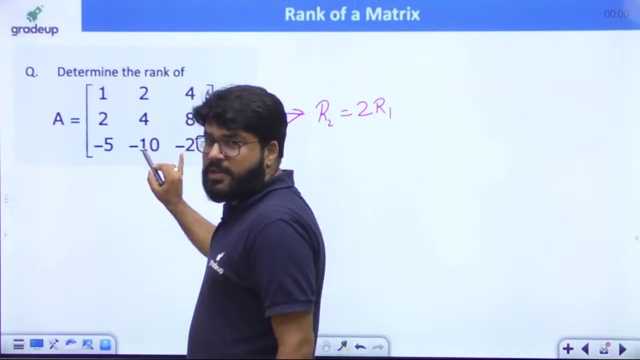 See, guys. basically, what is the observation here? that one into two is through two of the four fortunes are eight. so that means the R2 is equal to. R2 is equal to two or one. What is this? one into minus five. minus five is minus 20.. 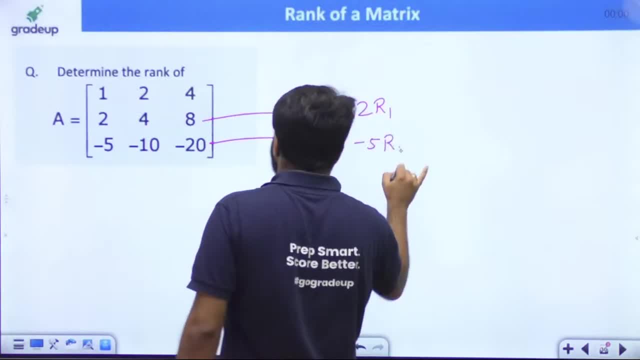 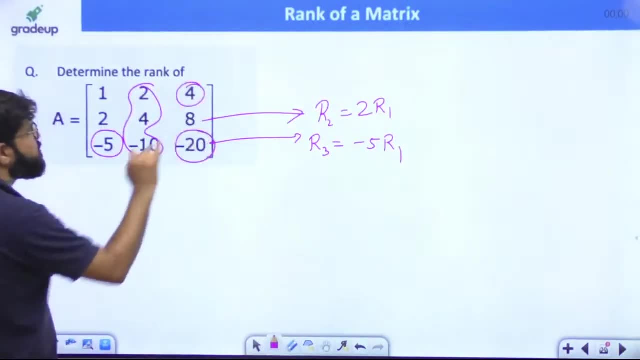 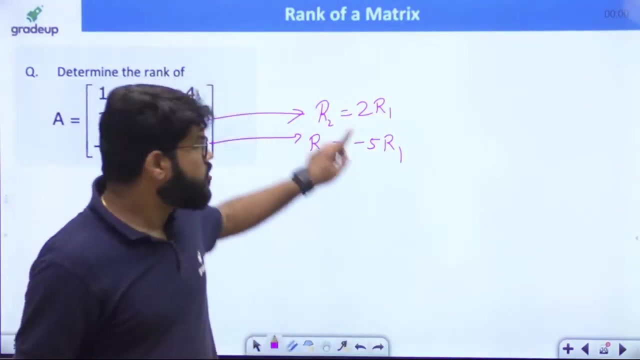 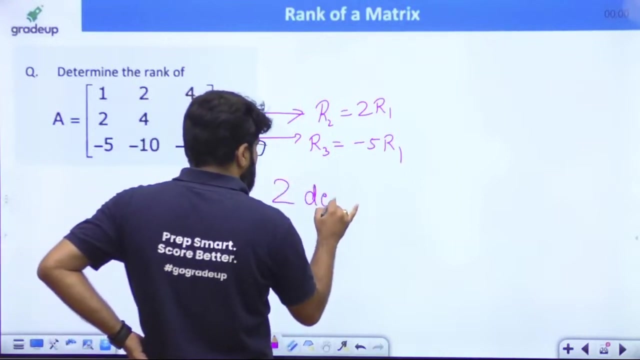 So what is this? R 3 is minus five or one. or once again see, one in two minus five is minus five. two into minus pi, minus ten, four into minus five minus twenty. So clearly are, three is minus five or one. So how many dependent rows? R2 also depends on R1.. R3 also depends on R1.. Two different types of dependency. So, sir, there are two dependent rows. There are two dependent rows. So how many independent rows? 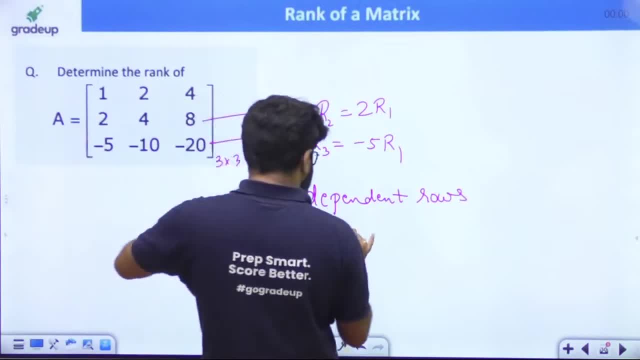 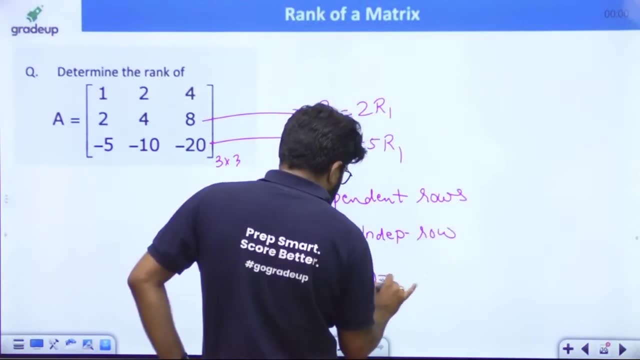 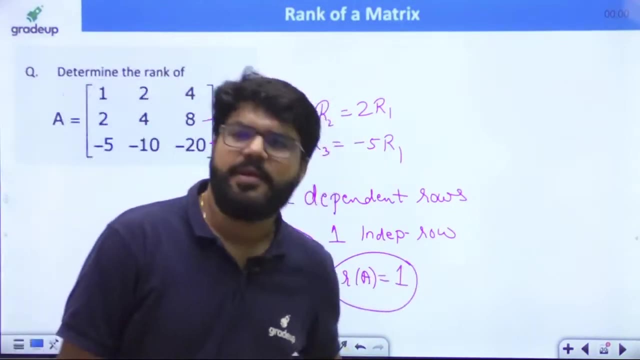 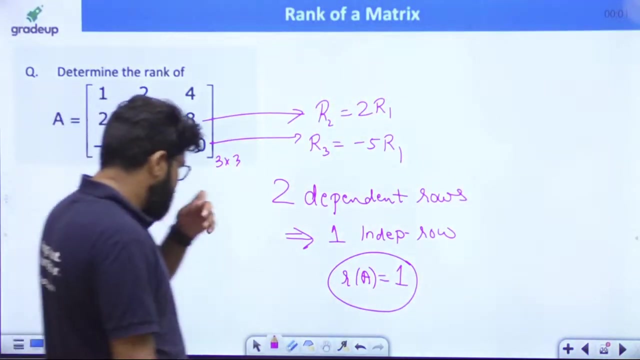 Three cross three is the matrix, Three is the number of rows, So three minus two, Only one independent row, and rank is equal to number of independent rows of the matrix. Answer is one. Answer is one. Yes, Synchronous academy that we can take up in any of the theory sessions. Right now I have planned the practice session, So that is why I have not gone into any of the theory, Right. 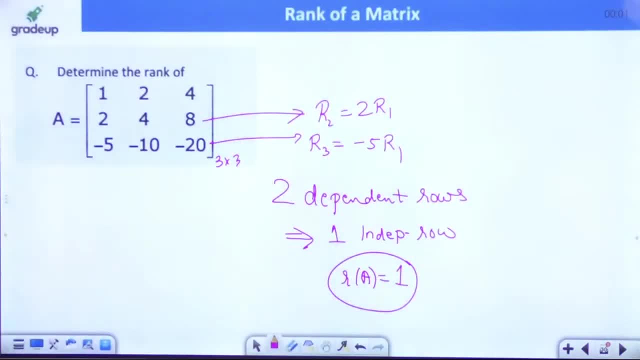 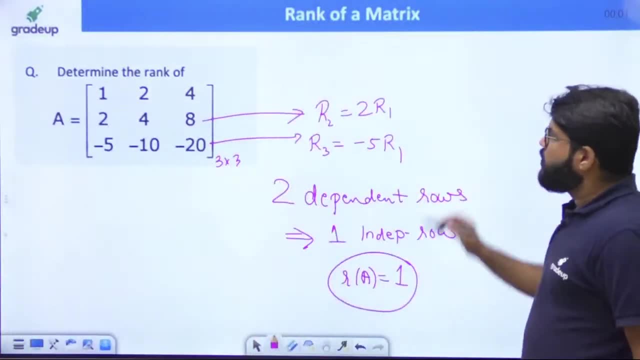 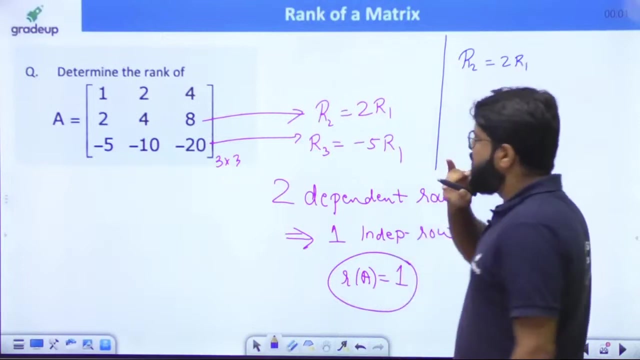 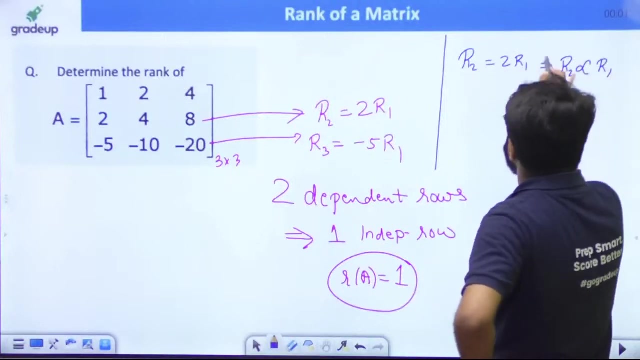 Chalo. So rank of the matrix Is equal to the one Got it. Now let's make a general conclusion here. In general conclusion, What you are able to see here- Okay, What you are able to see here- is R2 is 2R1.. Okay, Right, R2 is 2R1.. That means that means R2 is proportional to R1. It is just like KR1. Similarly, R3 is minus 5R1.. KR1.. So R3 also proportional to R1. 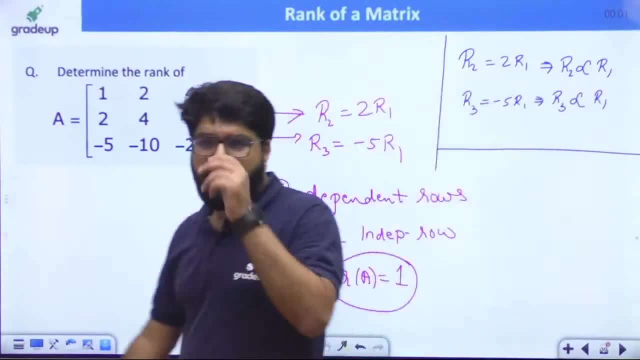 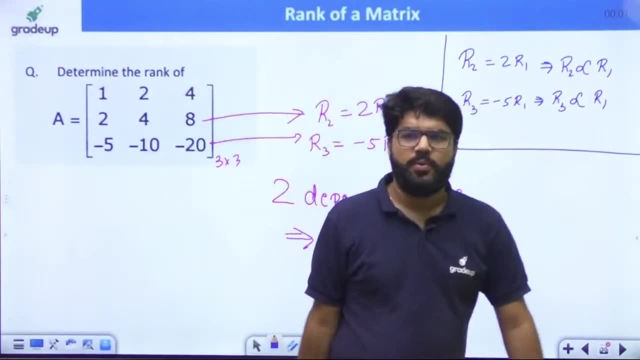 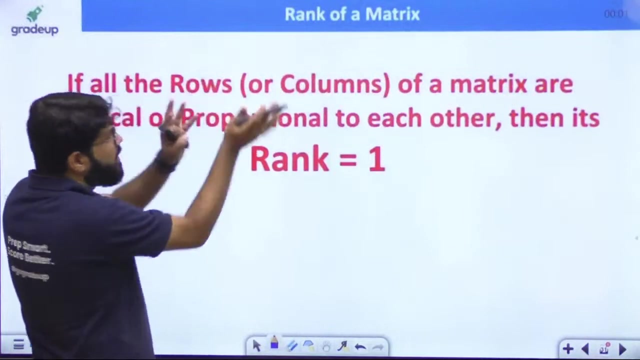 That means all the rows are proportional to each other. Right, All the rows are proportional to each other: R2 proportional to R1.. R3, also proportional to R1.. So, whenever the rows are proportional, If all the rows or columns Either rows or either columns. 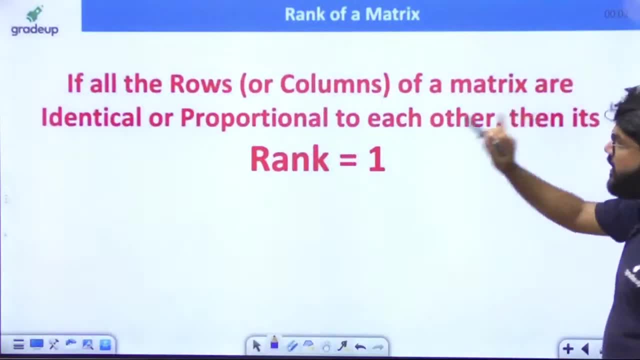 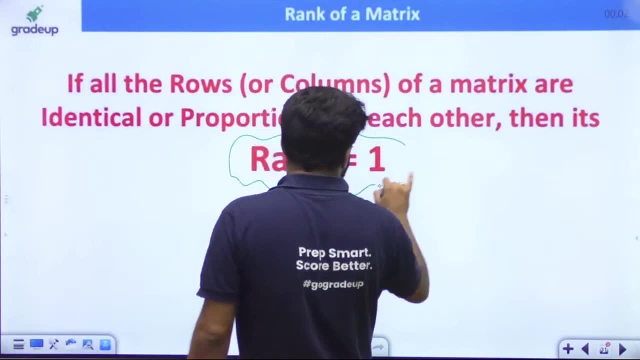 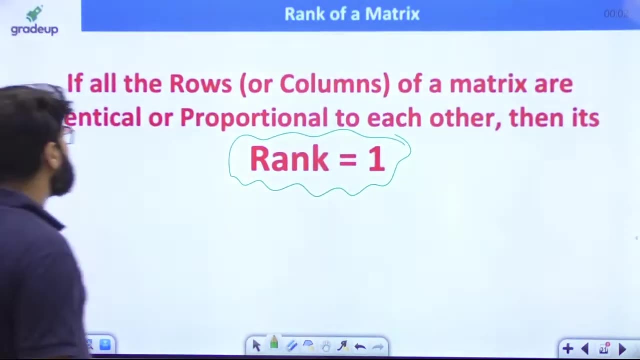 If all the rows of a matrix are identical or proportional to each other, then its rank is always equal to one. Rank is always equal to one. Let's take it as a very simple method: Whenever all the rows are identical or proportional to each other, then the rank of the matrix is always equal to one. 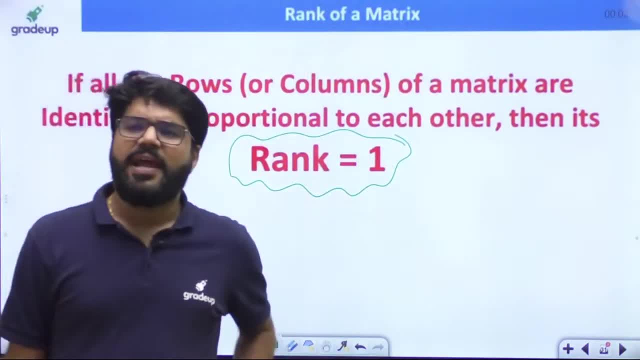 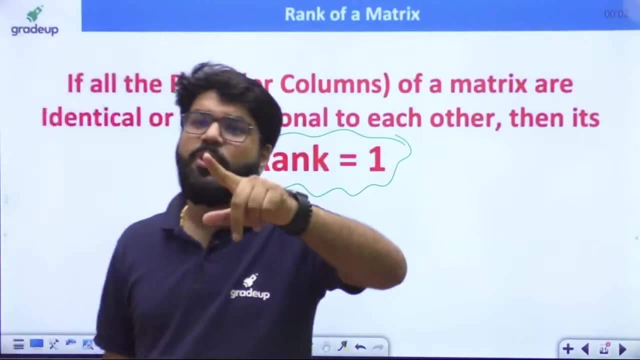 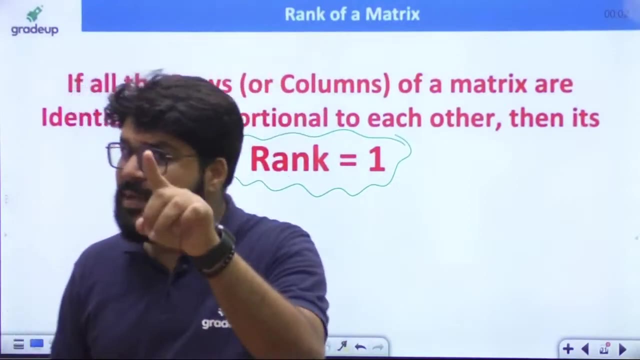 Chalo Suchi asks: Can a rank be zero? Yes, Yes, Yes, Venu, That's correct. With that point I am going to relate in the eigen value. So we have eigen value practice class. Okay, Rank is equal to number of non-zero eigen values. There is an exception to this property, Venu. 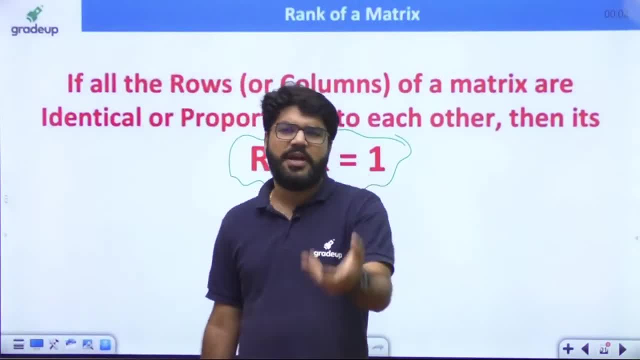 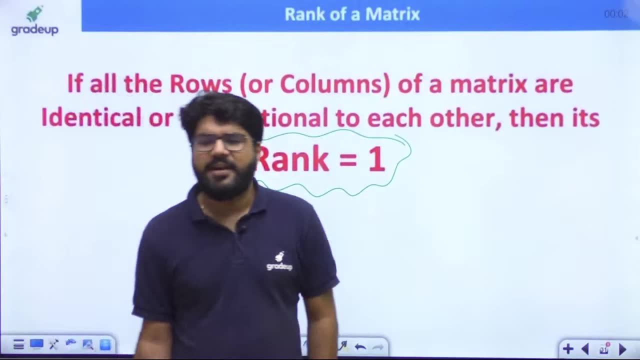 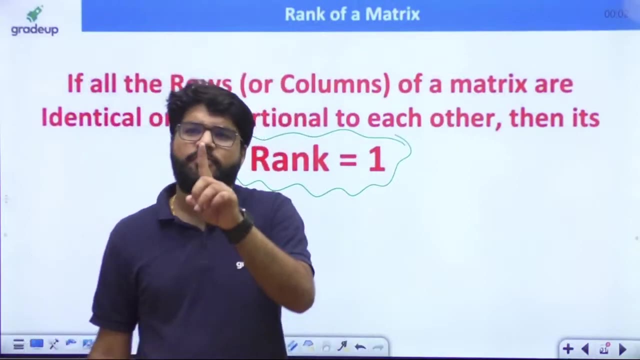 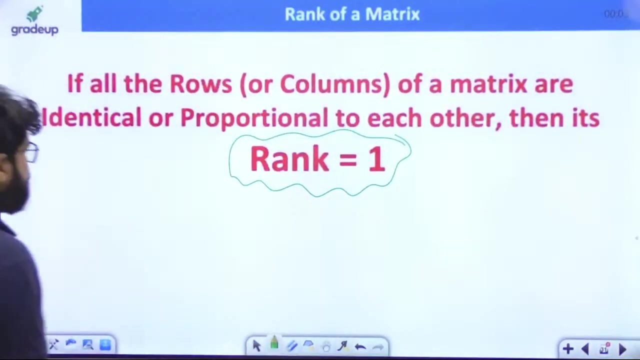 So you can follow that class on Friday. Friday and Saturday we will have, Okay, Friday, we will have Friday, and Saturday we will have the eigen value practice classes, Right? So Suchi is asking: can a rank be zero? Yes, It can be zero, but it can only be zero for a special type of matrix, For a special type of matrix. What is that matrix? Yes, Can you answer this, Chalo? 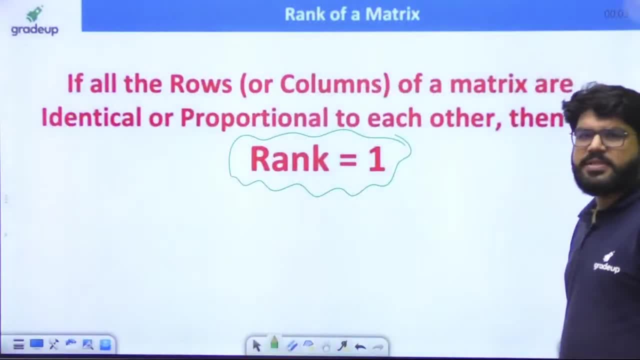 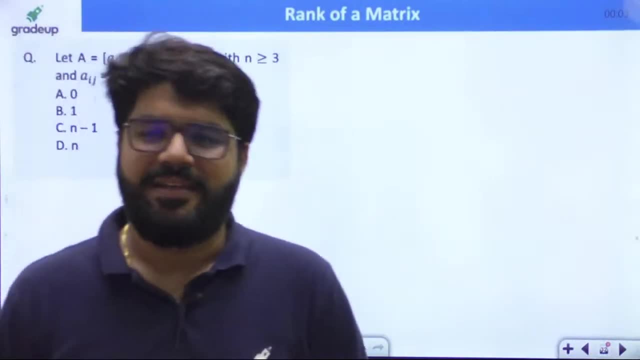 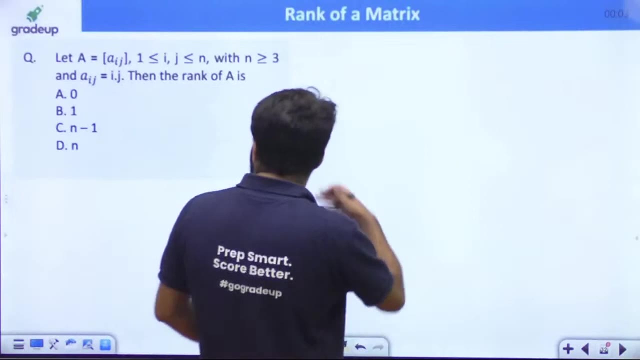 So let's take another question here. Let us take another question here. Yes, rank is equal to zero. right only and only for null matrix. okay, only and only for null matrix. rank is equal to zero. let's complete this questions and then i will write down. 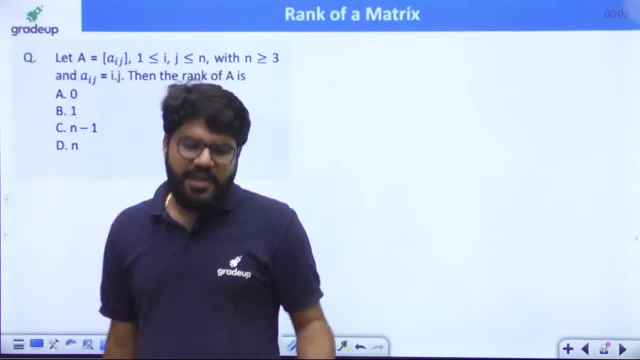 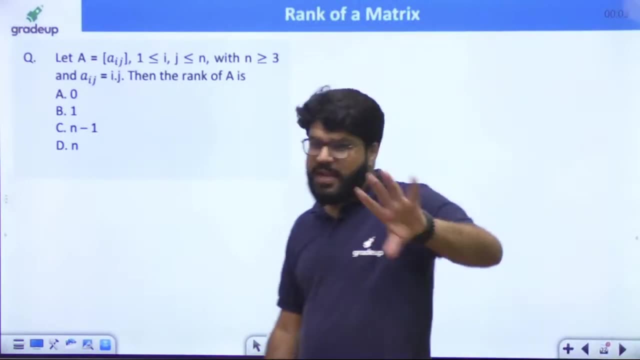 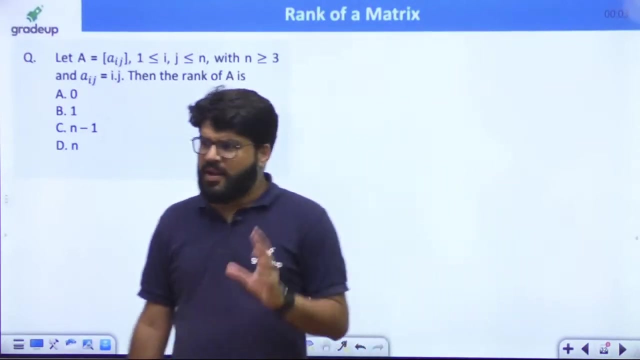 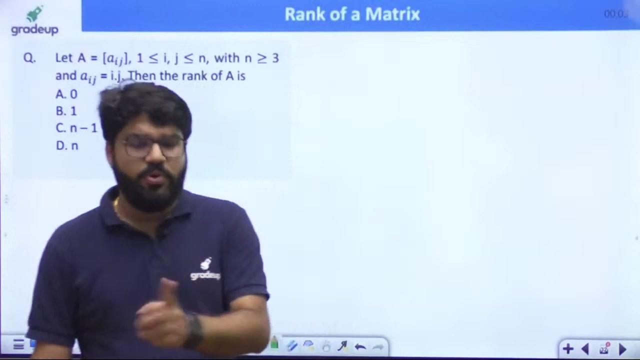 this class is daily till saturday. okay, 51 most expected questions and i will make it 51, don't worry, 51. so it will be minimum 51. it can be little bit more, but we will not go for less than 51 around 8, 10 questions. so i think. so, don't worry, 51 most expected question series and we are going. 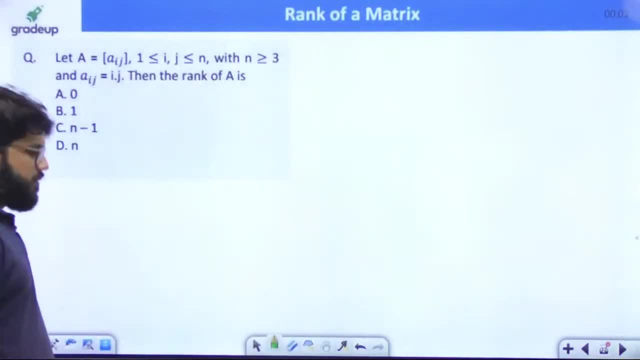 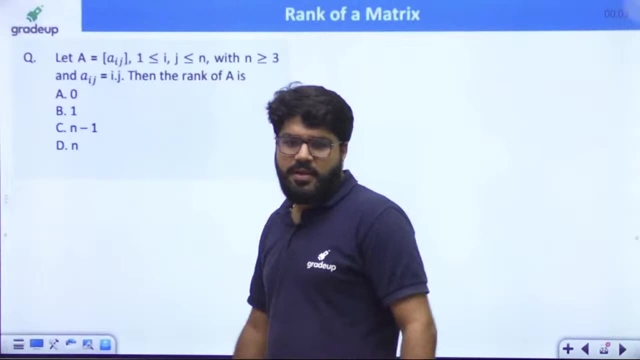 to go till saturday. yes, what should be the rank of the matrix? a. what should be the rank of the matrix- and this is a language based question- okay, if a is equal to a, i, j, where one less than equal to i, less than equal to j, less than equal to n. 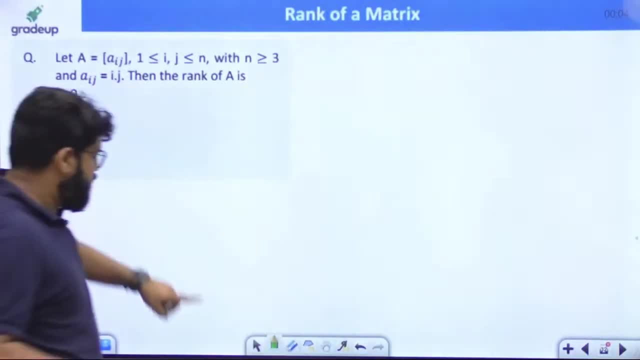 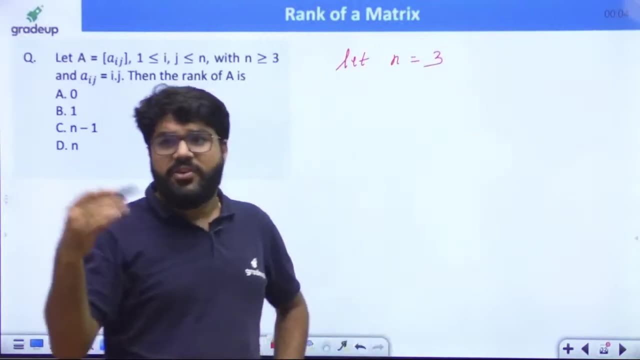 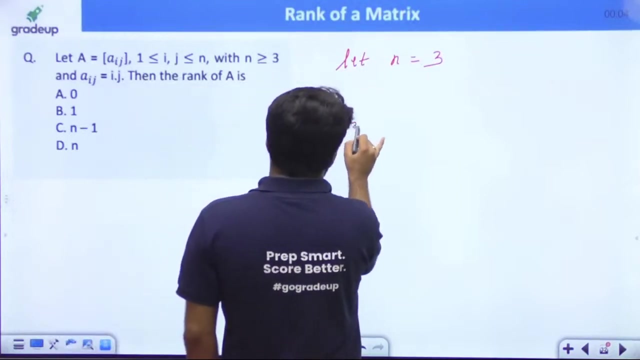 within greater than equal to three and a i j is i into, j okay. a i j is i into, j okay. n is greater than equal to three. so let's take n equal to three. just try n equal to three, right, let's try n equal to three. so what is a matrix? it becomes a three cross, three matrix. and what is the three cross? 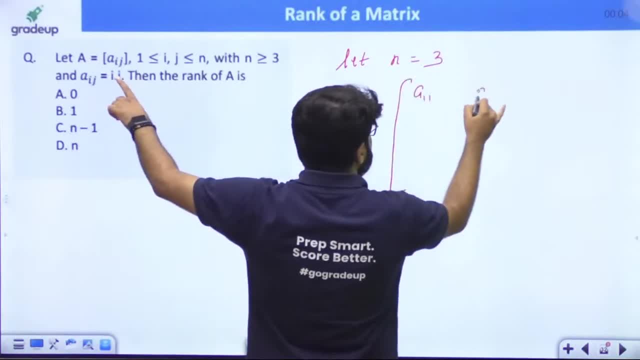 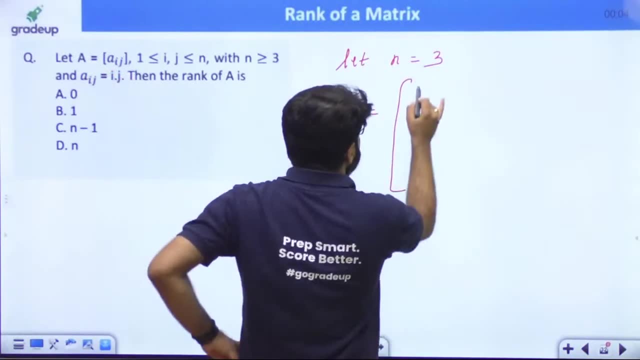 three matrix: see a i j. we should know this is a one one, a one two. but every element is the product of the coefficient i- j. so what is a one one? what is a 11 is one one into one. what is a 1 to 1 into 2? award 3 is 1 into 3. then 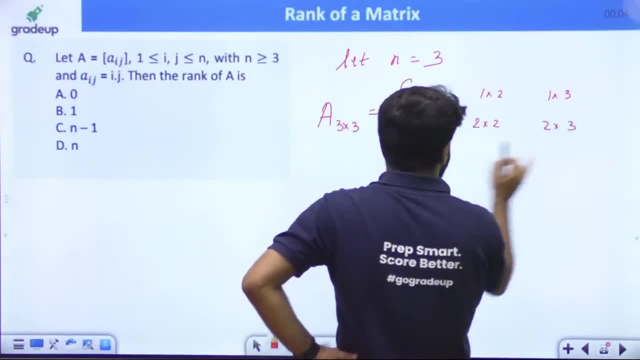 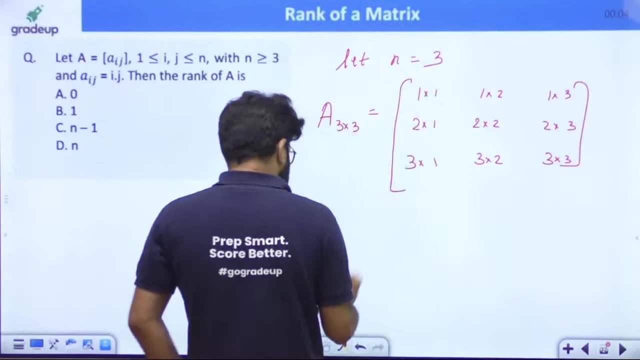 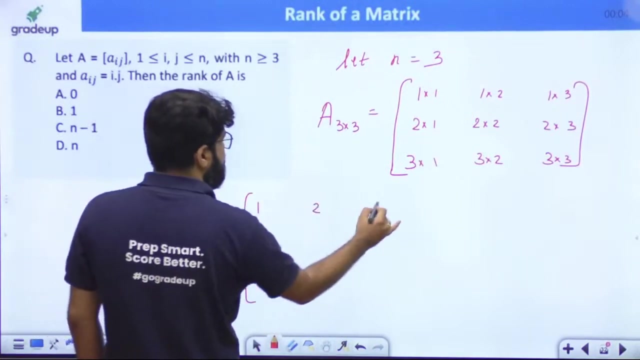 a 21, 2 into 1, 2 into 2, then 2 into 3, then third row, 3 into 1 a, 3 to 3 into 2 a 3, 3, 3 into 3, everybody. this is what should be the matrix a. okay, so what is the matrix a actually? okay, one, two, three, two. 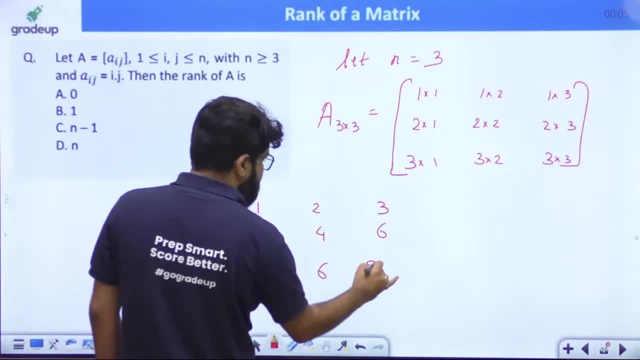 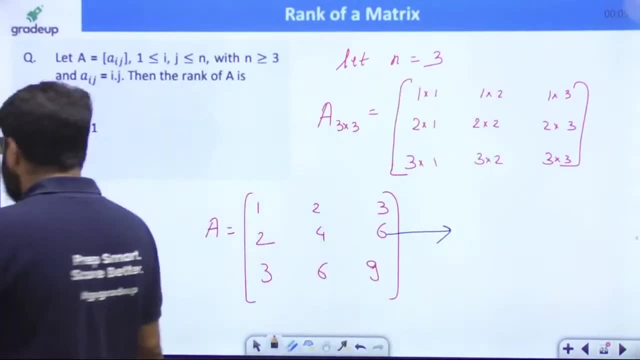 four, three, one, two, three, four, three, two, three is the nine, three, seven, eight, eight, three is a 10. okay, now see just the dependencies in front of you. just see the dependencies in front of you, right, one, twos are two, two, twos are four, three, twos are six. so r2 is double of r1. 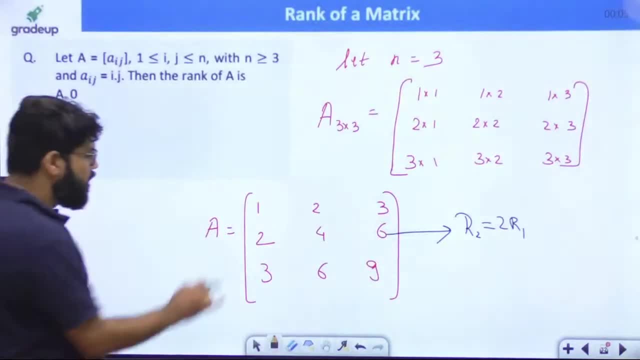 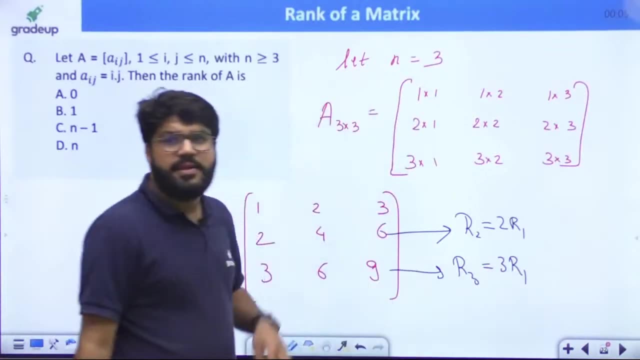 r2 is double of r1. next one: three is a three. two, three is a six. three, three is a nine. r3 is three, r1- got it. r3 is three, r1- got it. r3 is three, r1- right, so all the rows are proportional. 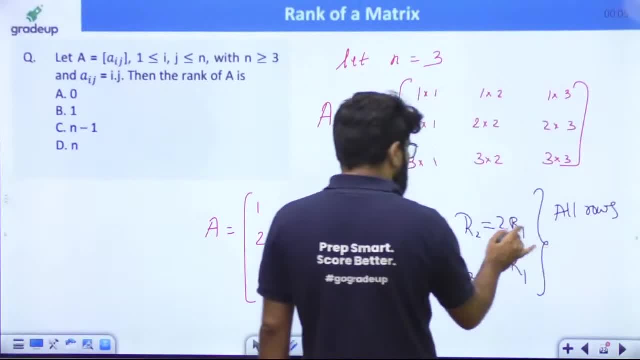 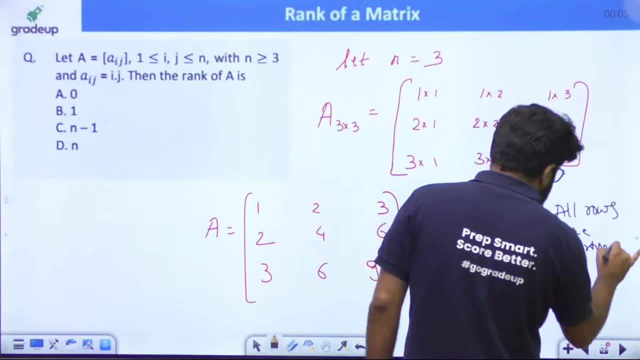 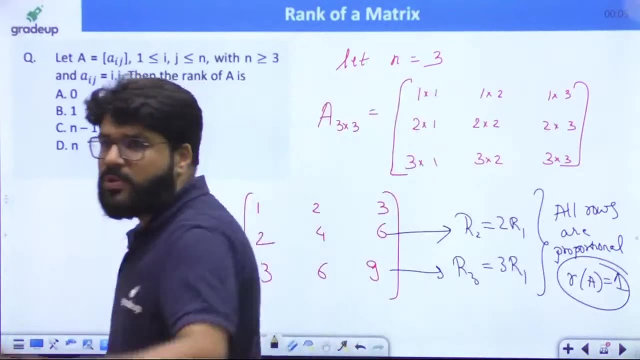 to r1. all the rows are proportional to r1, r3 proportional to r1. all all the rows are identical, or i can say, proportional to each other, and whenever that is the case, rank is equal to one. so the answer is equal to one, rank is equal to one, even if you try for fourth order matrix. 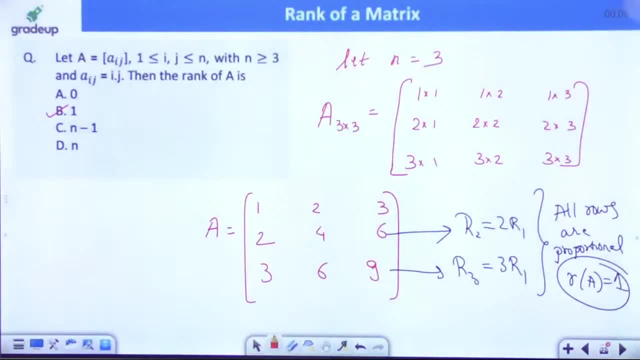 it will be one. it is one. answer is b. answer is b: bhat badiya. bhat badiya. answer is b. yes, i'll conduct more practice question sessions, don't worry. right rank is one: bhat badiya. yeh samajh mein aana chahiye. these are. you know, these are typically expected questions. 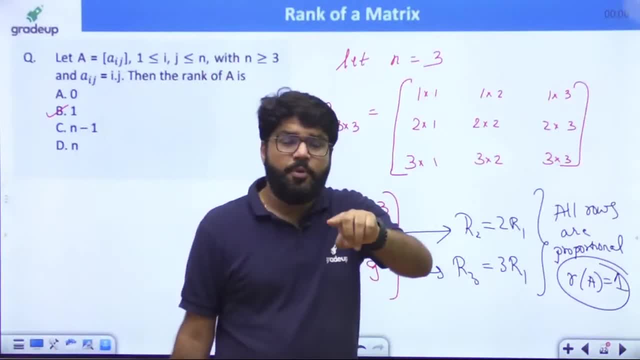 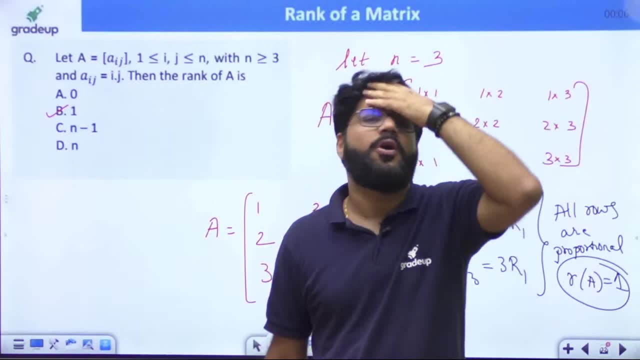 yeh ban raha hai. toh rank se sab kuch banega. and guys and guys, very important point, whatever concepts you are learning today, agar yeh trick samajh mein aagya, then the next topic, non homogeneous system of equation- tomorrow also will be very tricky and very easy for you. 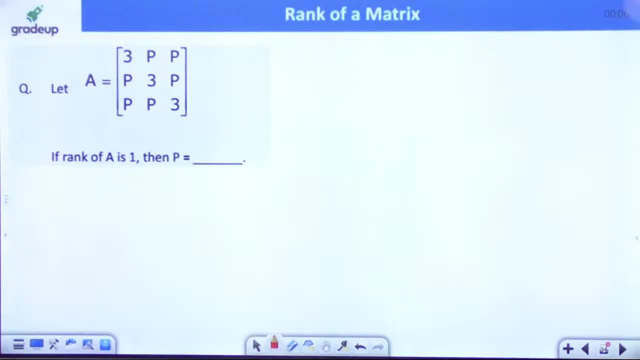 that will also be very tricky and easy for you. if a is three, double p, p three, p, p three. if the rank of a is one, then what is p? if there rank of a is one, then what should be the value of p? right, toh dekho ya pe kiya bolah hai. 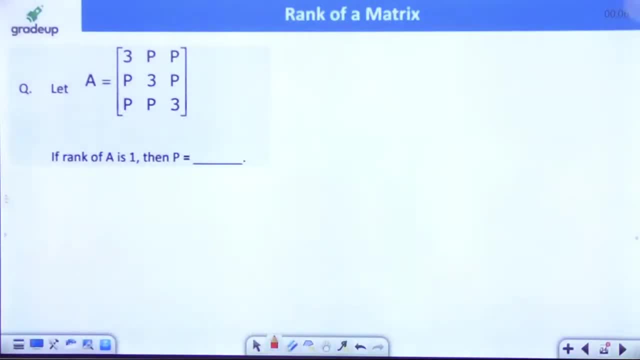 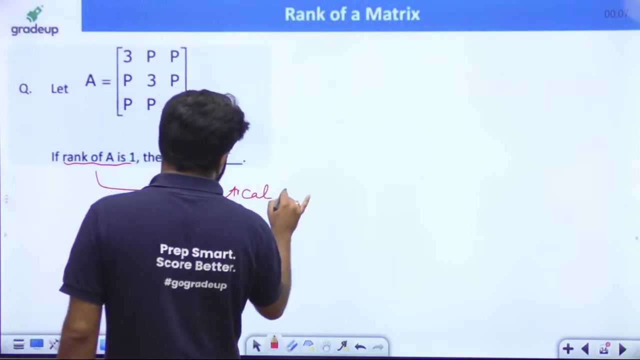 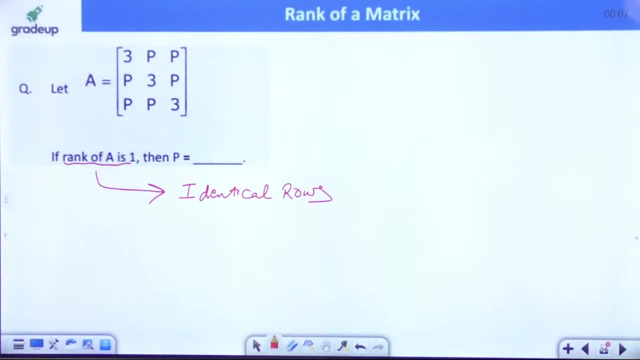 this should be a simple question. can you try out? thank you, pk. can you try out if the rank of the matrix is one? sir, if the rank of the matrix is one? thank you, pk. ok, rank is one. matlab: you should have identical rows or proportional rows. okay, and yes, yes, PDF will be there with you identical rows. so how I can make it. 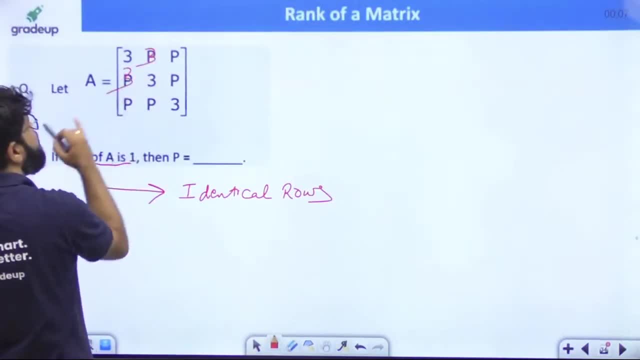 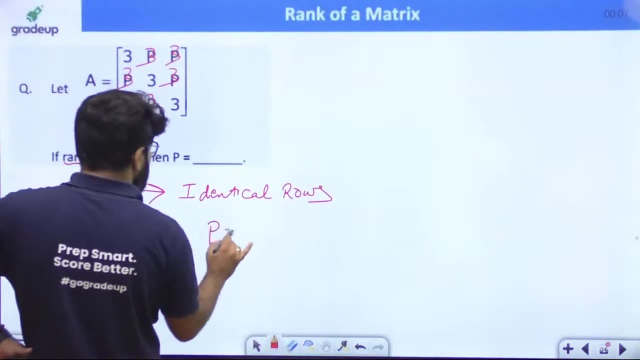 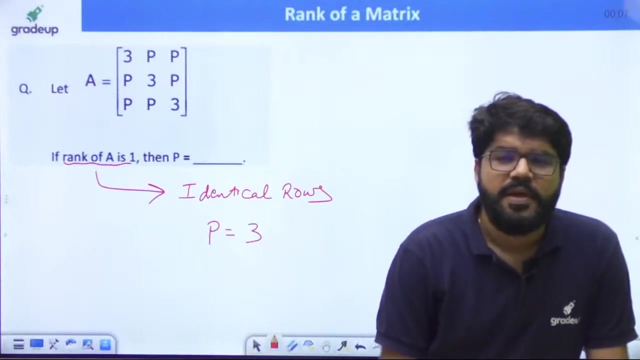 identical. yeah, happy, happy, happy, happy, happy three. so let's try p3. if P is 3, all rows are same. all rows are same, okay, so the only possibility is equal to 3. finished, just a simple guess of the answer, right? a simple guess of the. 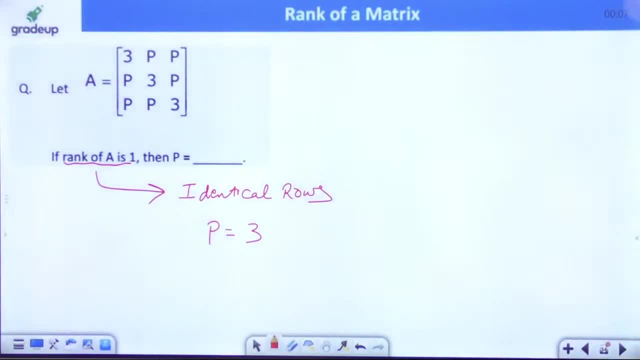 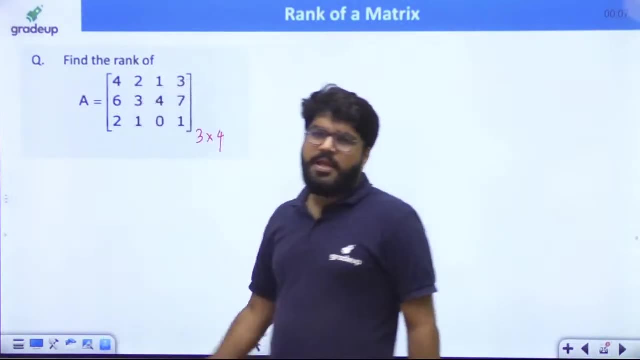 answer. answer is three. but he is in a boat, easy, a bay had easy. I am very easy, very easy. now a 3 cross, 4 non square matrix. many people will straightforward go for echelon form I, although I have cleared every method I will give you. 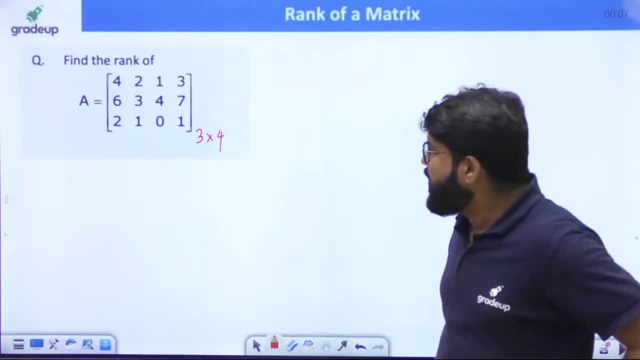 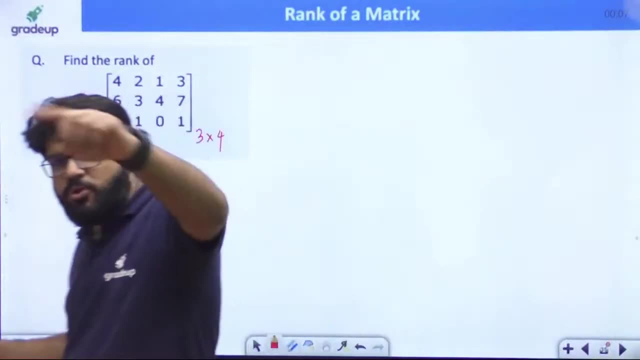 every method, don't worry. method mess up a Duga. so many people can directly go for the echelon form, can go for the echelon form, but do I need the echelon form or can I try with something else? this is up to you. please try and comment. 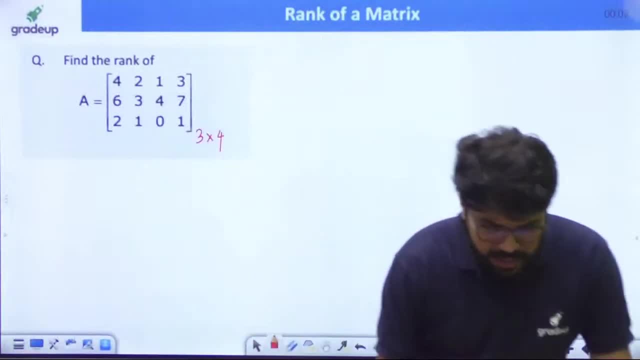 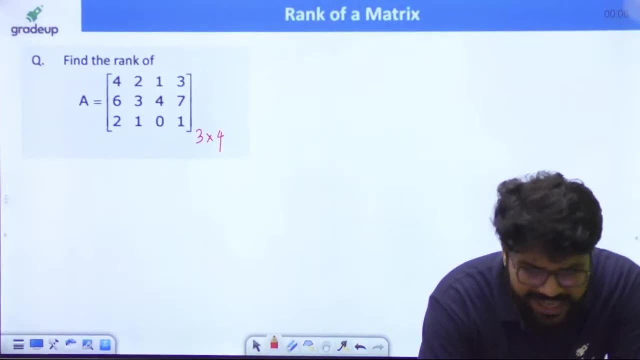 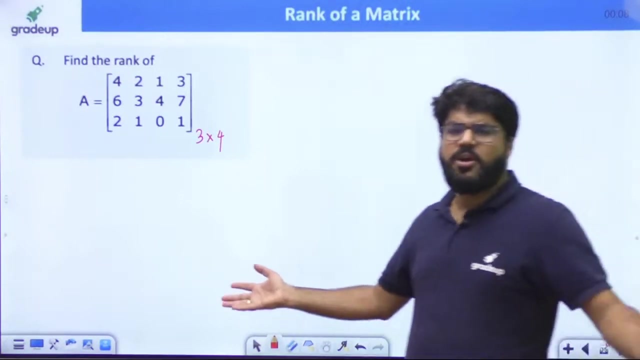 on the answer, everybody. 3 cross 4 non square matrix. 3 cross 4 non square matrix. do I need to go for the echelon form or can I give my answer very, very easily without any echelon form? think you tell me. you tell me the answer, guys. that's what? whether it is lengthy or not, your call Satyami. 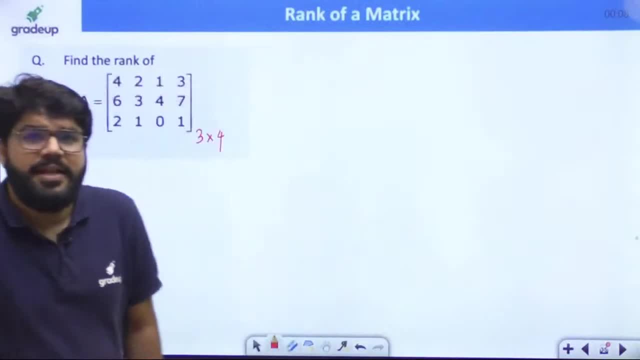 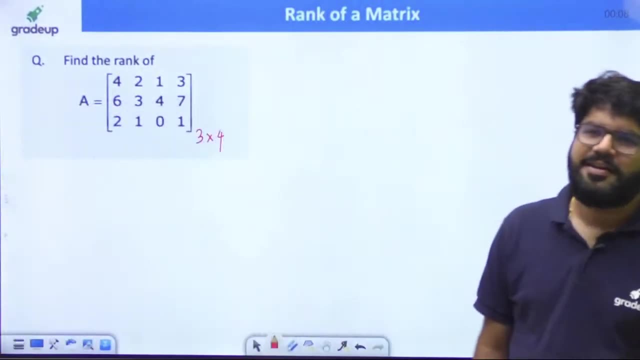 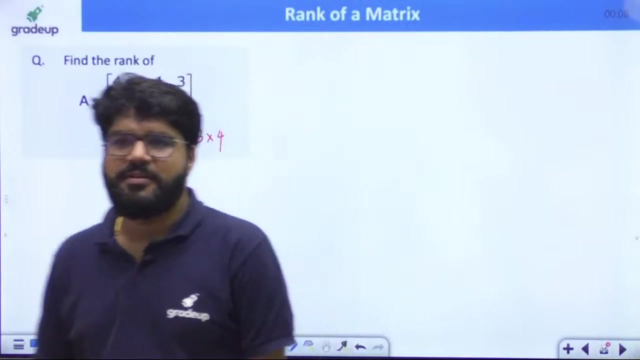 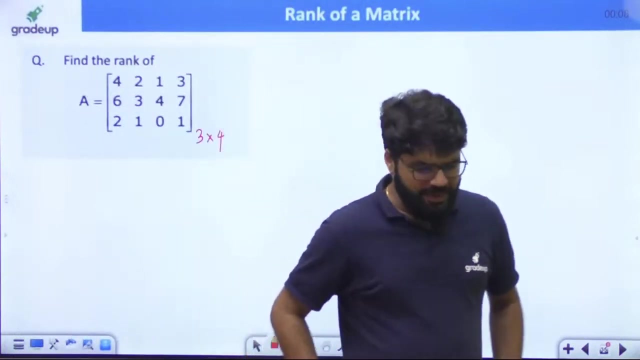 me. let me see whether you are able to get the answer and, if at all, how you are able to get the answer. that is more important. that is more important. yes, guess, aiga, echelon form I know will be little in the I know echelon form I can. 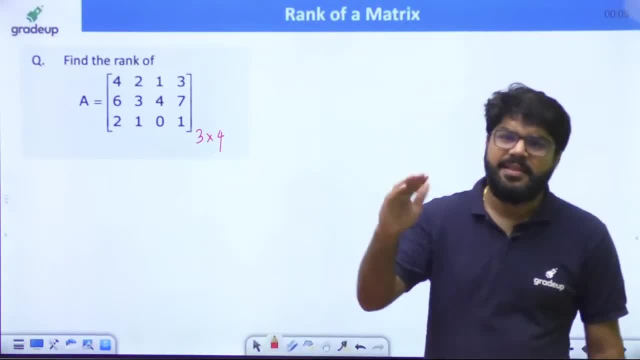 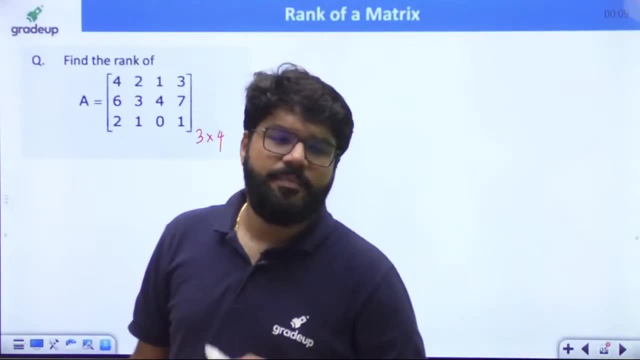 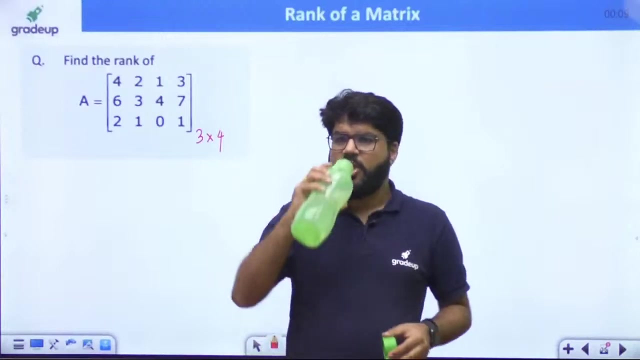 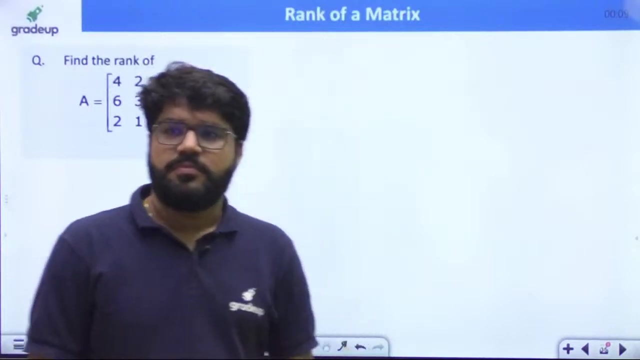 convert into a clean, not difficult. echelon is not difficult but it can be been a lengthy. if you need to convert into echelon it can be lengthy. so three and two, three and two mix are in a click or opinions are coming up as mix. mix. opinion are a three versus two, three versus two- sorry methods with our 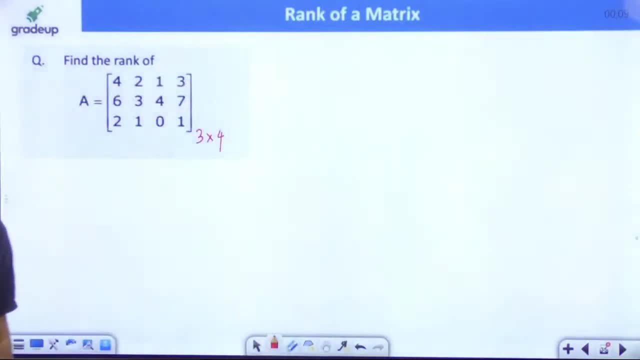 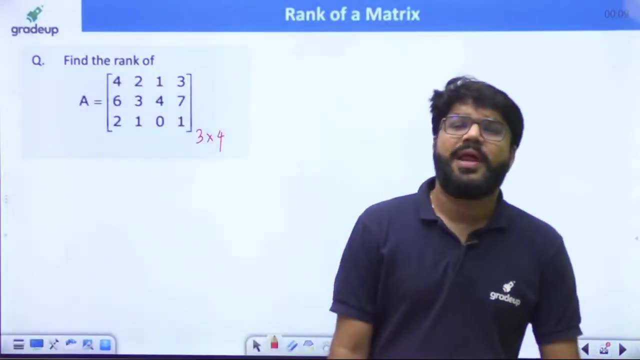 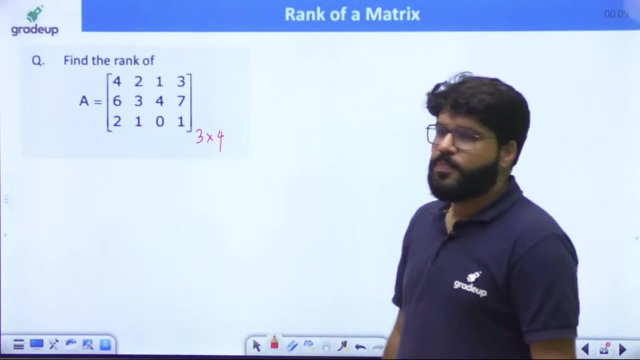 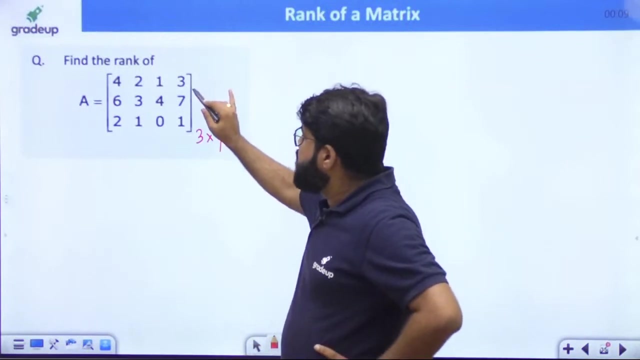 libraries. But so what it is. so check that they, check that they. so that is as I told you. rank is equal to number of nonzero rows, our number of nonzero columns. deco, deco. you may listen to the very important words. so my bull gonna put keem ap noche. it would be very important words, you may. 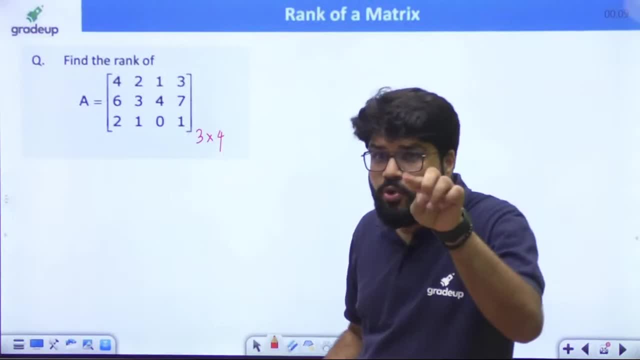 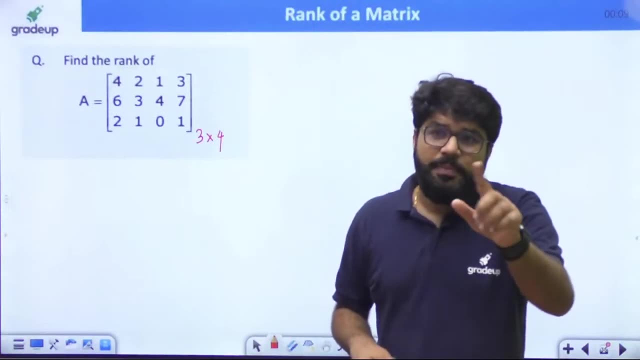 not be able to find any dependency in the rows. you, you, I am talking about you, you, you. you are not being able to find any dependency in the rows. you, you, I'm including me. also take a. I'm Barbara, I don't worry, you may not be able to find. 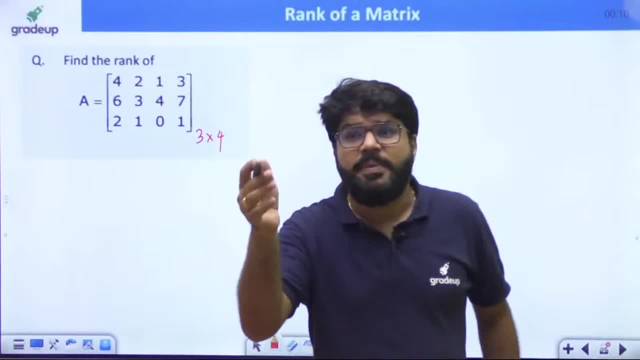 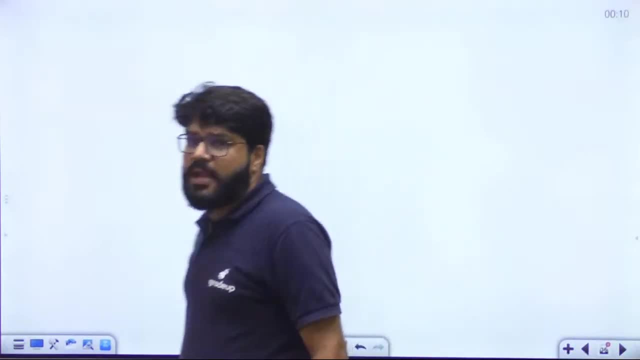 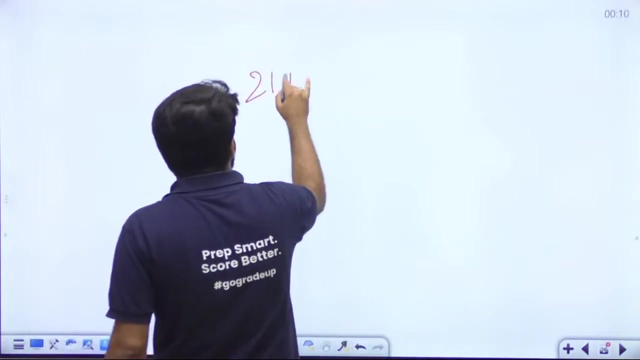 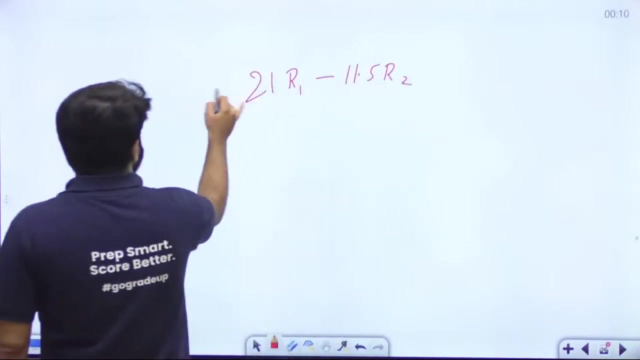 may not be able to find the dependency in the rows, it does not mean that the rows are not dependent by a subito host, a. sometimes the dependency can mean, sometimes a dependency can mean something. you know some absurd dependency by: suppose 21 R 1 minus 11.5 R 2, 11.5 R 2 is equal to 14 R 3 below by: 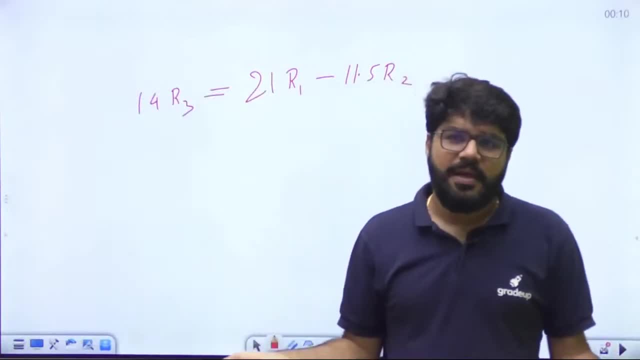 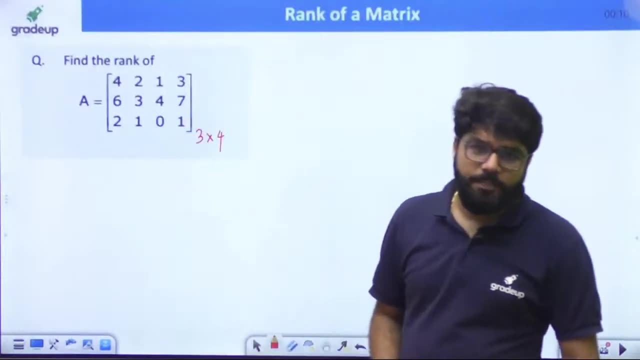 this is also a dependency. this is also a dependency by getting my point. so what I am telling you? listen to my words again. sometimes you may not be able to find row dependency directly, but it does not mean that rows are not dependent host at that dependent to our. 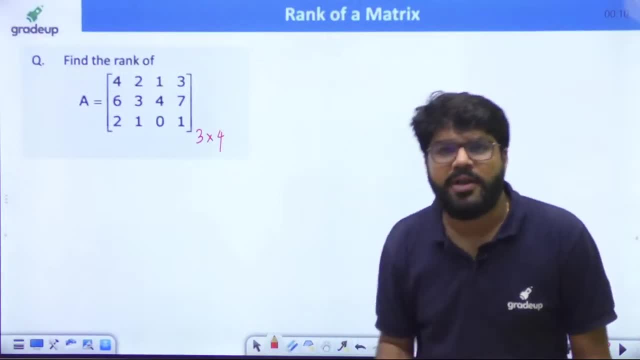 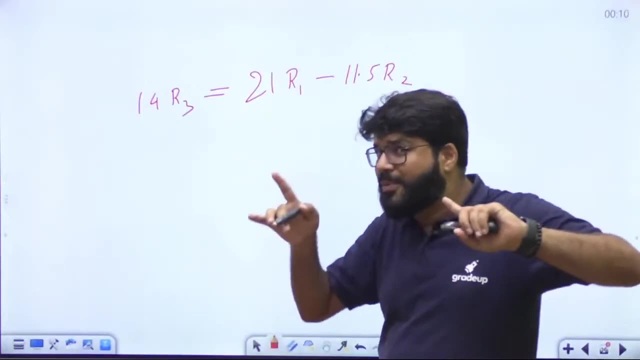 concluding us at the host, at the NIO. maybe may not be. you are not able to find. there may be some complex dependency or there may not be. there may not be. I'm not telling. there is a dependency, there may or may not be, but you can't conclude. okay, can I think with column if I am not able to search with? 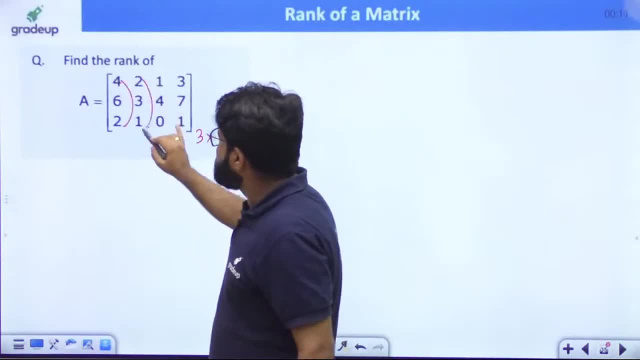 rows. okay, they come equal. a grata: 4 plus 2 is 6, 2 plus 1 is 3. but you have a logia: 1 plus 0 is not 4, 3 plus 1 is not 7. the row dependency. I am not able to. 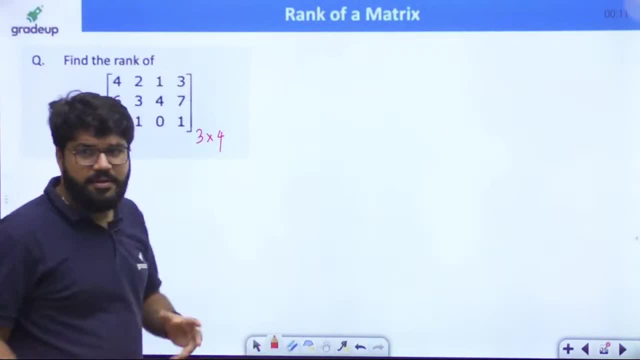 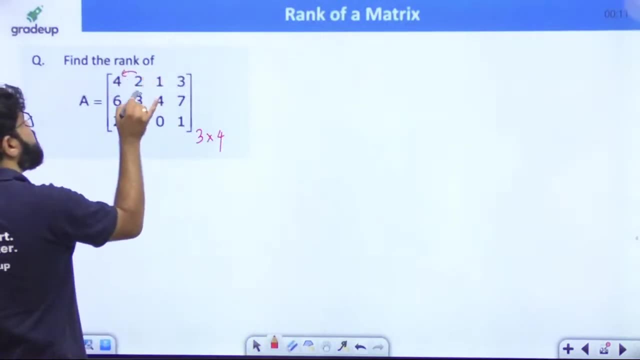 find. if I am not able to find does not mean that dependency, Nia, okay, can we try column, can we think column the andlett, anybody, everybody to, does a 4, 3, 2 0, 6, 1, 2, 0, 2 once 2 2 0, 4, 3, 2 0, 6, 1, 2, 0, 2, right, so I am able to see that whenever. 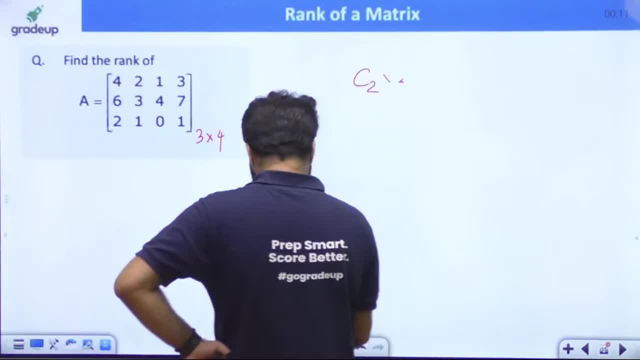 I take the column number 2 X to worry. I take the call. hurry board is skipping the words. huh, I think 12, 11 am. one board is going to such a dangerous route to hit it. hmm, do most of the time this type of a non-statistical term goes. so which is on up cross? I'm sorry. muse and all a bunch of other older examiner like my brother. so much you have to put my brother's name too over and I was streaming. you do not do anything's still and let's just waste all this and attempted phone call. the problem is now broadcast, flashing the intense text and the 에 and I was shocked by this glass: absorb the world. it all makes sense. 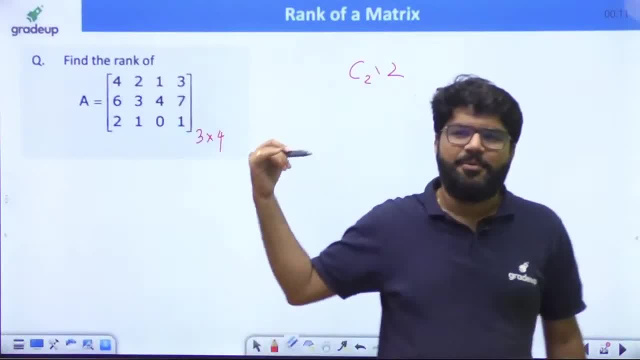 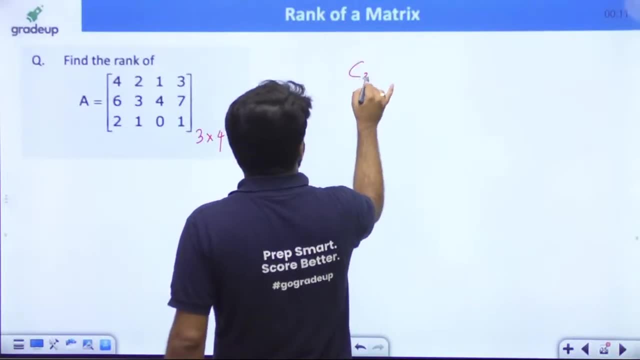 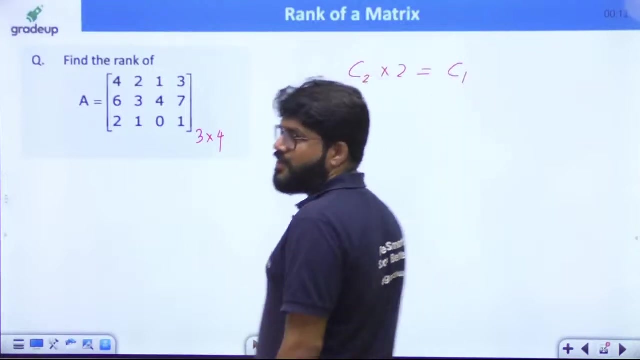 is tired. I am not tired. my students are not tired. board is not tired. Okay, Board is tired. Okay, board is a little tired. Since morning 11 am it is running, So sorry what I am writing- C2, when it is multiplied by 2, I get the C1.. By the way, he is also tired. 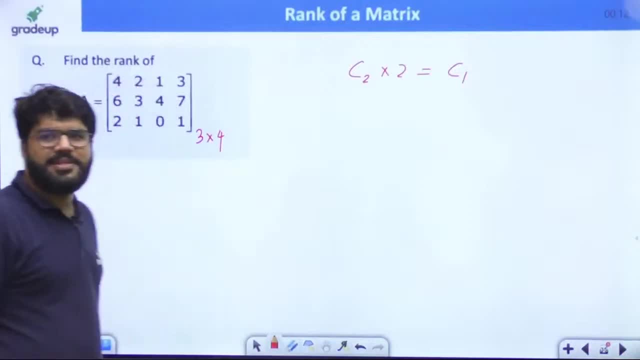 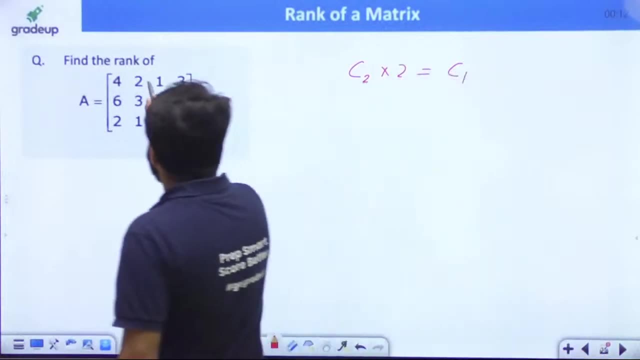 He is also working hard. since 11 am. C2 into 2 is equal to the C1.. Right, This is one. Any other, Any other, Any other Sir, search? 2 plus 1 equal to 3.. 3 plus 4 equal to 7.. 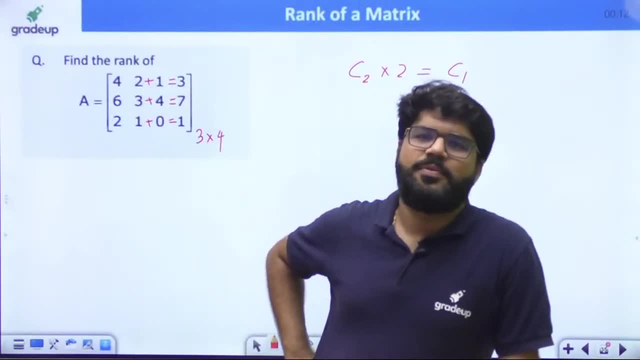 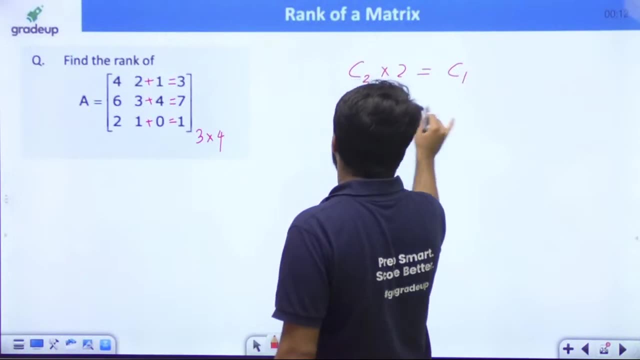 1 plus 0 equal to the 1.. 1 plus 0 equal to the 1.. Right, So I can write down that when I add column 2 and column 3, I get column number 4.. I get the column number 4.. So one. 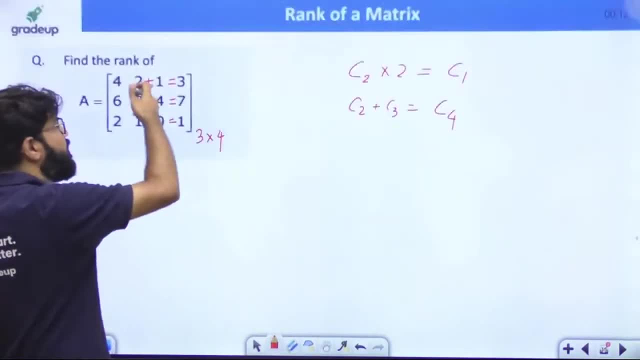 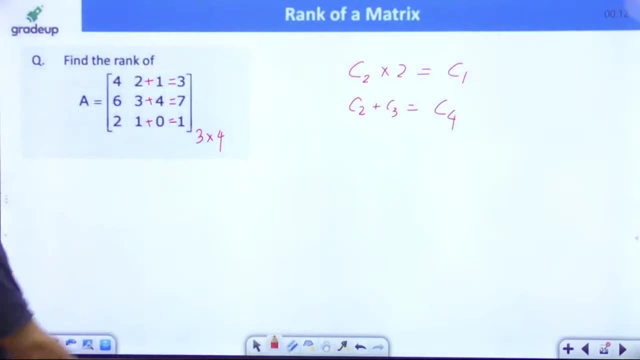 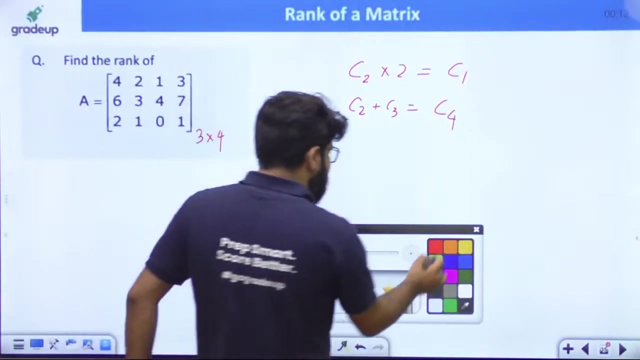 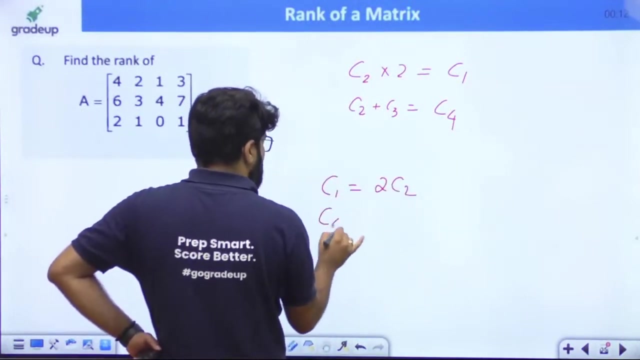 more easy dependency. It is not any absurd, not random, It is a very easy dependency, Very easy Dependency. It is a very easy dependency, Right, Easy dependency. So what I can say is what I can say is column number 1, twice of column number 2.. Column number 4 depends. 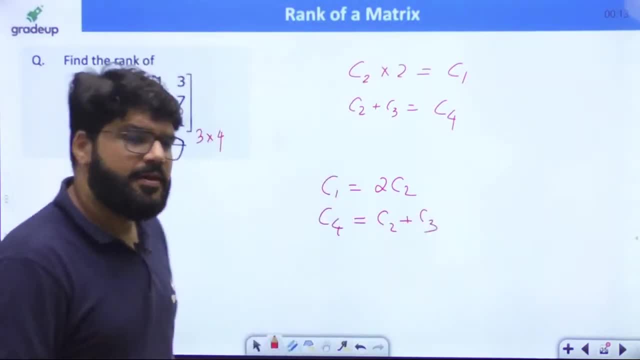 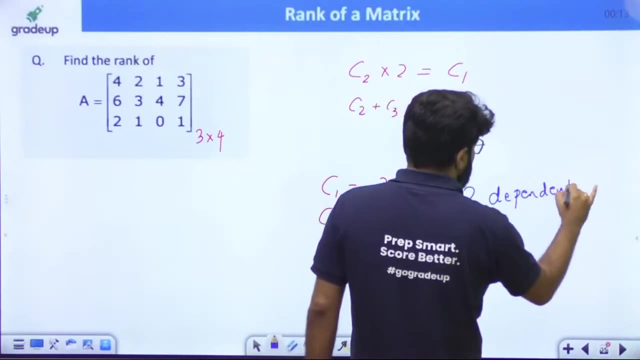 on C2 and C3. So there are two columns which are clearly dependent. There are two columns which are clearly dependent, Two dependent Columns. There are the two dependent columns, Right? So how many independent columns? I don't want dependent, I want the number of independent columns. So how many Out of? 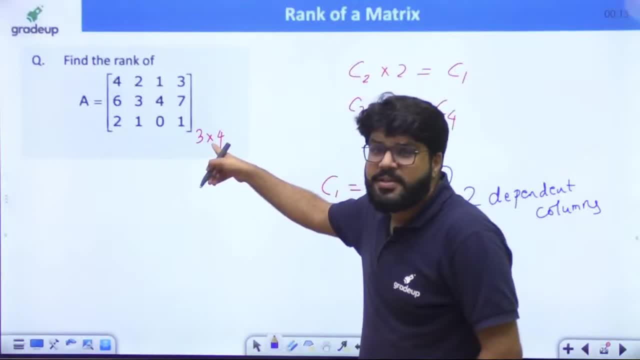 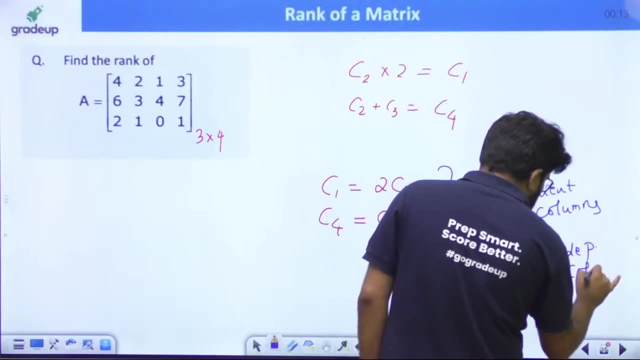 the four columns: Columns 3: nahi hai. Columns 4: hai. It is a non-square matrix, So 4 minus 2.. 4 minus 2.. Independent columns: 4 minus 2.. Kitna hua 2.. So the rank of the matrix. 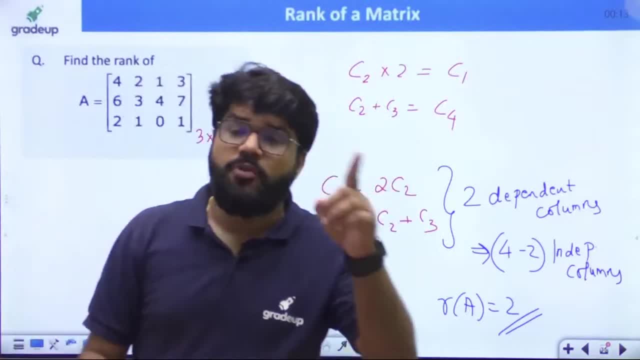 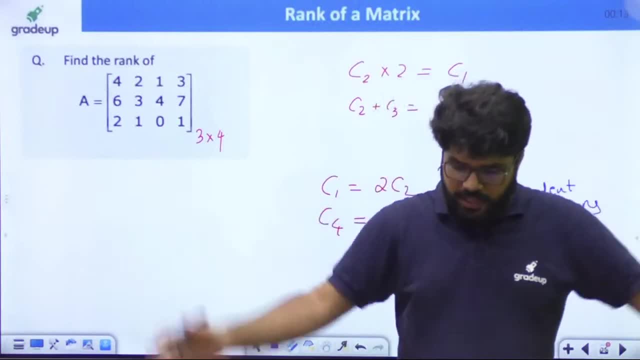 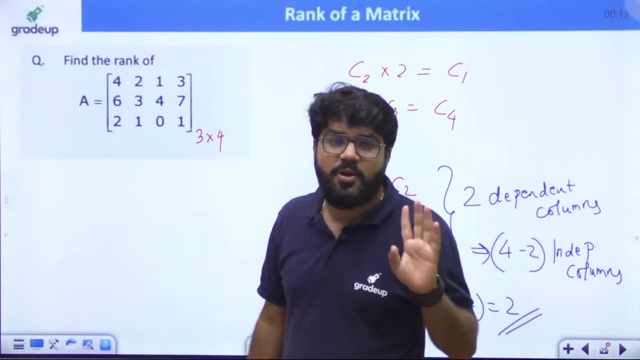 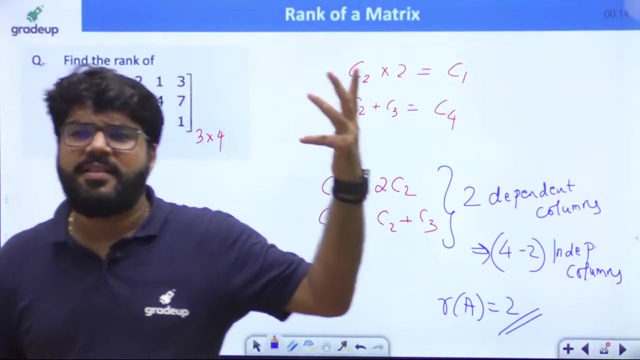 number of non-zero independent columns. Okay, Once again I repeat: Maybe we were not able to see the dependency in rows. It does not mean that the rows are not dependent Acha, If the rank is 2.. If the rank is 2.. If the rank is 2. Determinant, toh nahi niklega 3. 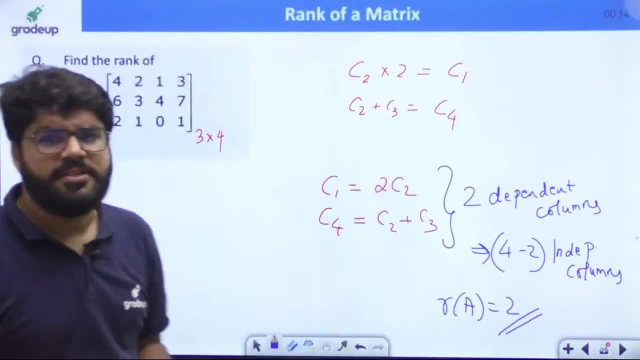 cross 4 matrix se kano gula. But yeah, you can find out 3 cross 3 minus. But again, wo lendi hoga? First you take this 3 cross 3 minus, 100% dependent. But again you can. 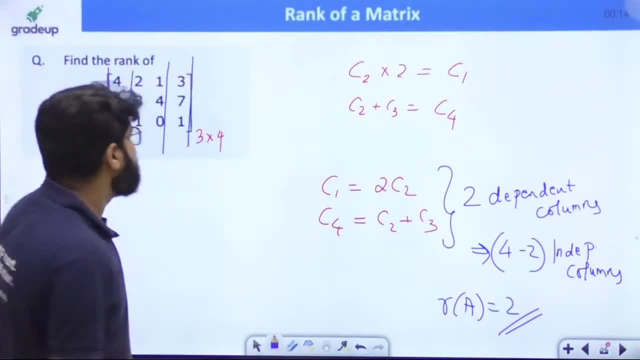 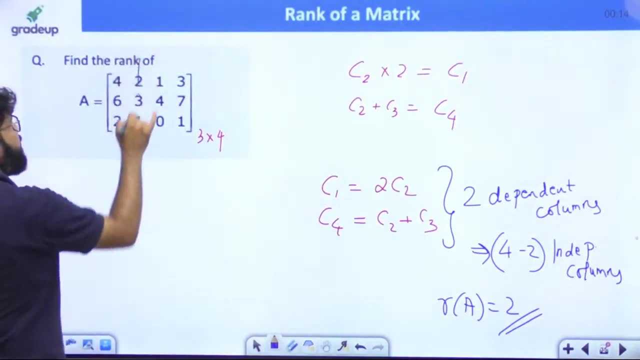 0 Shiva. Then you take this 3 cross 3 minus, That is also 0. Okay, So there will be 4: 3 cross 3 minus. Okay, First delete this column, Then you get a 3 cross 3 minus, Then delete. 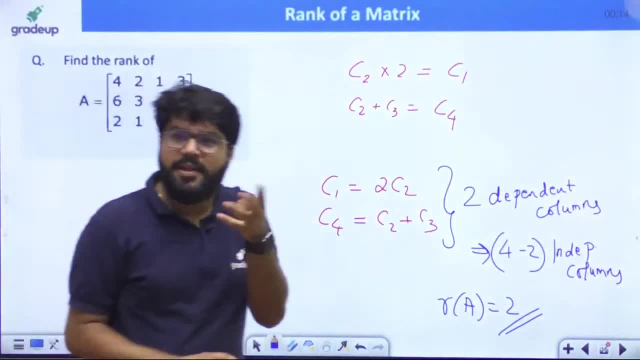 this column Again a 3 cross 3.. So like that, 4, 3 cross 3 minus, and confirm all 4 will be 0.. Then you will try 2.. Toh lendi hoga na, Shiva Kumar, Lendi hoga Acha What I was. 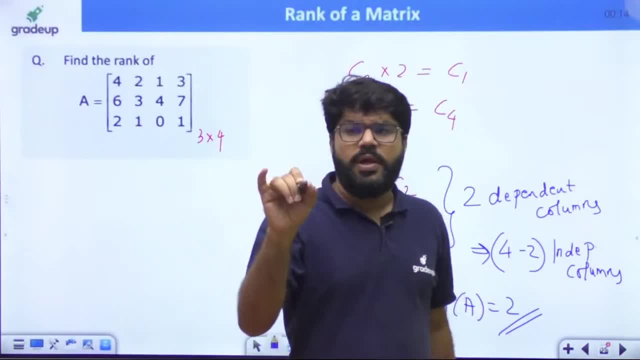 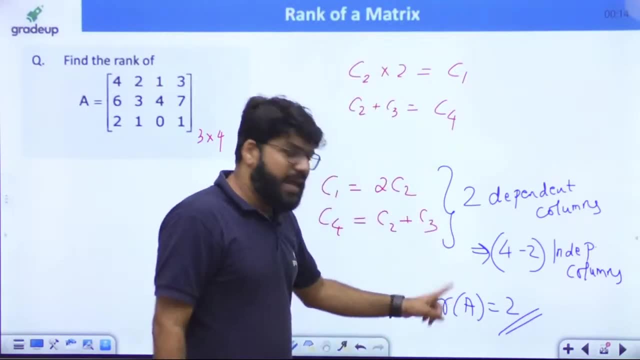 telling is ki rank is 2.. And if rank is 2, there will be confirmed 2 dependent rows. So there will be confirmed 1 independent- Sorry, I am sorry, Slip of tongue. Rank is 2.. So there will be confirmed 2 independent rows. So there. 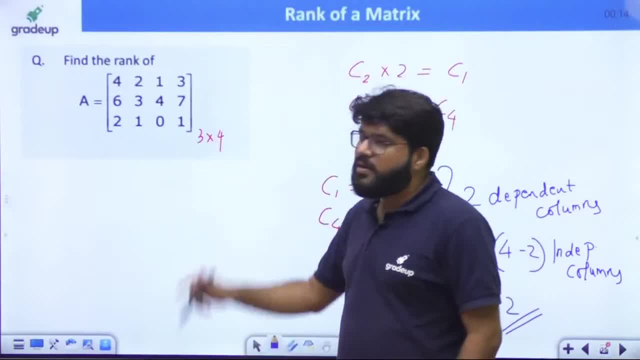 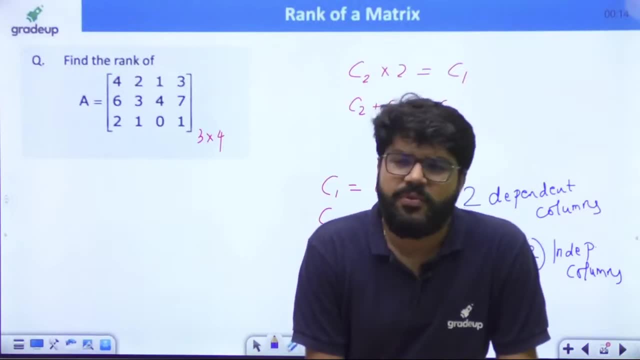 will be confirmed. 1 dependent row Right: There will be 1. confirmed. There will be 1 confirmed dependent row. Aap search kar lena. You have to try it out, But let's not waste time into that. Okay, No problem, yaar Dekho PK. That's what our practice should be. I. 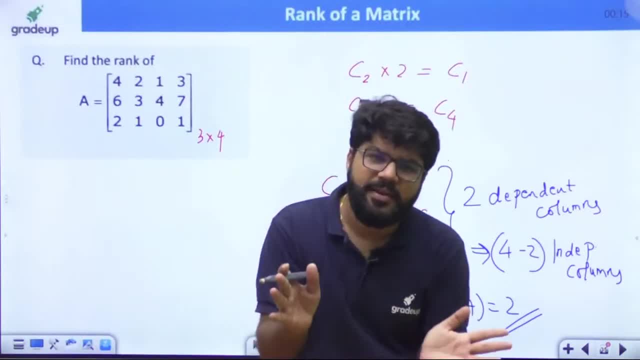 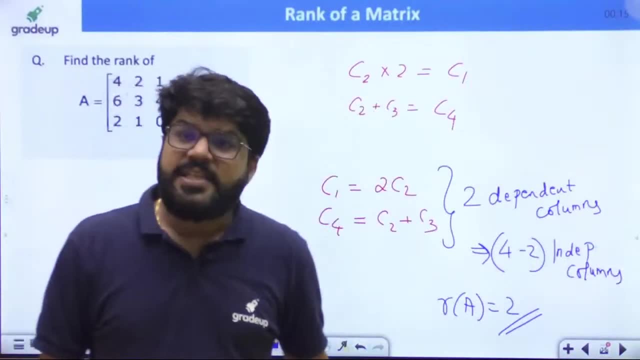 have shown you some very simple questions, Okay, In all our gate category Okay, And I have shown you some good questions And our practice should be broad, Easy to difficult, Easy to difficult. See why I told you echelon method, The reason. now I will explain you. 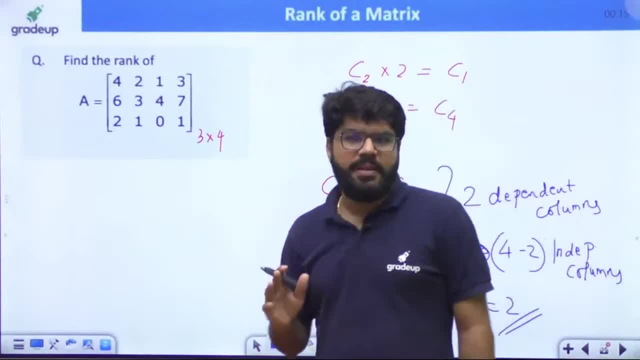 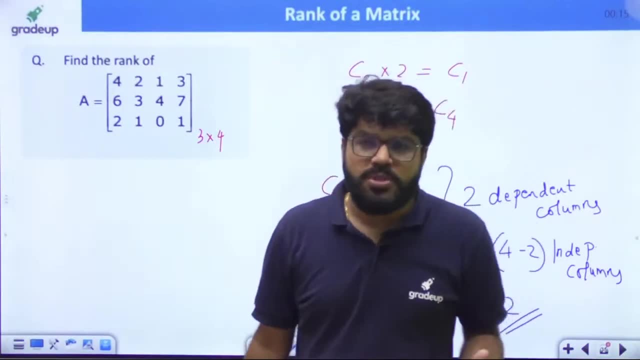 Why, in the beginning, I told you echelon method, Because it is a definite method. See, although these tricks are appreciable, These tricks are appreciable, This is what is: a simple trick of finding the rank. But suppose Aap hoga na yaar. You know how to find rank, But 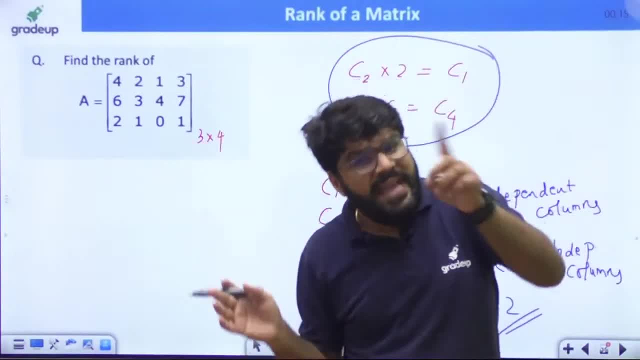 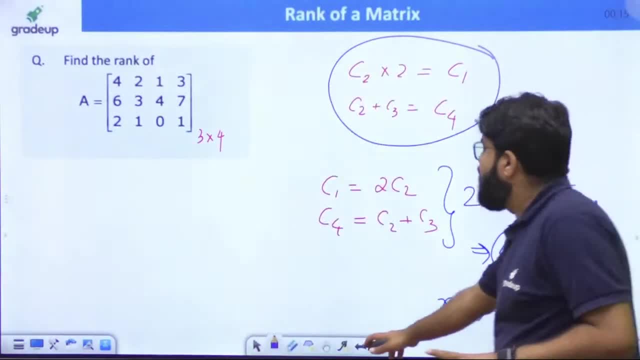 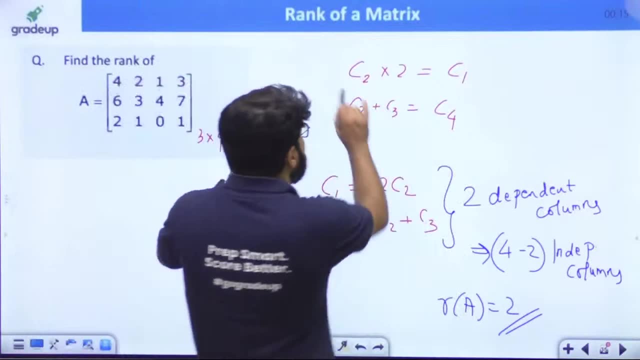 That is why I think you get now why I was stressing in the echelon form. Echelon form, if the matrix is already in echelon form, then it easy to apply, then it is easy to apply echelon. otherwise we have to convert into echelon. But imagine the situation ki agar. 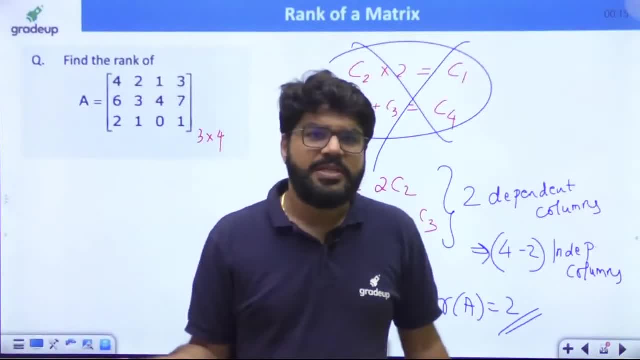 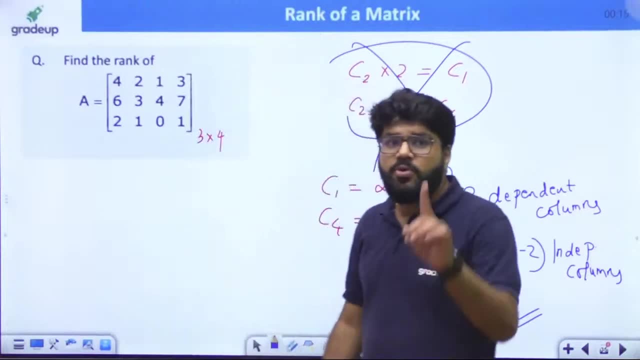 aapko yeh nahi mila. then you are stuck with the question, Or either you have to leave the question, But no, don't leave the question. Then try finally the echelon form. and you know what is the echelon form. You know what is the echelon form? Right, Right, So that. 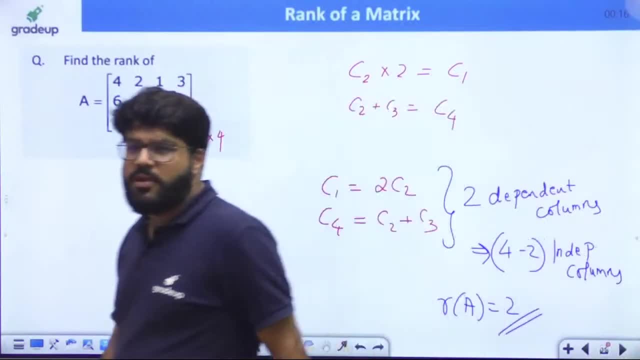 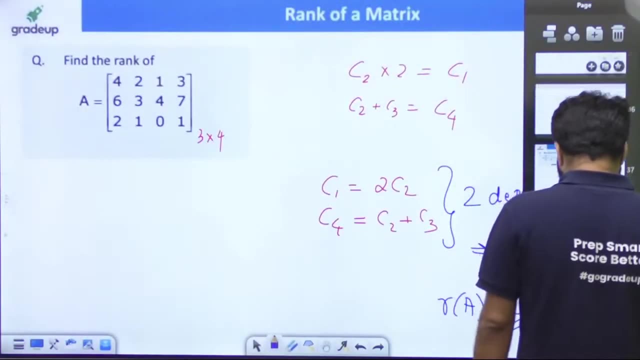 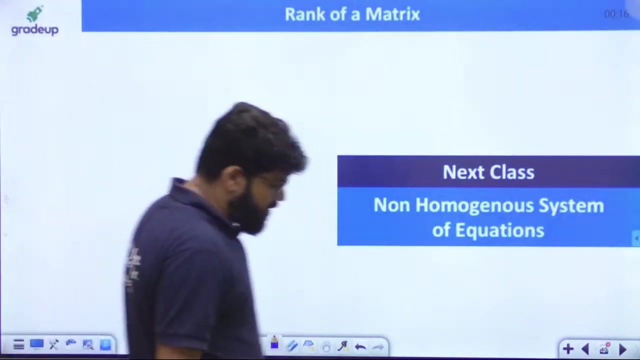 is what it is. Then you can go for the echelon form, Then you can go for the empty one, Can for the echelon form, everybody. then you can go for the echelon form, echelon, echelon, echelon, and then we meet tomorrow. see guys, non-homogeneous system of equation. i will tell you what is known. 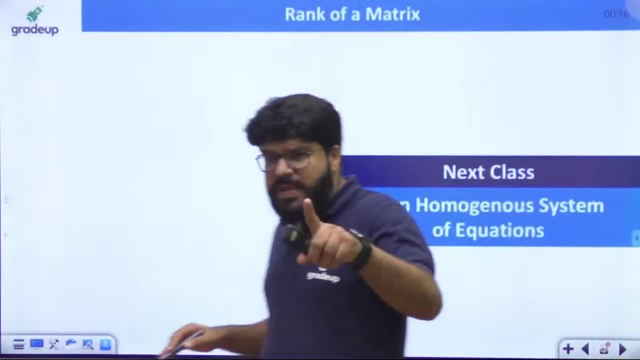 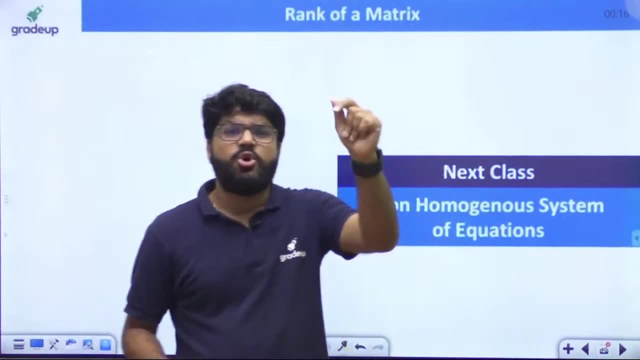 as rauch's theorem. i will take up questions based on this. but trust me, whatever tricks you learn today, i am going to even utilize the tricks in non-homogeneous system of equation and i will show you some gate two mark questions. i will show you some gate two mark question. two mark question. 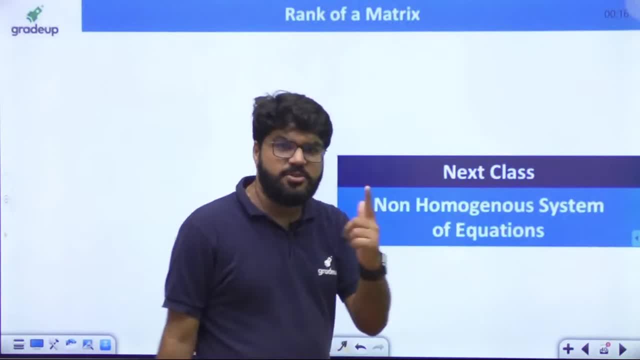 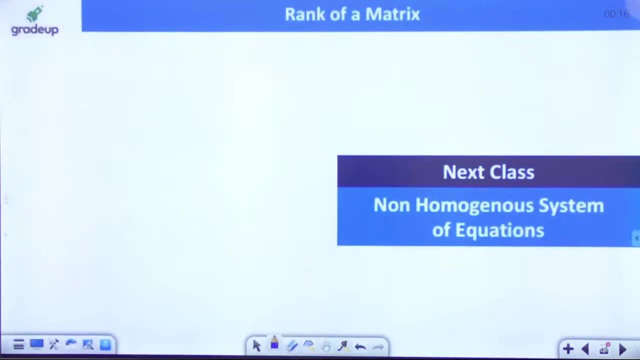 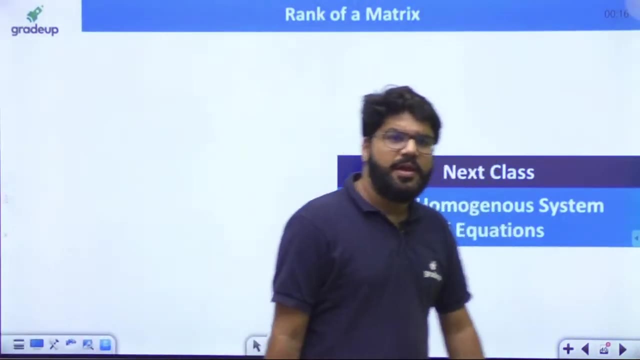 to be solved within this tricks. 10 seconds, 20 seconds. we can solve the gate two mark question. right, why, why? why, sunali, if you are able to confirm on dependency, then independence is also their total number of rows minus dependent rows. we can do okay. so, guys, one important update. 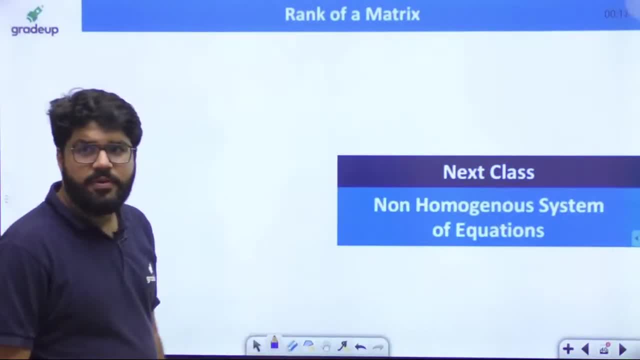 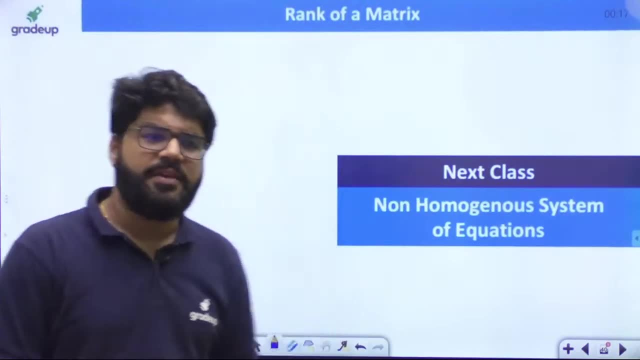 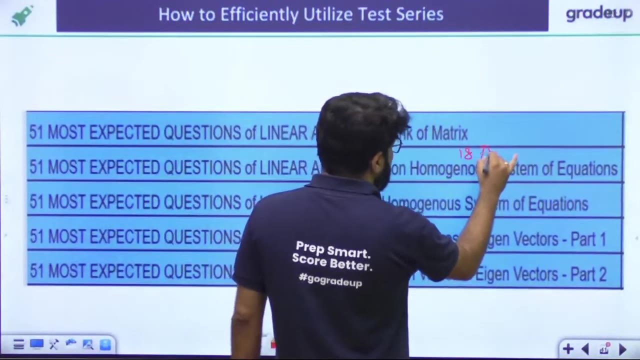 for you. okay, one important update for you. i will tell you right, you not not for all chandan, you know, because it is the time savior. it is the time savior. so, guys, let me tell you this is what is tomorrow. this is what is the sequence of the classes. this is tomorrow, 18th august, then 19th august. 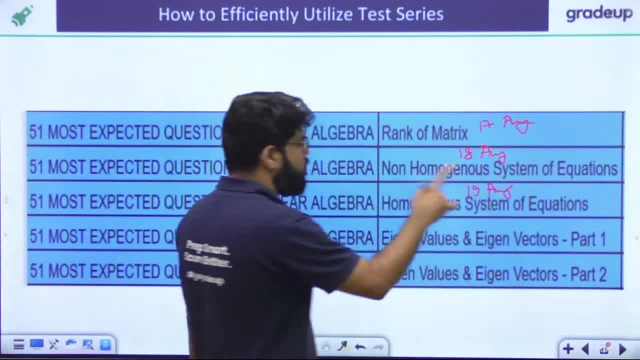 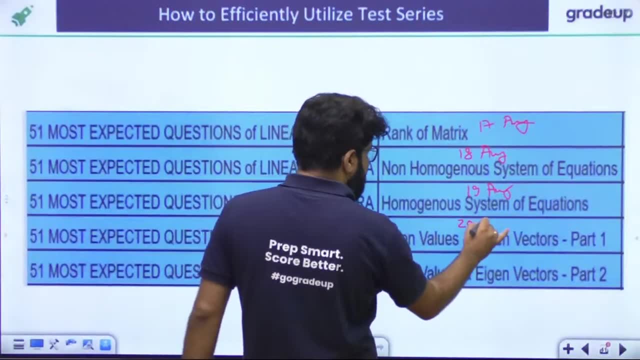 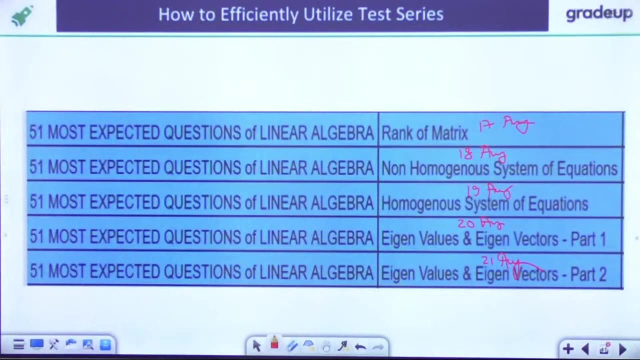 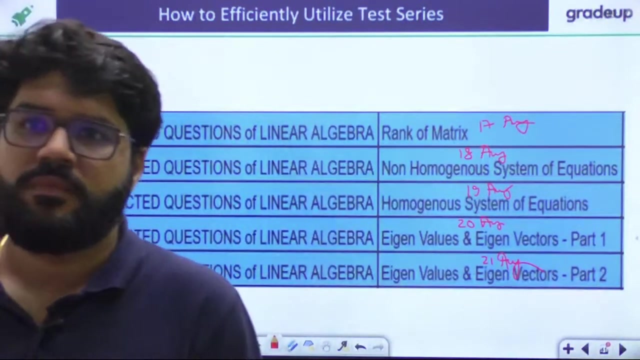 today, 17. yes, today we have done right. tomorrow, non-homogeneous, then homogeneous system of equation to linear system of equation, right, approximately daily, same one hour, then. this is what 20 august. this is what 21 august. this is what 21 august, right, right? 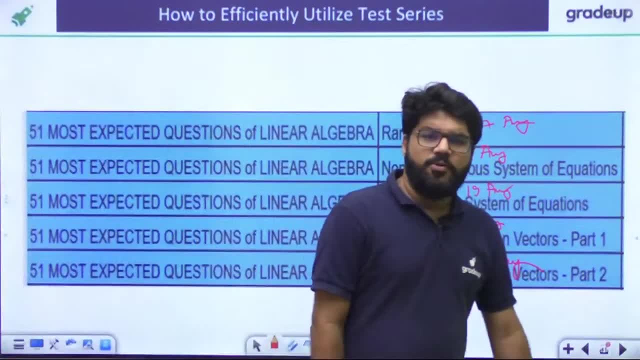 so go, pk, practice a little bit, make the states go float, okay, doubts float. now guys. now guys, let me write down la underscore: yeah, keep your simple. so guys, so guys, we have the time last worst, study the declaration of agreement and yes, tomorrow, which is given the order. 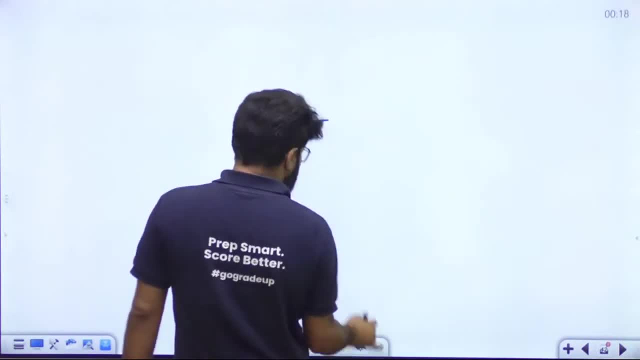 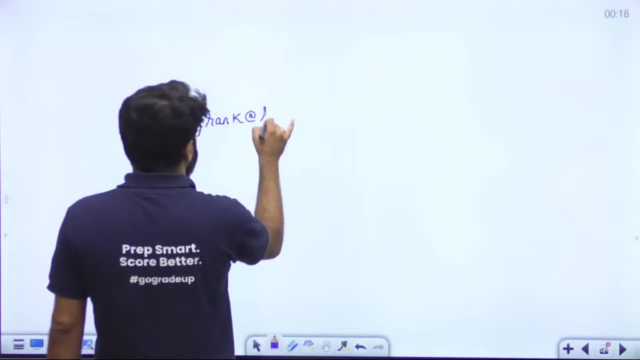 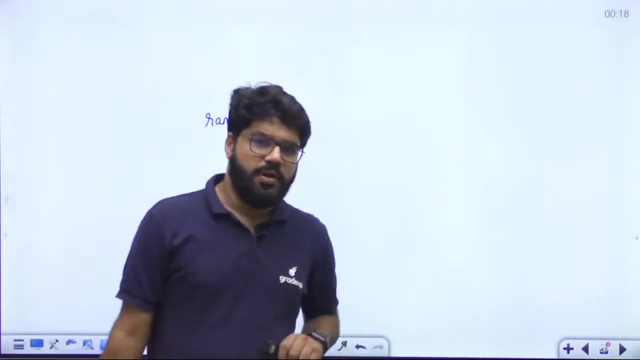 too. okay, so right, today, puffs if it do not happen. hey, mr teacher, you are screaming. I have posed some doubts. let me put down you many days problems. sir, there he is. see, this is it's all money tooitting. rank at the rate la, rank at the rate la. this is the simple, simple passcode. see, guys, i know. 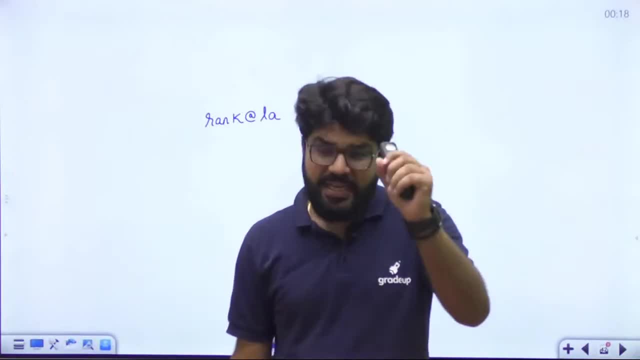 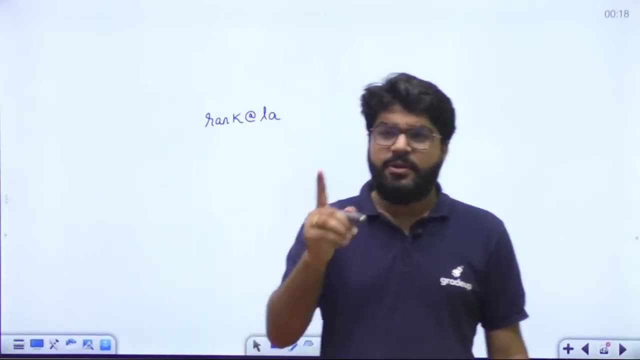 people like you, students like you, shedding your blood at night 12- 20, you are there, live right. differential equation will take you home. okay, next i can plan differential equation so night 12- 20, it is approximately 2020 and you people are live dedicated. so, whatever pdfs you, 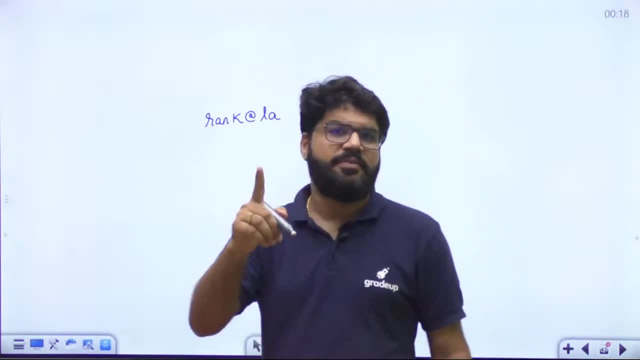 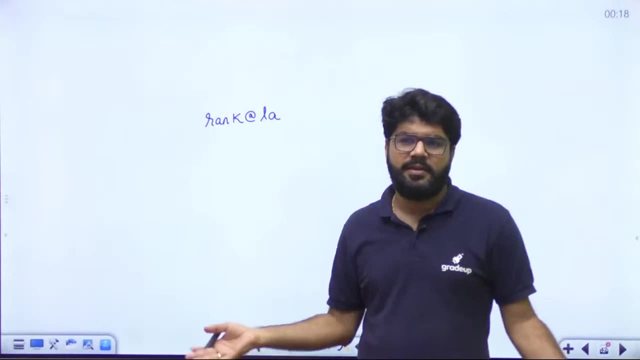 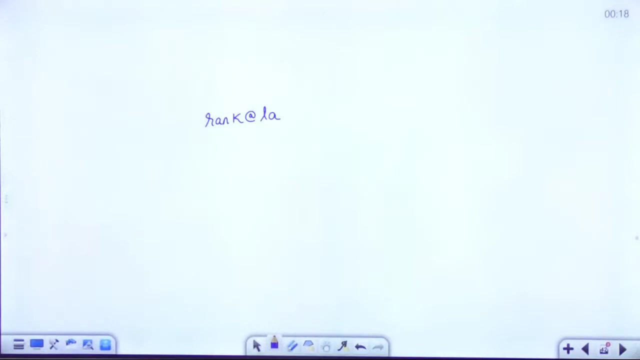 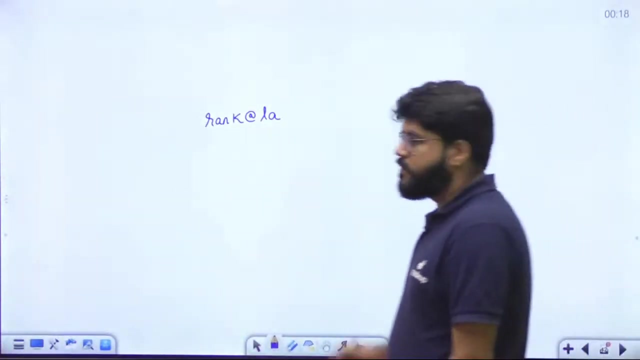 want will be there in the telegram, but it is password protected. always, my funda is there, password protected. i don't want to spread it out unnecessarily here and there, unnecessarily here and there. right rank at the rate, la rank at the rate, la rank at the rate, la right. so this is the password, this is the password of the pdf. okay, this is the 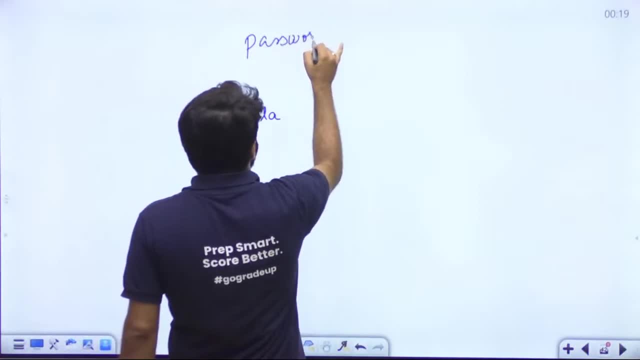 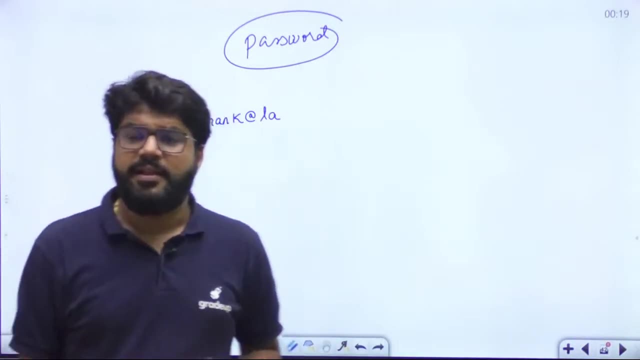 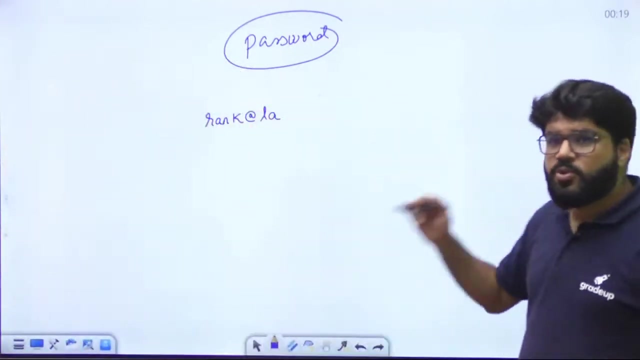 password of the pdf that will be shared in the telegram tonight. okay, rank at the rate, la rank at the rate or your random passwords. tomorrow will be something fresh, something different, random, random, random, random passwords. okay. so, those who are live- and i request guys, because you are live, you are getting the benefit, don't share the benefit. 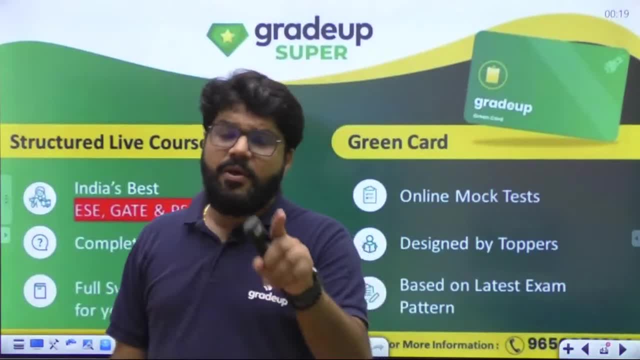 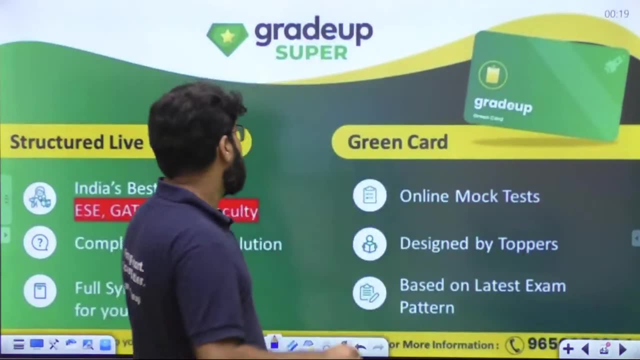 it is you who are live till 20 disappointed. okay, so it should be your right. don't spread across the password. keep it with you. that is what is my humble request with you, because this is your benefit. okay, so do get access to the great of structured life courses. you can go. 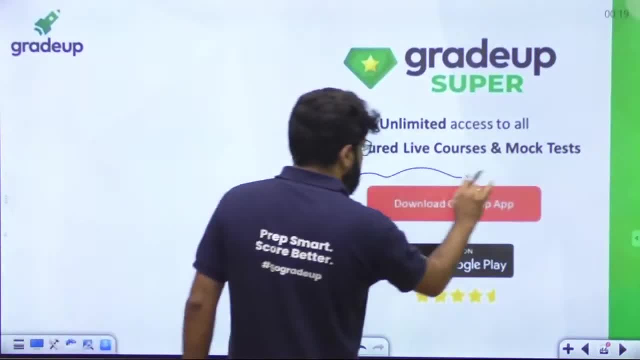 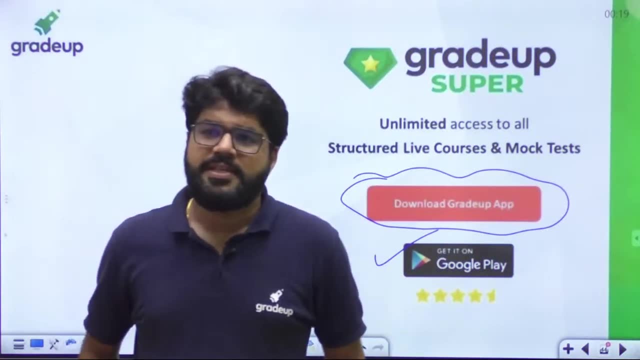 for the grade of super platform. okay, right, so you can just download the great up app available on the google play store. okay, yes, as we looking through the first story session tomorrow will be coming up tomorrow with non homogenous system of equation guys. tomorrow, same time. tomorrow tomorrow and then after幾issimo. 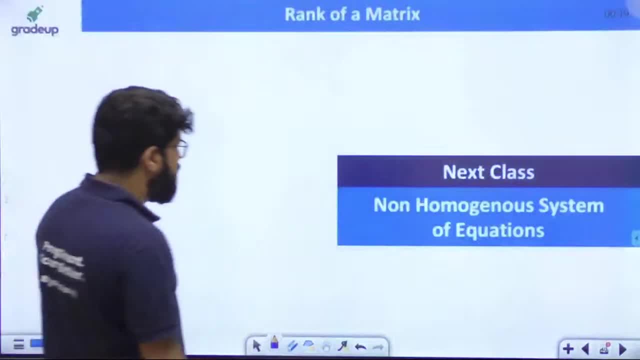 that the sum possible. so data is something will be delivered to mc where from the pdf, which is because the string is correct. how to use it right for all the sharing here in the uniform Tomorrow, same time. I have told you the password. I have told you this: 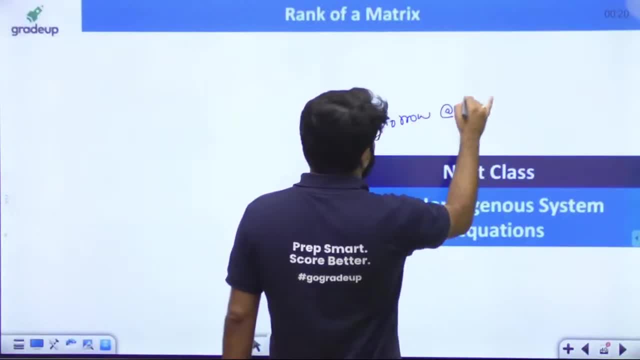 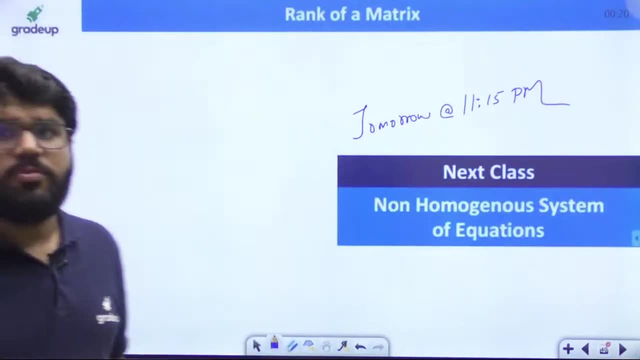 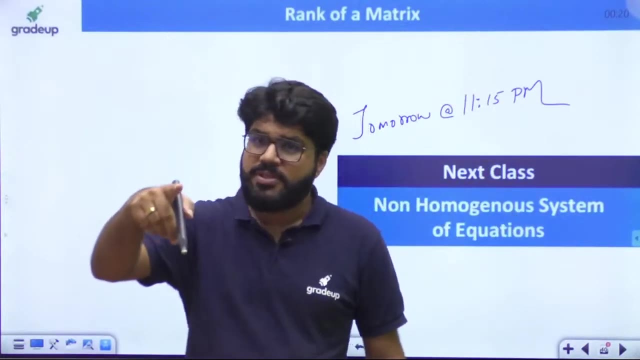 Tomorrow, same time, 11.15 pm. Okay, guys, Bye, bye. See you tomorrow, same time, 11.15 pm. With the same joy, Same attendance. If your attendance will be maintained, Then I will understand How much dedication is there.